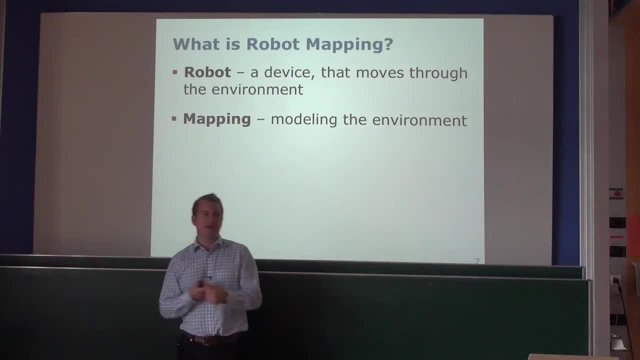 fly through the environment, swim whatever you can imagine. And the second thing that actually we look into here is devices with sensors. So some people call actually what? sensors on wheels, which is actually in some sense true. depending on the application that you do, It may be sufficient to just have sensors on wheels and some very 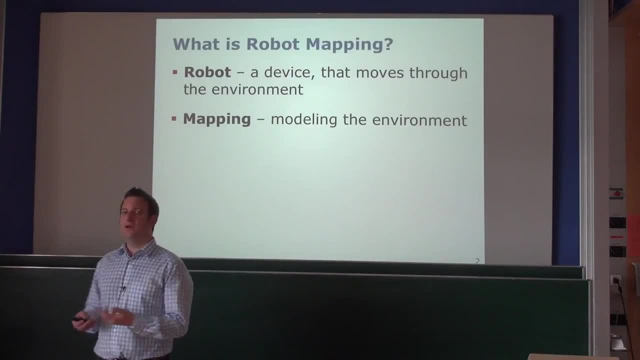 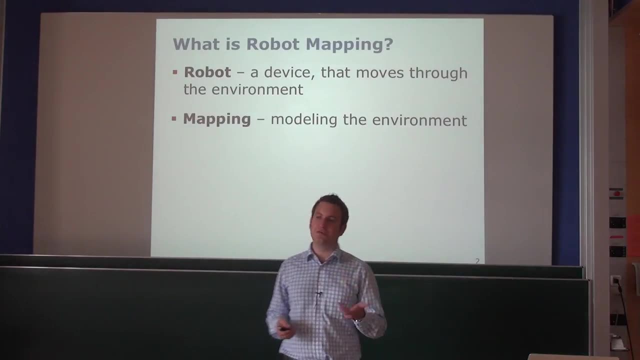 limited computation power. Depending on the application that you focus on, you may want to have a more powerful robot, But the most important things that we actually use here in this course are the perceptions and also the controls that are sent to the robot. So 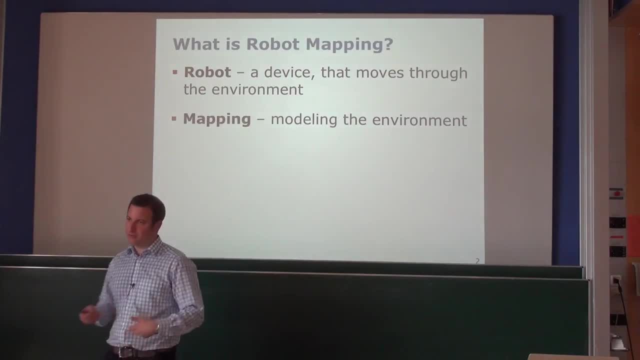 if the robot says drive a meter forward, and send this to the motors and the motors drive a meter forward, or approximately a meter forward. that's a valuable information And whenever the robot has a camera and takes a picture of some part of the environment. 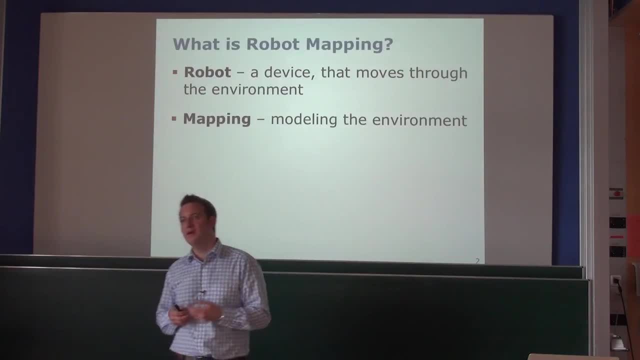 or it has a laser scanner installed and gets proximity measurements to the closest obstacle. that's kind of our sensor information, And we want to exploit the controls and the sensor information to gain knowledge. We want to gain knowledge about the environment. That's where we come to the second part of the title, which is mapping. We want to look. 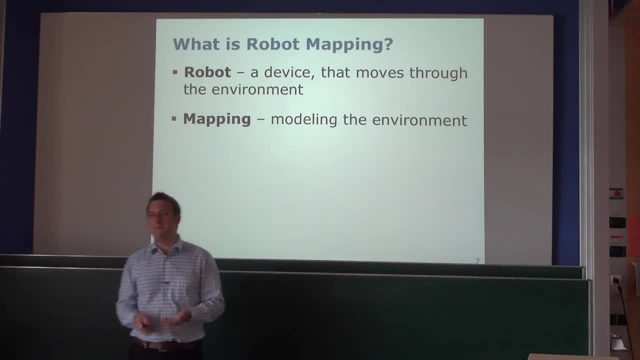 into robots that actually build a map of the environment. Map is a very flexible term that can be some representation. Openly look to a computer that actually creates a map, And also for mobile robotics. you really have to explore the environment a little bit If you're. 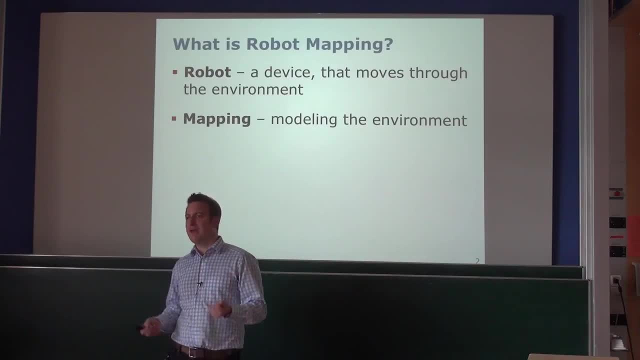 representation, some model of the environment. It doesn't need to be a metric map that you may know, or your city map or your subway map that you're used to. There are different kind of maps: geometric, topological maps. It's just some representation that the robot uses in order to model the environment, gain, collect knowledge about the environment. 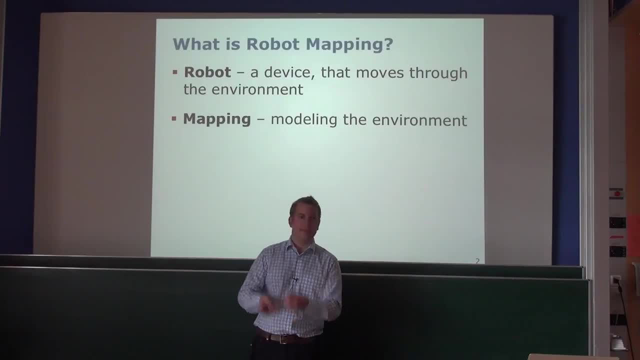 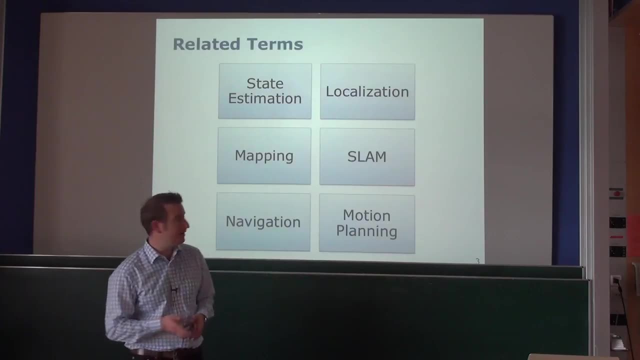 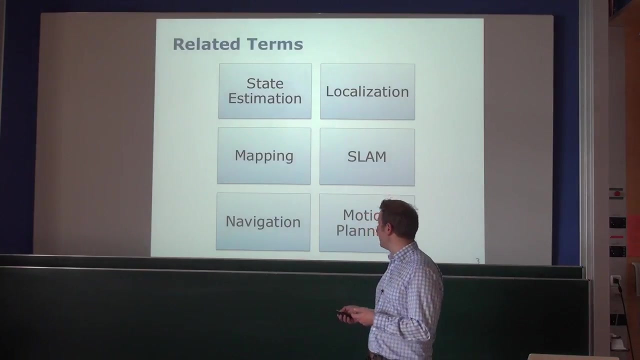 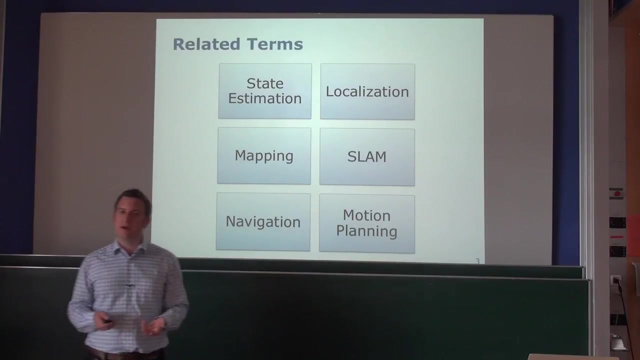 and, in the end, use this for decision making. Any question at that point? Okay, So these are terms which occur in the context of robot mapping. Some of them are closely related to robot mapping, Some are less related, but still influenced by that course. So we start with state estimation. State estimation means: 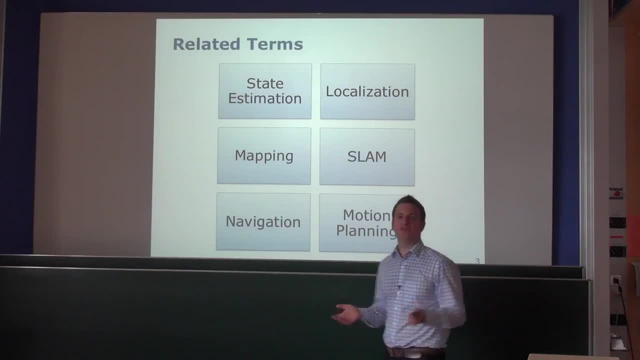 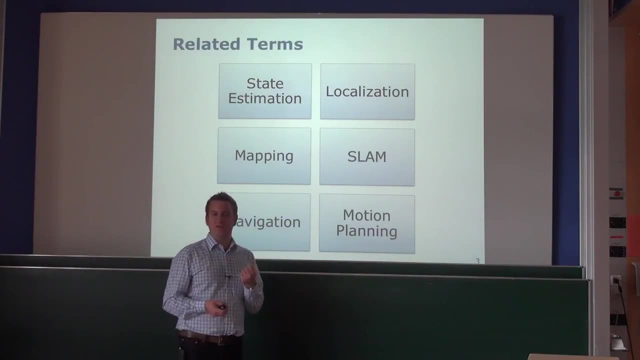 we have a state- Let's say the position of the robot in the environment were the position of a landmark in a given reference frame- and we want to estimate this quantity of the state, the state the world is in The world state. We want to estimate it because we don't know it perfectly. We just get sensor data. The sensor data is noisy. 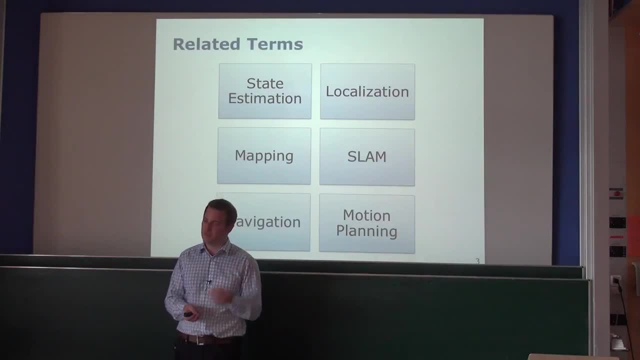 in most of the cases- actually always- The noise can be very small, but often the noise is not that small and we want to estimate that state. So, for example, we want to know where the robot is, or we want to know 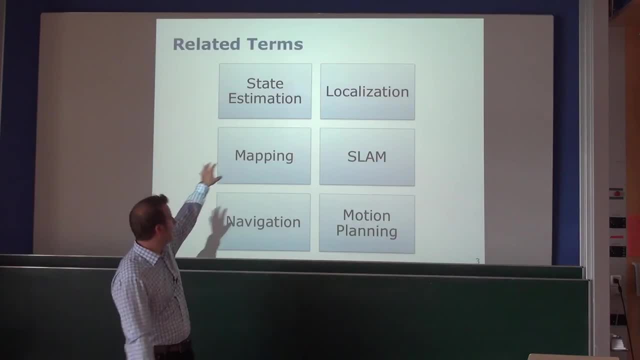 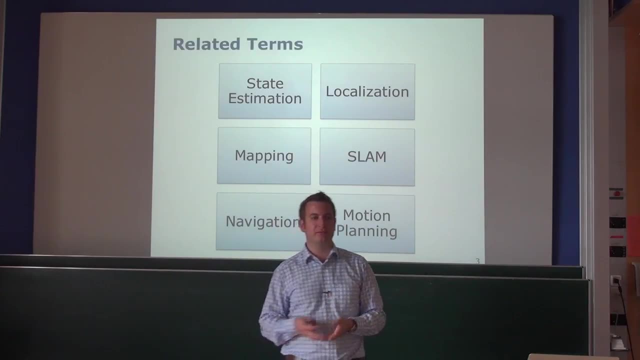 where landmark is in the environment. So this is what often set with state estimation, And one way to do state estimation is a base filter, recursive base filter that you may have seen. So if you have noisy observations, you have noisy controls. 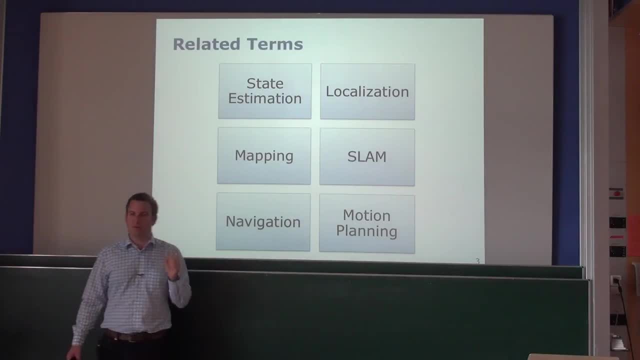 there are techniques. We will look into this recursive base filter in more detail next week. It's one way to do state estimation. So to estimate what's the state of the world, The world can be whatever you want to model about the world. So the position of the robot, the position of landmarks, 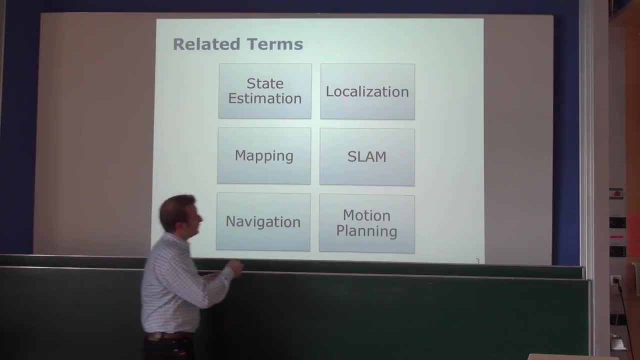 whatever it is you're interested in. This is closely related to the second problem over here: localization. Localization is actually a part or an application of state estimation. in most cases, It means we want to estimate where is our device, our sensor, our robot. So where is it in the world? 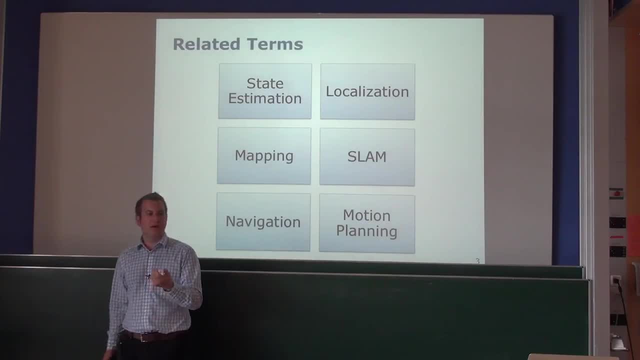 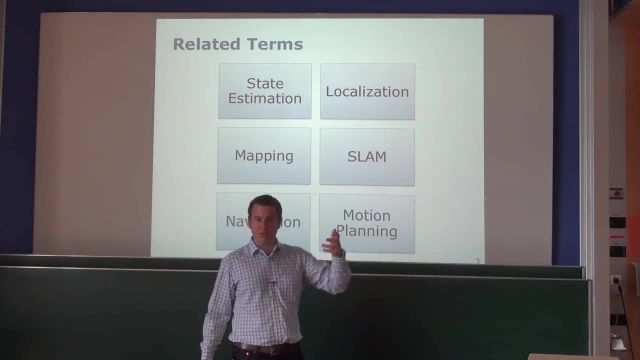 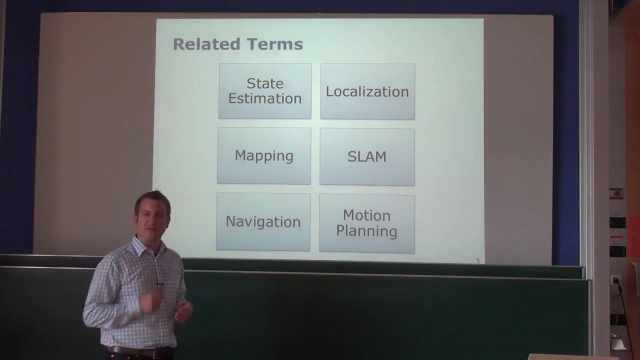 We want to estimate the location of the robot. We often talk about the term pose here, which is often referred to as the location, the XY coordinate, for example, as well as the orientation, the angular orientation. So where does the robot look? Which direction does it look? 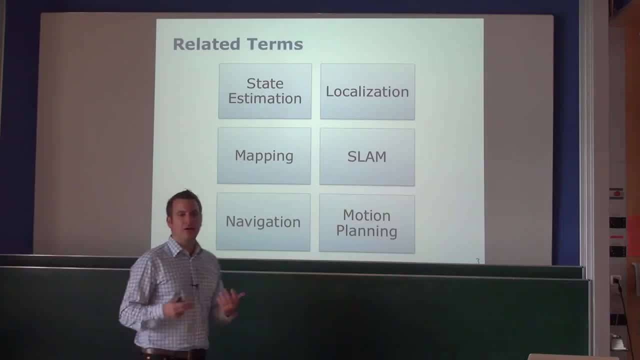 There's something which is often referred to as pose, whereas location often means just the XY coordinate. This is different in different fields, depending on whatever. In robotics it's kind of coined into a kind of a standard to do it like that. We have other fields, other fields which do mapping, which are related to what we're doing here. 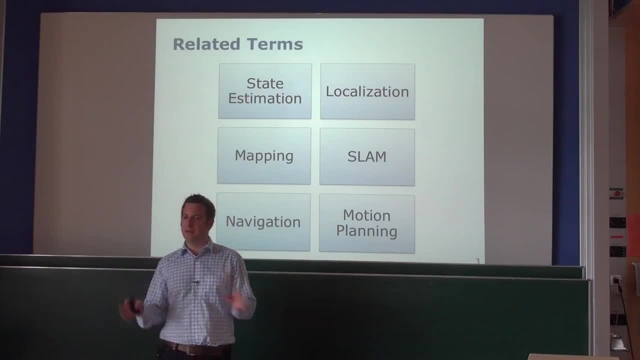 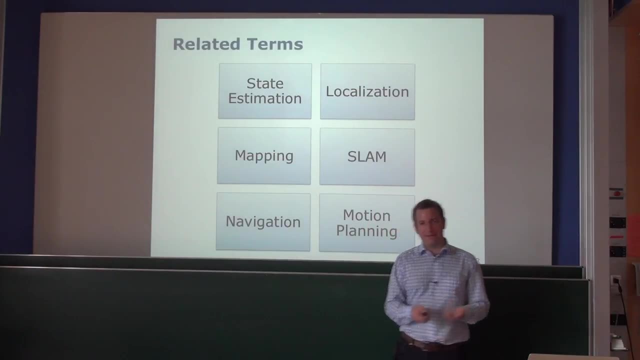 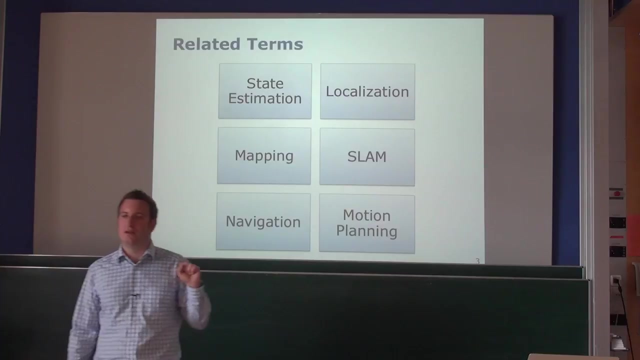 They may use a completely different terminology, But that's kind of that's a standard thing most people use in robotics. Okay, then we have mapping. Mapping in the robotic sense is often referred to as kind of having sensor data and I want to estimate the model, the model of the environment. So I want to map the environment. 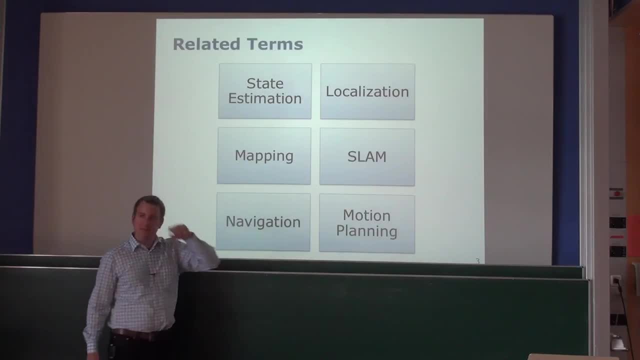 In a lot of aspects, this mapping means that you know where your sensor is. This is not the case in the general mapping framework, but in robotics. if we talk about mapping, we typically mean we know where the sensor is and we just want to estimate the quantities that we see. 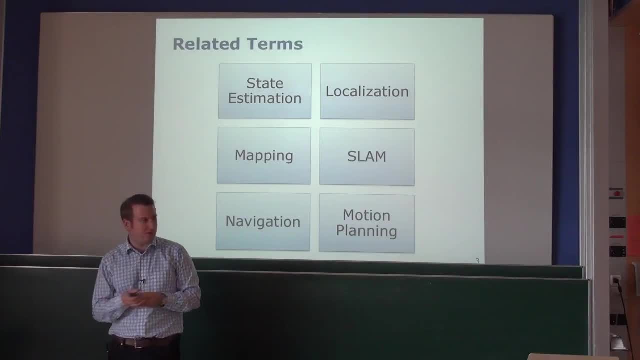 For example, we know the position of a sensor here and I want to, for example, with this laser measurement device. I want to measure what's, where is this wall with respect to the position of the of the laser pointer here? And then that's the measurement and I just want to estimate where is that wall. That's something which is mapping. 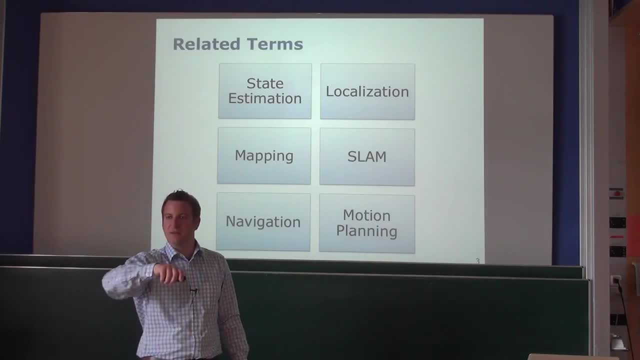 If I don't know where this sensor is. that's typically a combination, a combined problem which includes localization- telling where this device is- and mapping, telling where that wall is. So therefore, in robotics, often people use the term mapping, assuming to know the 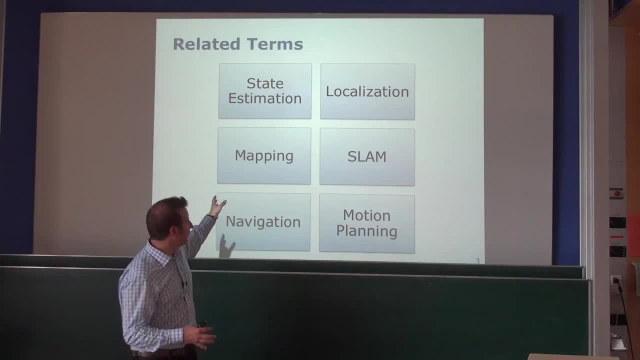 position where the robot or where the sensor was, And if you don't know that, then you actually end up in SLAM. SLAM stands for simultaneous localization and mapping. That means you want to simultaneously estimate the position of your sensor, of your robot, and the state of the environment. 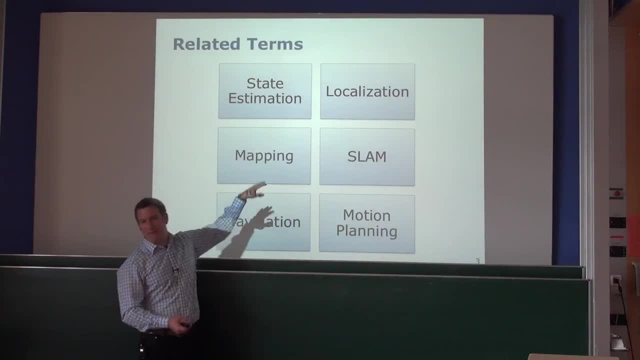 Therefore, people sometimes, or often, distinguish between mapping and SLAM, Although if you talk in sloppy terms, mapping would mean everything, because at the end, you're often interested in the map of the environment. Therefore, the course is also called robot mapping, or so it's a bit sloppy in the terminology that we often use in robotics. 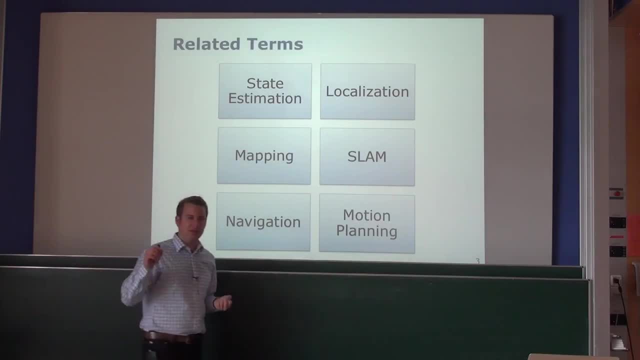 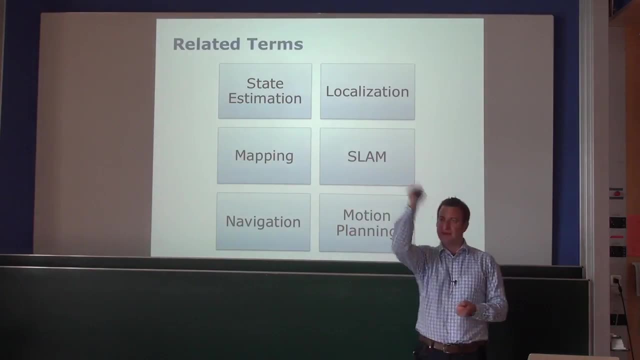 Okay, the next thing which is important is navigation. Navigation means I have a device or a robot which can make its own decision and maybe I tell that robot: hey, go whatever in that corner over there and the robot needs to decide. should I actually navigate here around here? 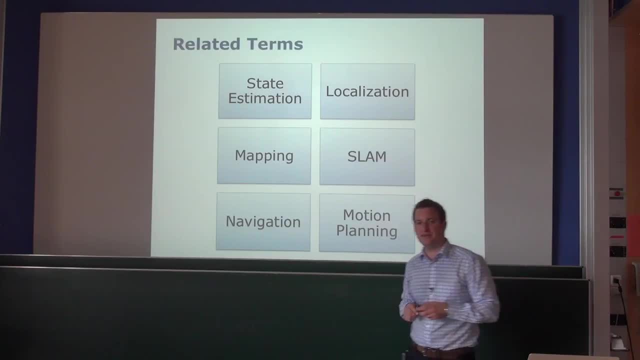 or should I take a left and then turn right over there to end up at the desired target location? Navigation is not a topic that we are going to address in this course here, but navigation strongly relies on SLAM or on mapping, on having a map. 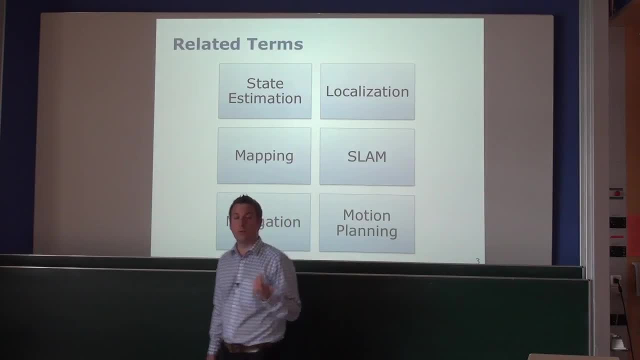 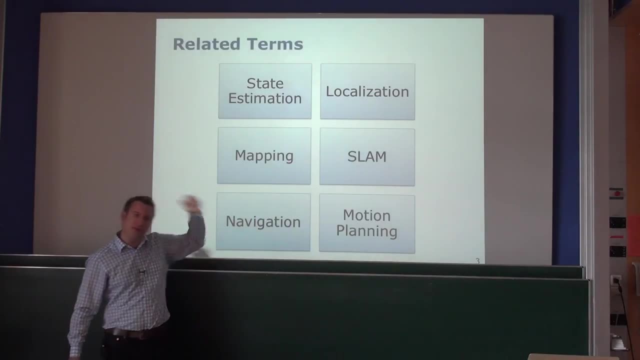 And also knowing is required to know where the vehicle is in order to plan a path and navigate somewhere. So navigation is not explicitly addressed in this course, but it's. one of the key motivation factors of that course is that we want to have models about the environment and 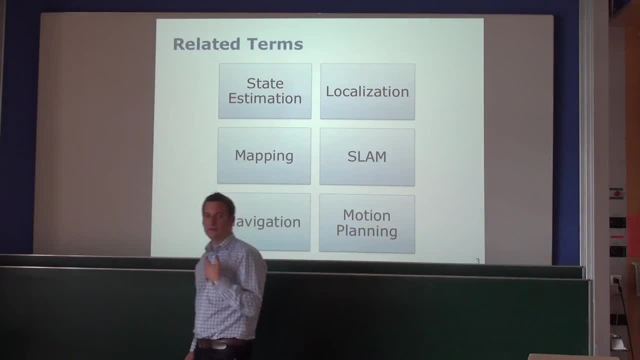 estimate the location of the robot in the environment in order to carry out navigation actions. We may do other things. we may manipulate objects with the manipulator and the robot may not move at all, but they also need to know what the environment looks like around that robot. 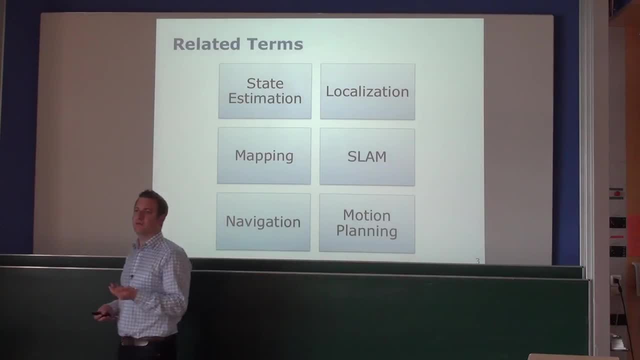 So, whatever decision you're making, it's often very helpful to have a model of the environment at hand. That's kind of one of the motivations for that course. here And then. motion planning is kind of very tightly coupled with navigation, so you really want to plan where to go which may satisfy some constraints. 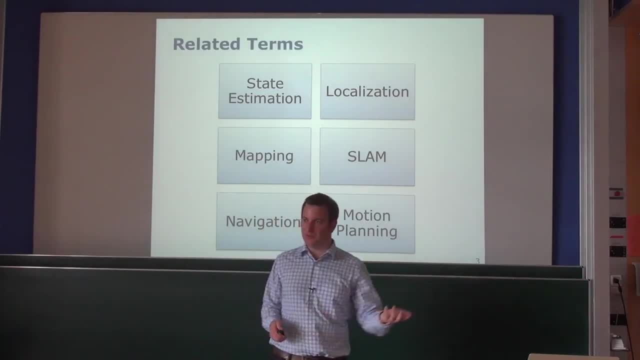 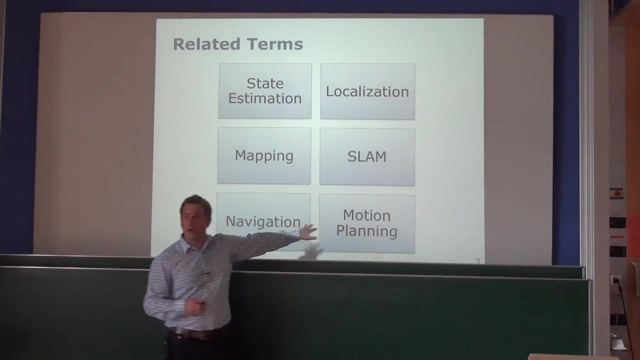 and you may seek to find the optimal motion sequence to reach your goal location. You may plan motions of, as I said, manipulators before, so it may go even beyond whatever. just moving a rigid body in the XY space Can be more complex, but again that's nothing we are going to address in this course. but these are techniques which actually 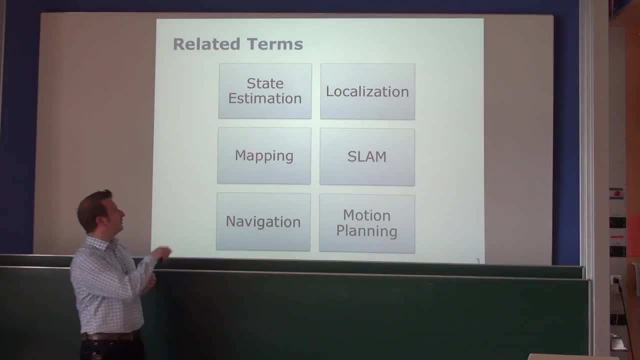 benefit from having an environment model. So we will actually look into these four aspects here, where SLAM is the most important stuff that we cover. but if you solve SLAM, you also solve localization, you also solve mapping, and in order to solve the SLAM problem, you need to say destination. It's kind of the rough picture that we are going to address here. 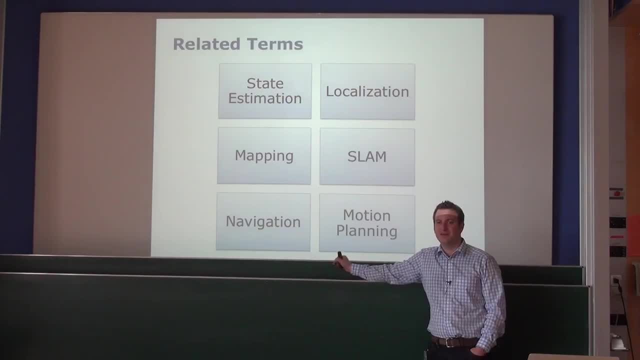 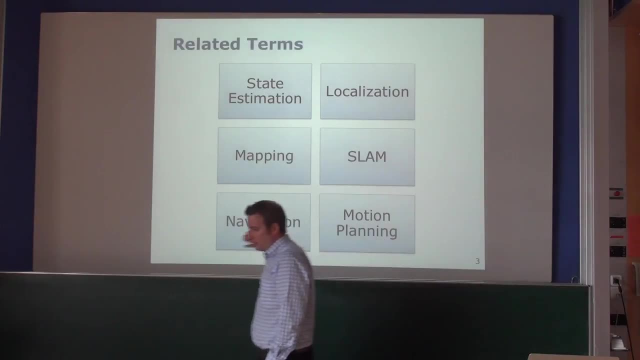 Any questions so far? Yes, please, I actually have a question about navigation and motion planning. Yeah, I think it's actually the difference between them. Yeah, so, as I said, in motion planning, you can actually plan the, the trajectory or a sequence of states that a system should be in in order to reach a certain goal: configuration. 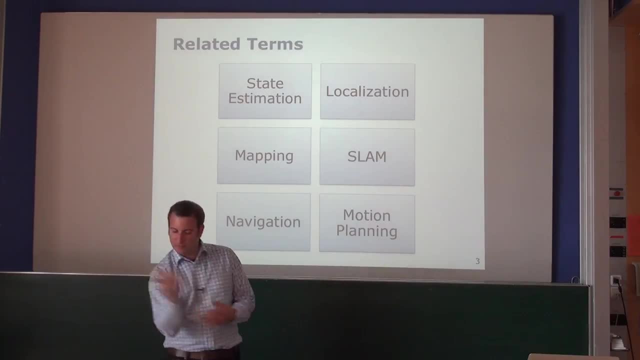 So it can be a manipulator. So let's say my arm is here and the arm should be. how should I get my arm in this hole over here? That's a typical motion planning problem. You wouldn't typically call that navigation. Navigation is typically a device which moves in the x- y theta, x y orientation. 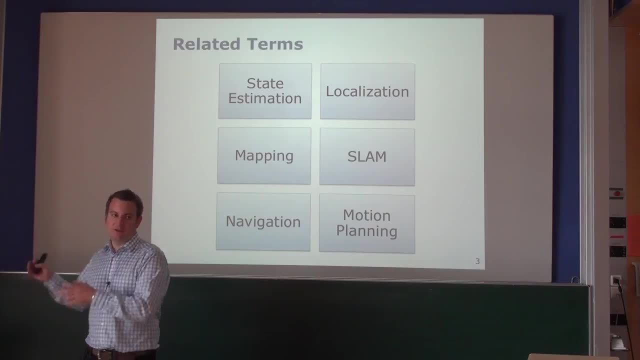 or in the three-dimensional space of physically guiding a robot from one location to another location, But they are very tightly coupled. So most navigation systems use motion planning algorithms, like whatever A-star or variants of A-star that you may have used. that you can use for guiding a vehicle from location A to location B, but it's not restricted to that. 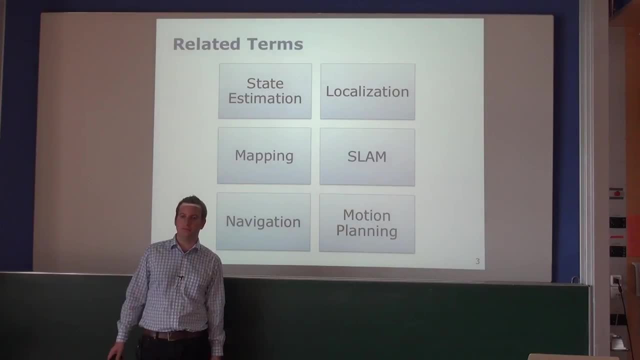 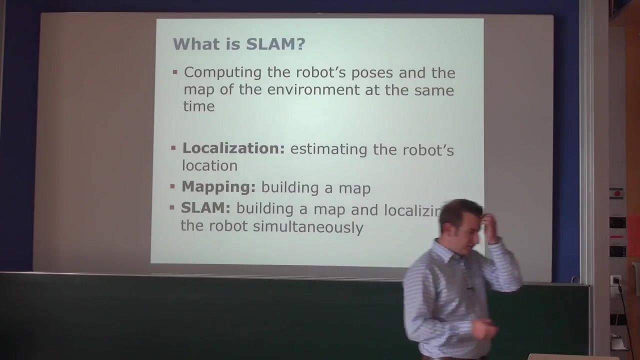 You can also use planning for other kinds of problems that you're going to solve. So it's kind of what I told you before was kind of more the core robotics perspective of that, But generally you're absolutely right. Any other questions? Okay, so let's go a little bit more into the details of what is SLAM and kind of be a bit more. 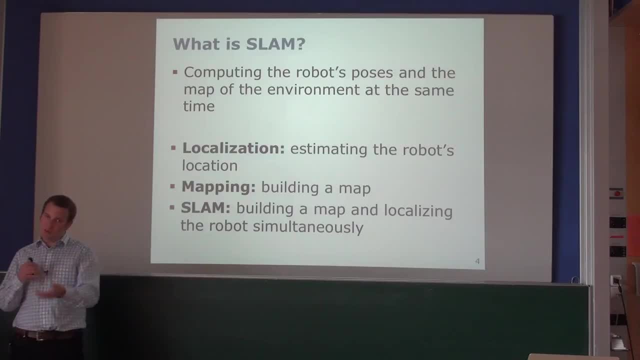 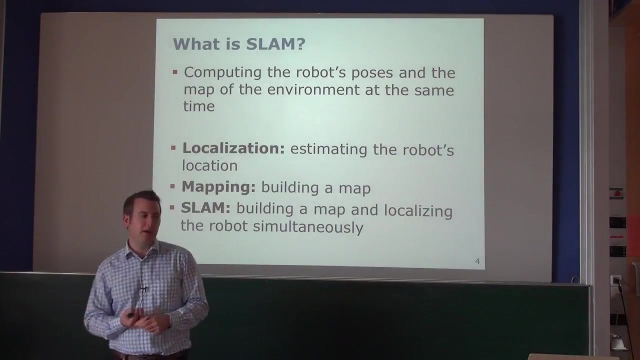 not yet formal, but formalize it a bit more so we end up in a more formal description in the end. So what we're interested in is actually computing the different positions of the robot at different points in time. It's kind of a trajectory or a path that the robot took, as well as a map of the environment. 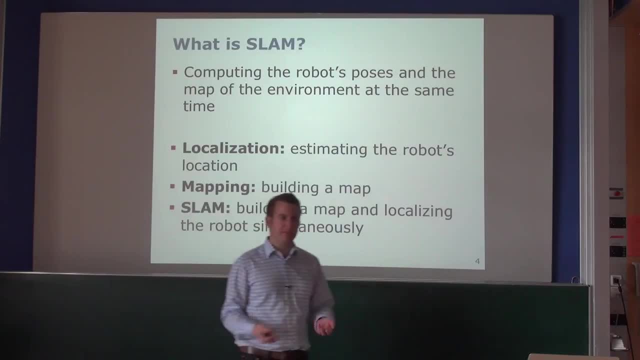 a model of the environment. There are different types of environment models that you can imagine. We'll discuss them on a higher level, at least during this course today, But that's kind of our main objective. And then we have the problem I said before: localization, which means estimating the robot's location. 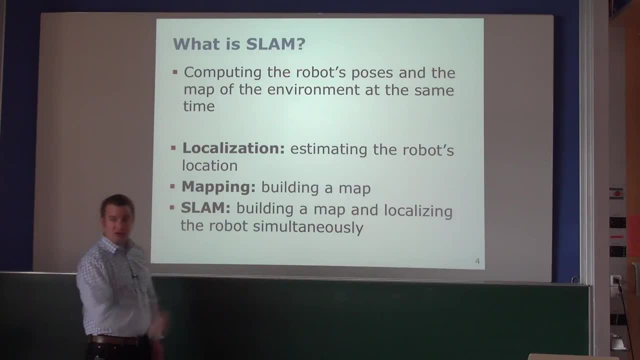 So this actually means estimating the trajectory- So where has the robot been at different points in time? And then we have mapping, which is actually trying to build a map. So, yeah, we have an environment model And SLAM. simultaneous localization means doing this at the same time. 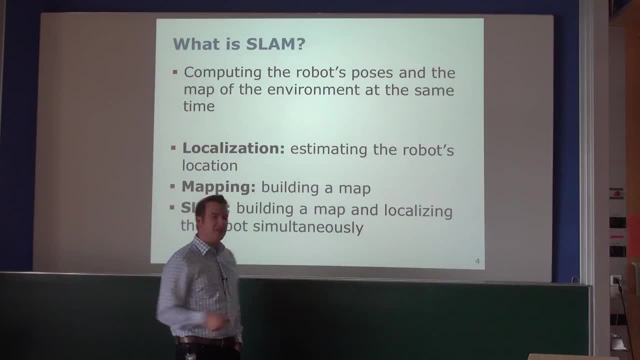 And in reality, these localization, the mapping problem. I don't want to say they don't exist, but in the end you always need to solve the SLAM problem, Unless you have some external, absolutely great whatever tool sensor. If God told you where the robot was at different points in time, yes, you can do mapping. 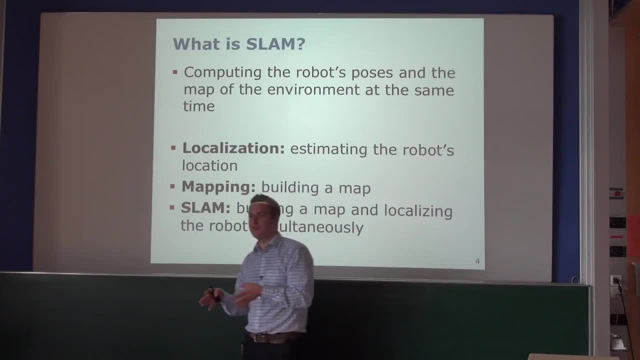 And if the robot told you exactly what the environment looks like? yes, You can do localization, But quite often these are things which strongly interact with each other, So if you don't have a model given by someone which you assume to be right, 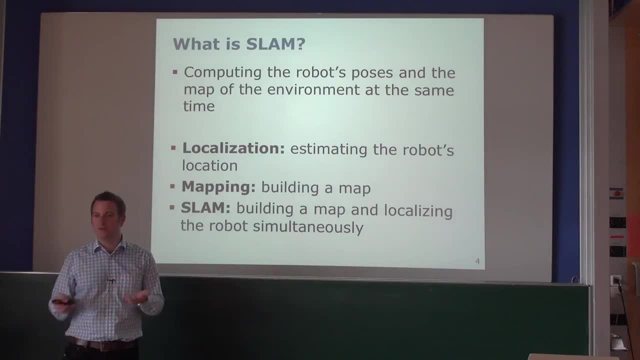 you typically need to do some form of SLAM to solve both problems at the same time. It may be that the environment model that you have is sufficiently good or sufficiently accurate. you can say, okay, I ignore the rest and just do localization. 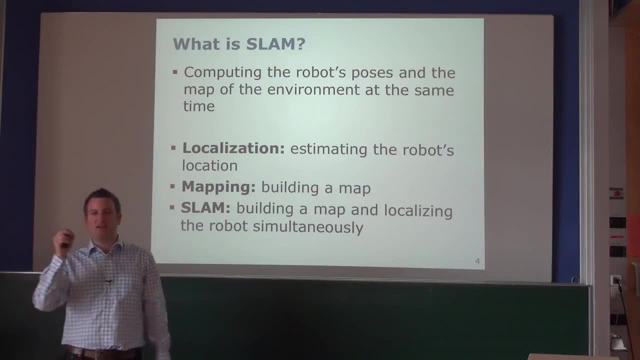 This case exists, Or if you say that's such an accurate whatever X, my robot moves on. I don't know a rail and I perfectly know it is on the rail with some other- means that I can focus on the more challenging task of just modeling what the environment looks like. 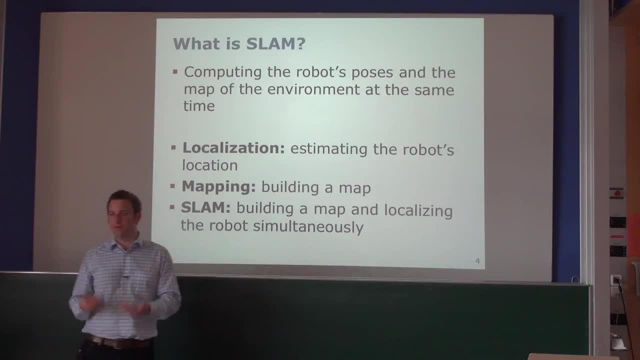 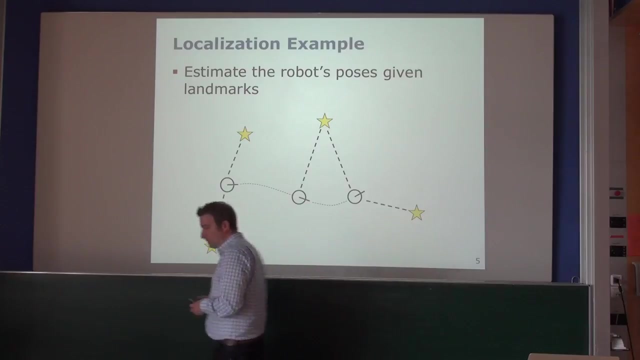 In this case you can also separate that a little bit, But in reality you're mostly faced with simultaneous localization and mapping, even if you're only interested in what the environment looks like or where the robot actually is. Okay, So just to make the point why, to illustrate the different properties of these problems, 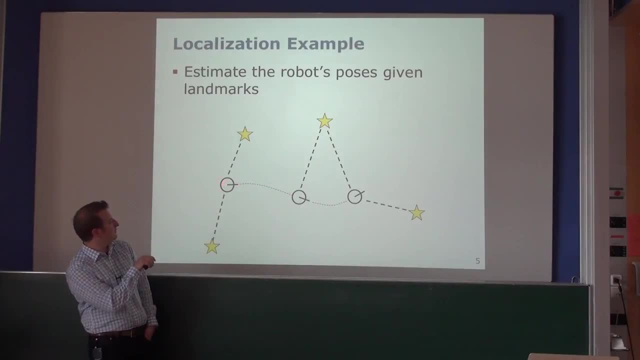 So what you see here is a robot at different point in time. So t equals 1, t equals 2, t equals 3.. The robot moves through the environment on some trajectory- We typically don't consider this as a continuous process, but at discrete points in time. 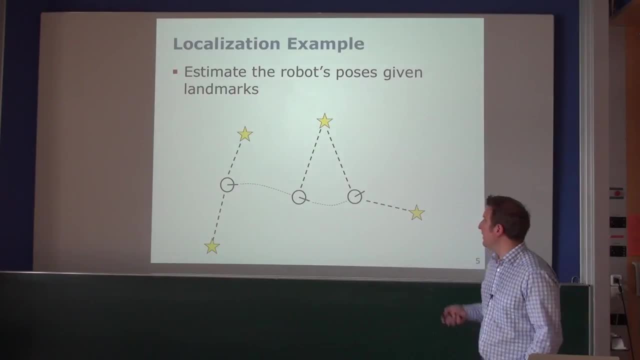 Say, every second or every time the robot takes a sensor measurement, And then we have other things here which are these stars, And these stars should illustrate landmarks. That means something the robot can observe and can recognize. So if you have a robot which drives around here in front of our university on the green, 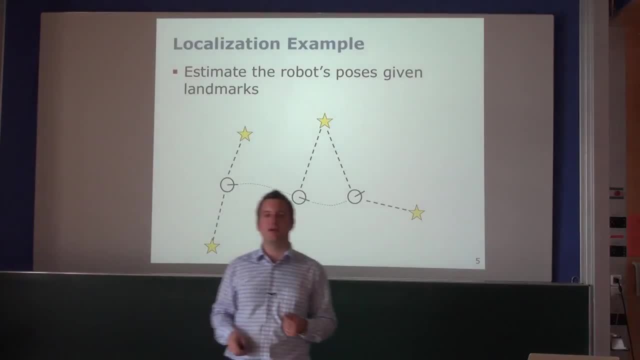 you will. it may have a sensor to detect trees, So every tree will have a sensor, Every tree will be a landmark. So then you have whatever Twenty trees here in front of our building, Then you have twenty landmarks And the robot may estimate the location of those trees, of those landmarks. 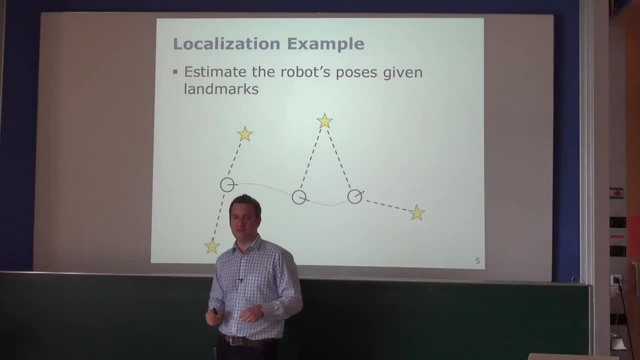 And then it can also estimate its own poles relative to these landmarks. Okay, So these guys are landmarks And these dashed lines here should illustrate observations of those landmarks. So if the robot is here, it can see these two landmarks. If the robot is here, it can see only this landmark. 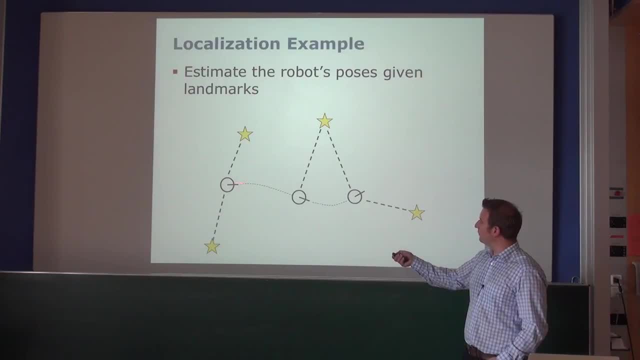 If the robot is here, it can see these two landmarks, And these small dotted lines are landmarks, And these dotted lines should actually represent the trajectory that the robot was taking. And I'm just considering these three points in time. Okay, Now we look at the localization. 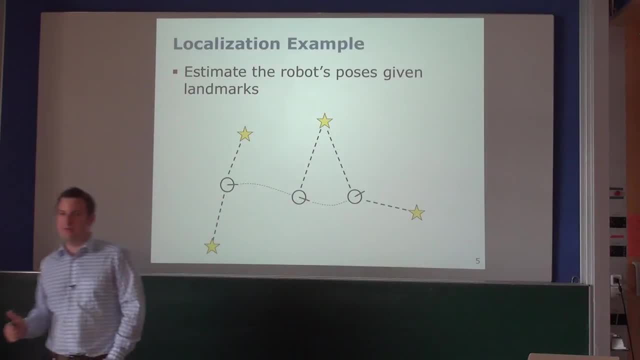 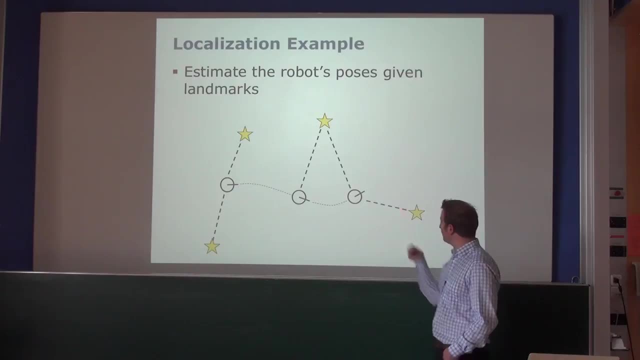 Localization was. we know what the environment looks like, but we don't know where the robot is. That means we know the position of those landmarks. So God told us the position of those landmarks, So we know those stars are here, And then we need to estimate: where was the robot? 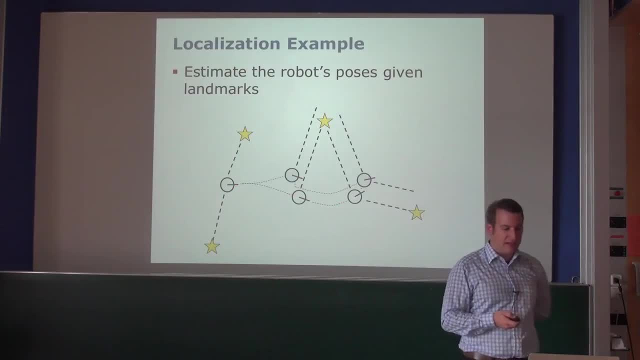 So we need to estimate those poses And this may look like this. So in the beginning the robot actually observed that here quite well. Then the robot was driving and it can actually deviate it from its path, So this is kind of the true path. 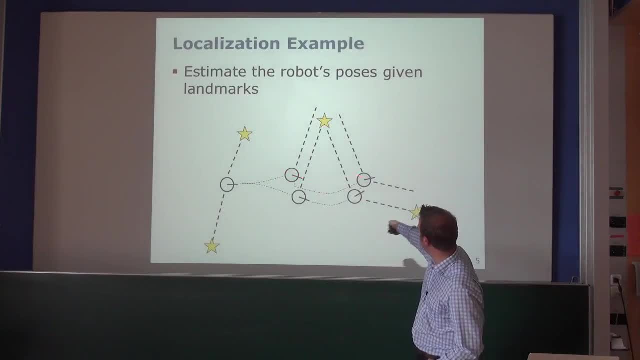 And this is what the robot estimates. So it's kind of the grayish dashed ones. are here the estimates of these two things. So here the robot thought it turned left But in reality it turned right, So maybe the air or one of its wheels lost air. 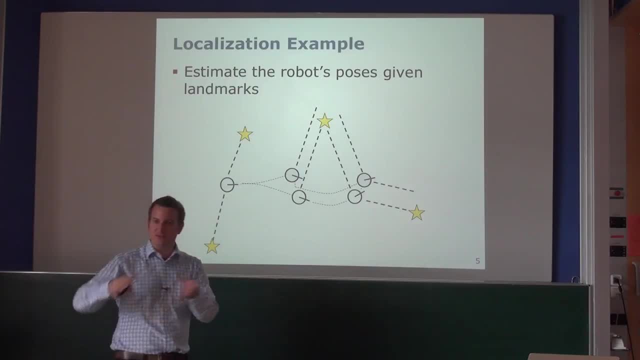 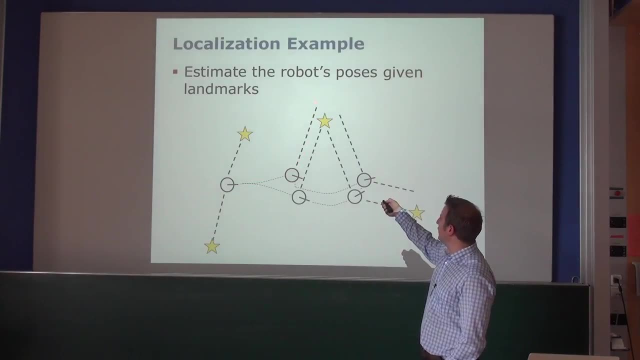 So the diameter of one wheel gets smaller And the robot gets a drift to one side. Maybe one explanation For these stupid behavior here. turning to the left, Then the robot makes an observation. It's okay, Here. the landmark should actually be here. 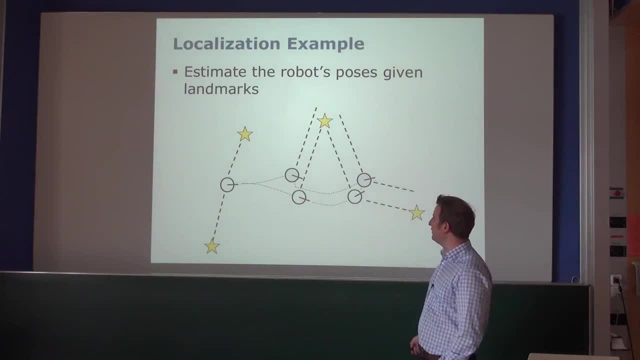 You say, hmm, But there is no landmark. So the landmark is actually here, So there's kind of a correction step that actually drags the robot towards its real pose. The robot was here, The landmark is one meter away. That's what I measure. 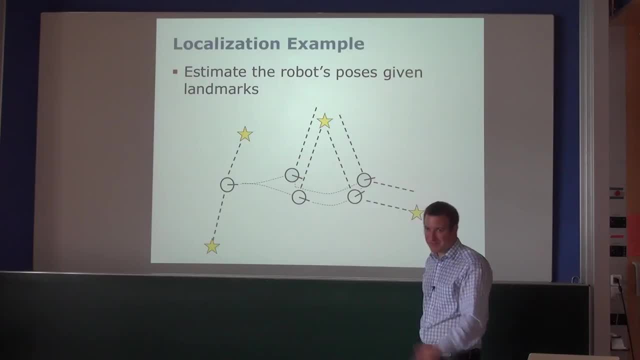 But according to the map it should be only 50 centimeters away. It's okay. There's a mismatch between what I measured. This is kind of what comes from this correction zone here, And then the robot continues driving And then another correction may end up here at the current pose at the end. 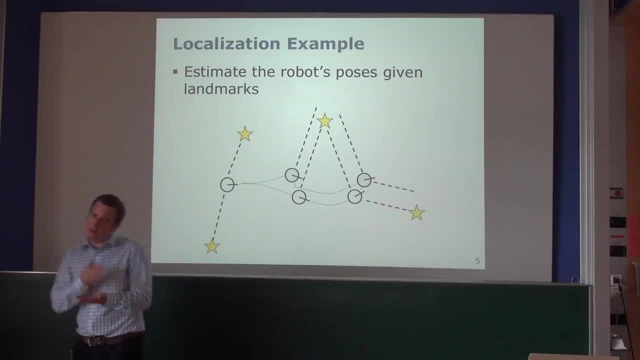 So that's kind of the localization problem. The robot drives to the environment. You integrate its control commands, You get an estimate of where the robot probably is. Then you get an observation. The robot sees some landmarks in the environment And then can kind of correct its pose. 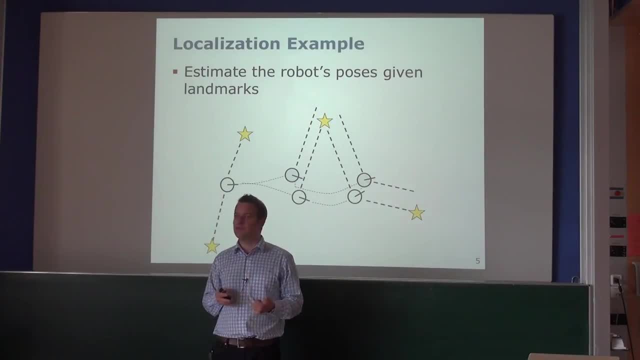 And the correction, or the amount of correction, depends on how accurate is its sensor, How accurate is its motion execution. If you have a very, very accurate motion execution but a very, very stupid or bad, noisy sensor, you will probably trust your motion estimate much more than your sensing data. 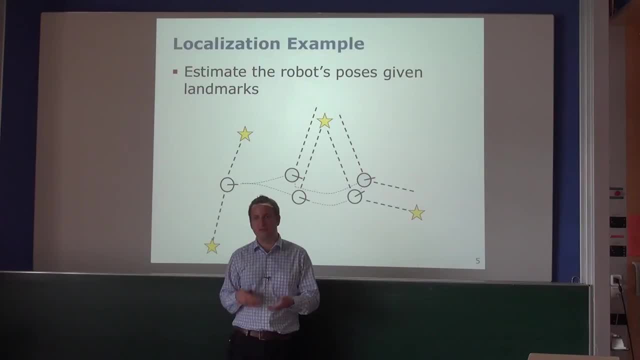 On the other hand, if you have a very poor sensor, for example, lacked robots like humanoids, it's pretty hard to get a good odometry, a pose estimate from the way these robots walk. You will probably rely much more on your sensor data. 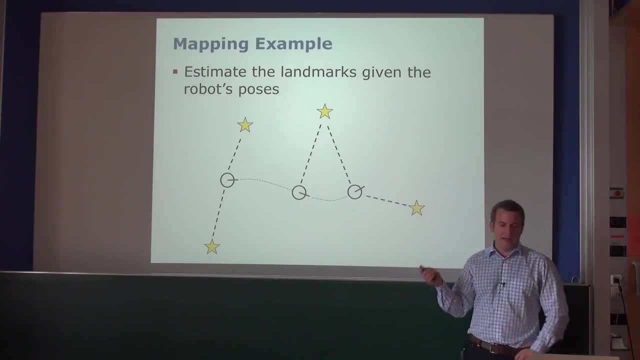 Okay, That's that. Then we can actually look into mapping. So this is what the world looks like in reality And the robot knows its pose, So it's kind of a mapping example now. So someone tells the robot where it is at different points in time. 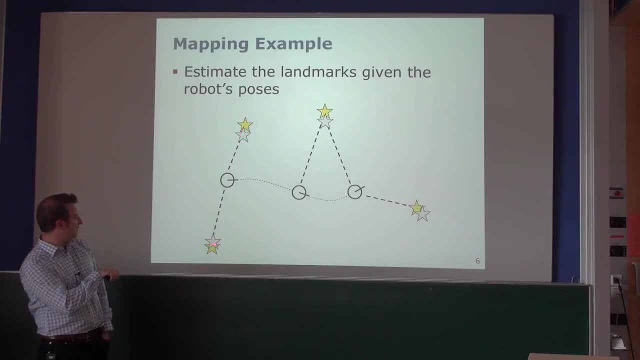 The robot takes observations And these observations may be here, that grayish stars. So the robot will move through the environment, So it will create a map where it will say, Hey, this feature is here. This feature is here, It continues driving. 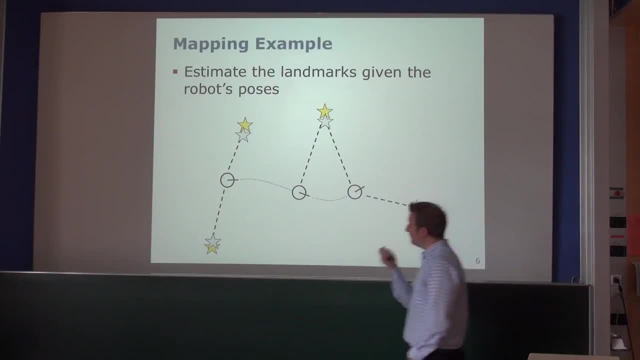 A feature is here And this feature is here. As you may observe, here again, this estimate about the world state is not perfect. The position of those landmarks are not exactly where those landmarks are, But this is just a result from your noisy sensor data. 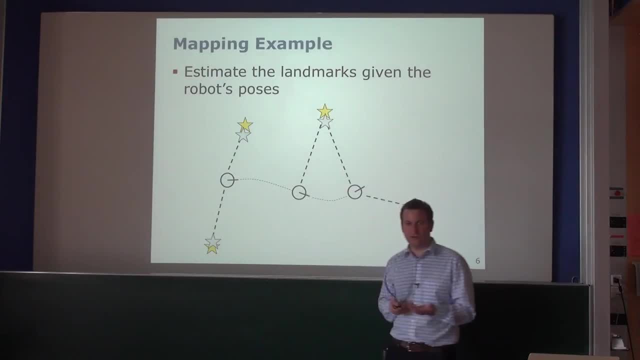 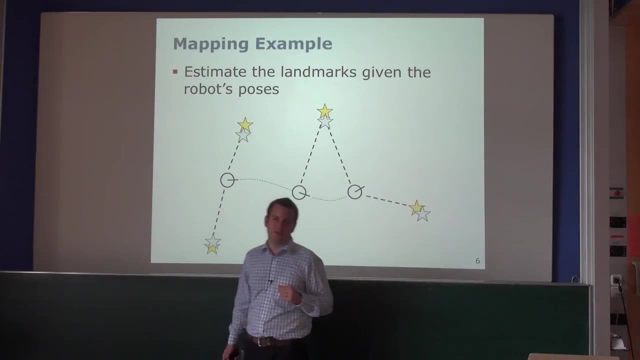 And in the ideal case, you know what the uncertainty of your sensor is. So you know. let's say, in 95% of the cases I have an error of up to 10 centimeters from my measured distance. In this case, 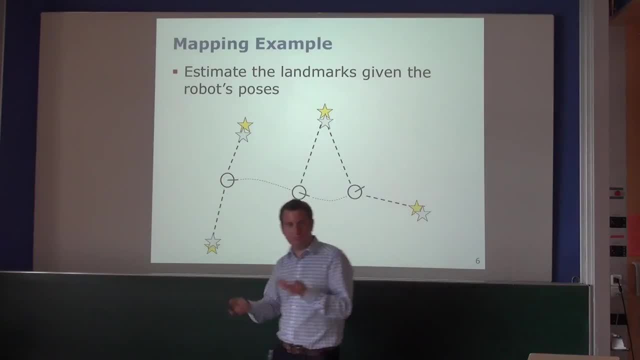 you could actually draw some uncertainty ellipses, like you would do if it would be a Gaussian estimate. You actually draw around your estimates and say: the true location of the landmark is very likely to be whatever within a certain bound. That's what mapping is about. 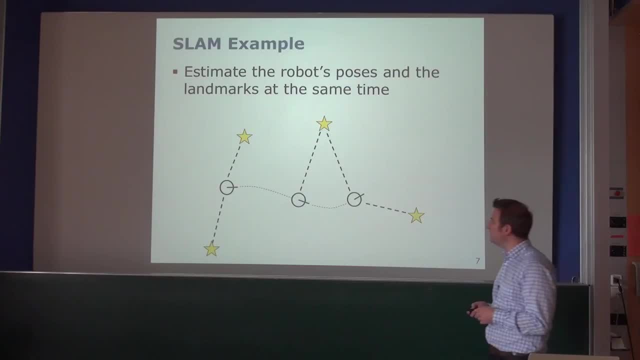 Okay, in SLAM again, that's a setup. what happened in reality? The robot started here, measured the location of those landmarks. These are these two guys. Then it continues driving Again. has this turn to the left? can drift to the left? 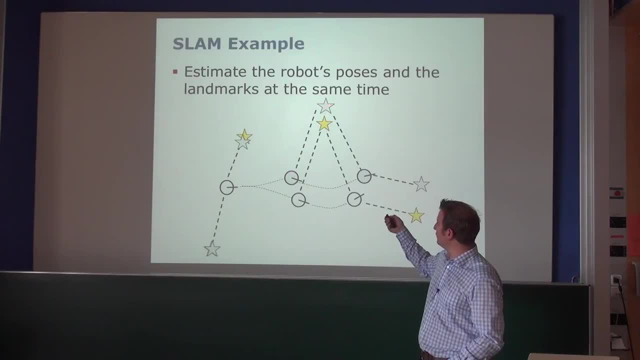 Then it measures the other landmark. So this is now this over here, And since it doesn't know where this landmark is in reality, it just adds this landmark to its map, to its self-built map, And it cannot do this correction step, or only maybe to some degree. 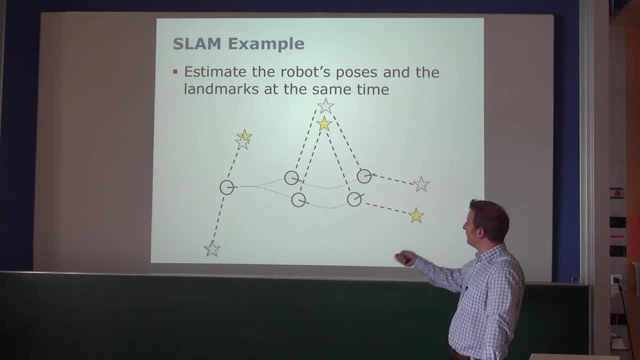 that the robot did in the localization example. Then it continues driving, So here the estimated trajectory of the robot will be this one, although in reality the robot took this movement, and the grayish stars is what the estimated map would look like. 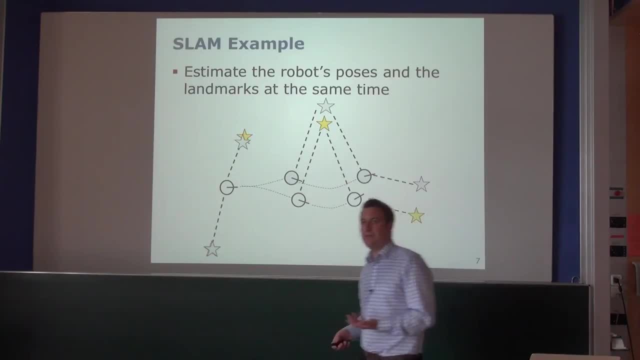 And this is substantially different from what the real map looks like. So there's always an error in our estimates- All realistic situations. there's an error in the estimate. What you may have seen here or guessed here is that actually the map estimate depends on the localization accuracy. 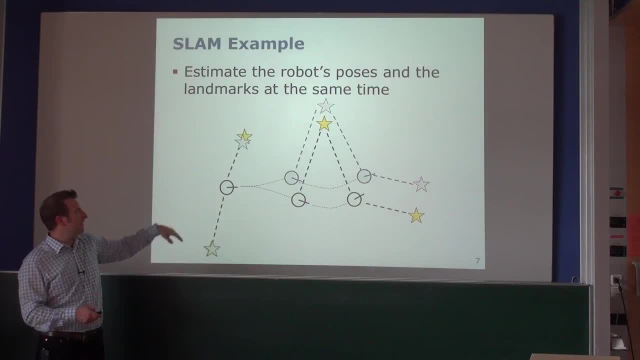 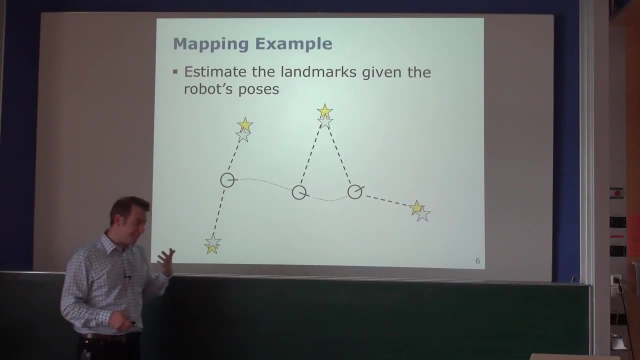 So this map is less accurate than this map over here where I knew the pose of the robot And if I know where the And so this pose estimate where I have this correction here, so this guy is dragged down here- is more accurate than the pose estimate. 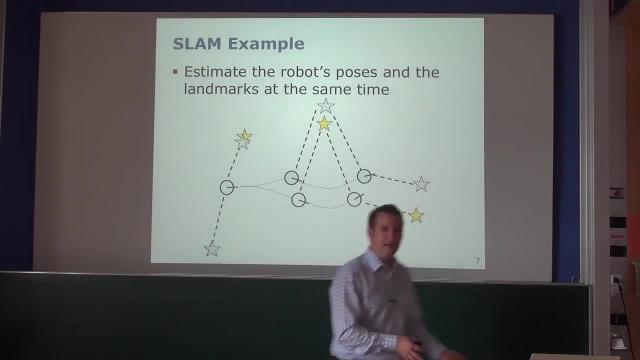 in the slime context. So whenever I know what the environment looks like, I can better estimate my pose. And if I have a good estimate about my pose, I can actually build a better map. That's also why this is often referred to as a chicken-rag problem. 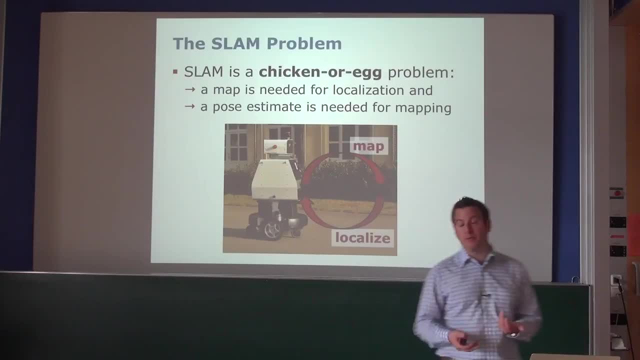 So a map is needed for localizing the robot and a good pose estimate is also needed in order to solve the mapping problem. So there's a dependency between what the environment looks like, or the model of the environment, and how well the robot can localize itself. 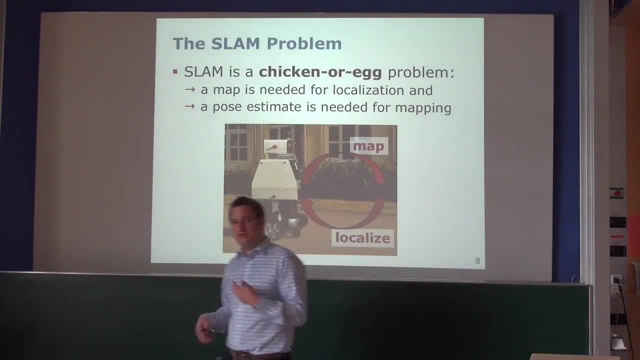 which again influences on how accurate my model there is. So this suggests that this is kind of a joint estimation task. We cannot fully decouple localization from mapping. We actually have to solve this at the same point in time. That's the reason why it's our main motivation. 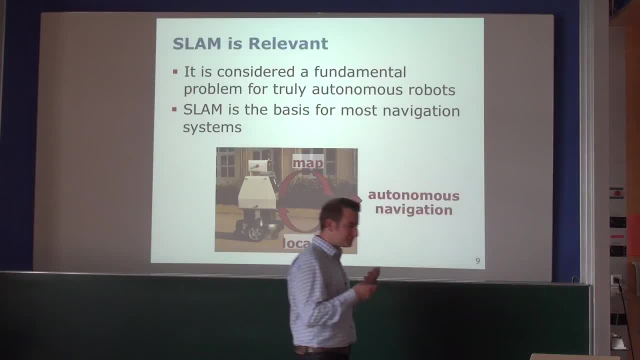 for the slime problem, And if we do that, then we can actually, So we can solve the slime problem. We have the most important, let's say, tools at hand or means at hand in order to solve the autonomous navigation problem, Having a robot. 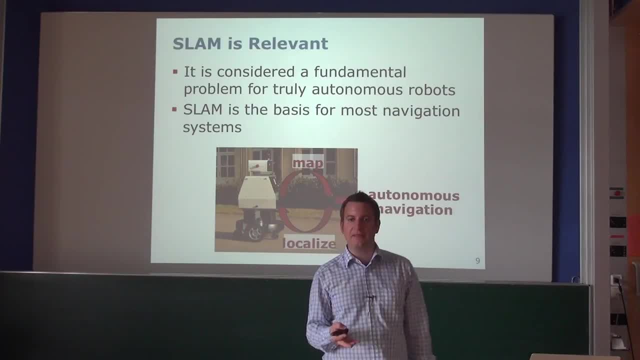 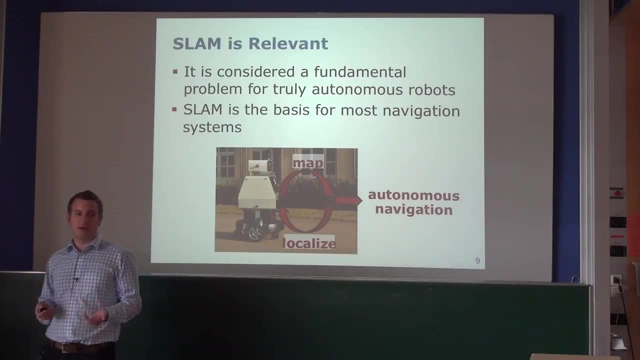 which I can just specify its goal location, and the robot is able to navigate there. In order to do that, it needs to know what the environment looks like and it needs to know where it is in the environment in order to reach its goal location. 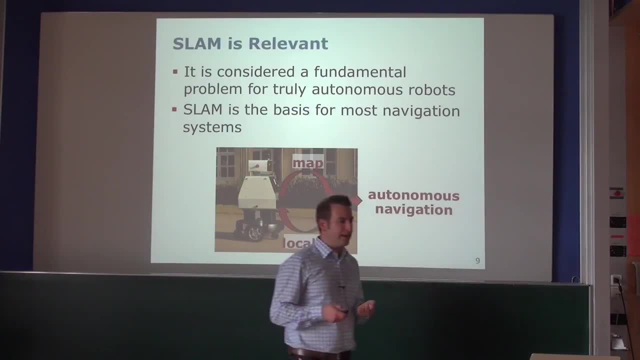 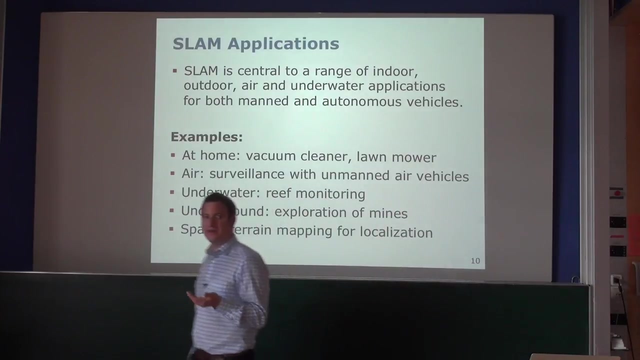 And so solving the slime problem has a direct impact on the applications that we can actually build with mobile robots- And there are typical applications or it's kind of Having a working slime system at hand is still something that a lot of robots actually miss. 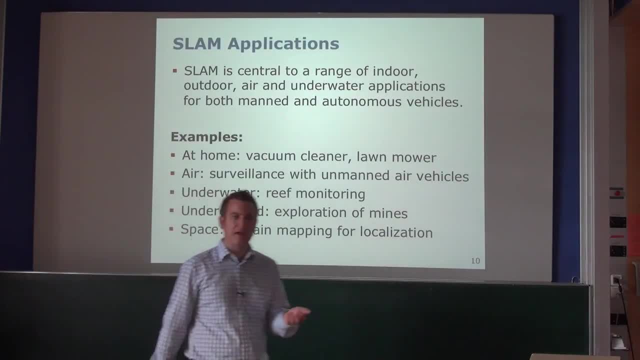 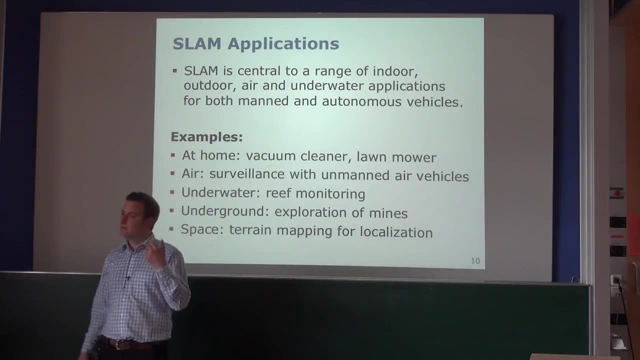 And it's one of the limiting factors today to, let's say, dramatically increase the number of robots for service tasks on factory floors. So, for example, on factory floors, this problem is typically solved by just screwing the robot to the ground. 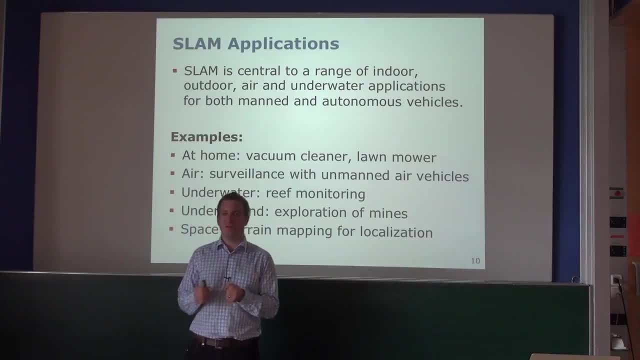 So the robot cannot move. Then you don't have a localization problem and you typically don't have a mapping problem, And that's a way of how industrial robotics solve this problem. But as soon as you have more flexible production lines where, let's say, 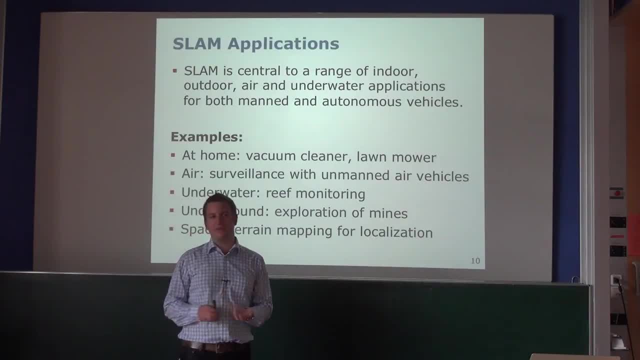 manipulators are on wheels and can drive freely in the environment, this really becomes an issue, And even for other applications. so if you have For every kind of whatever logistics service task where a robot needs to transport goods from A to B, this technique is needed. 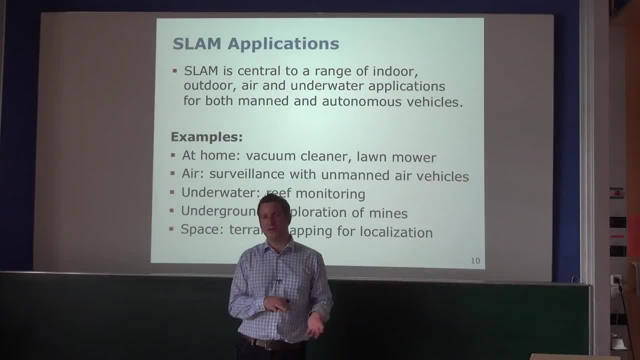 You can argue: oh, you can build a map once manually and give it to the robot and only do localization. It's partially true, but still, if someone changes something in the environment, if new goods arrive and the path is blocked or it needs to replan, 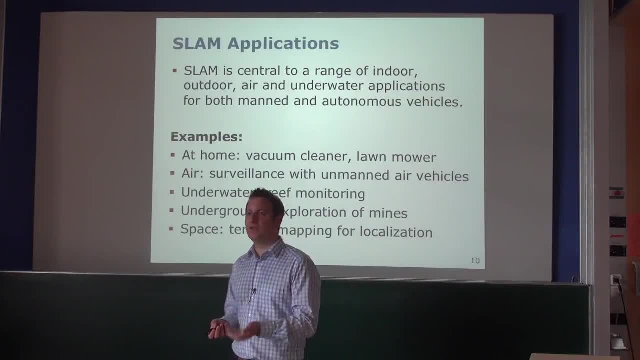 how can all this be taken into account? So having a working SLAM system that solves mapping and localization at the same point in time is not something which is just academically interesting, or interesting from an academic standpoint, but it's also a direct impact. 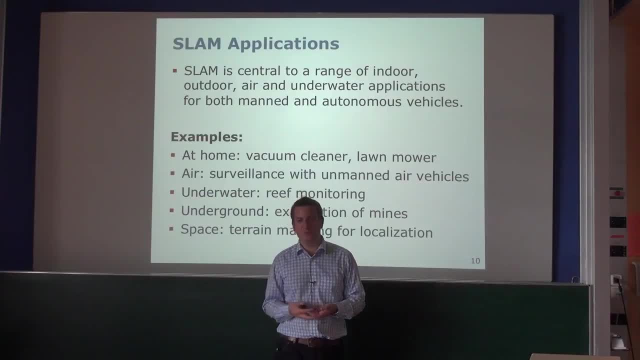 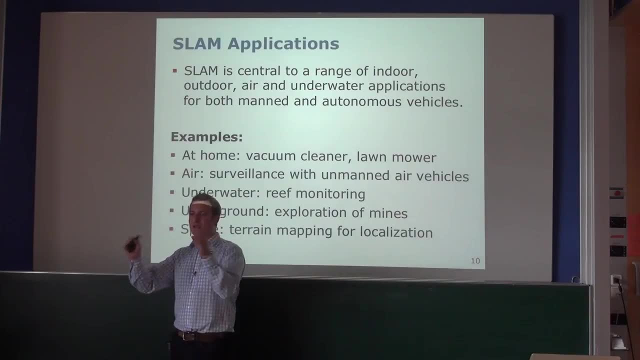 on real-world applications And today there are some systems which can actually solve the SLAM problem quite well. Sometimes it's compromised between having a good estimation technique and making some assumptions about the environment, or having certain requirements, like a certain type of landmarks. 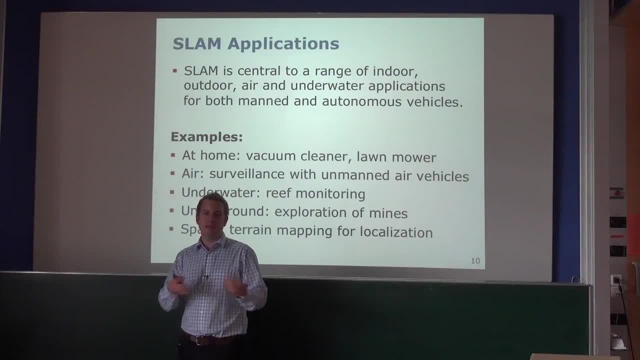 that are ensured to be always visible. so some constraints that maybe need to be fulfilled on a factory floor, And if these constraints are fulfilled, the system is guaranteed or not guaranteed, but it's very likely to work. So there are compromises between that. 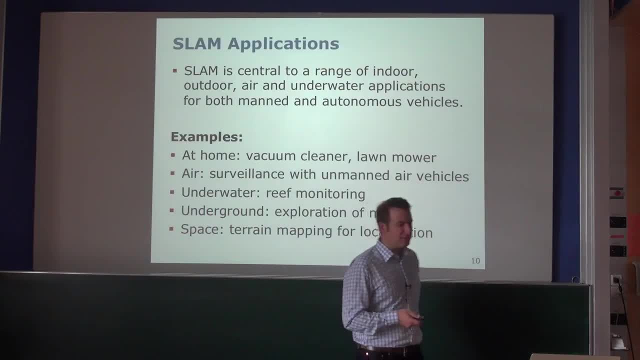 but SLAM is still an open and interesting problem. So there are different applications that you can envision. So, for example, in your home environment, you can think about your Hoover, your autonomous Hoover robot. You may have whatever a Roomba robot at home. 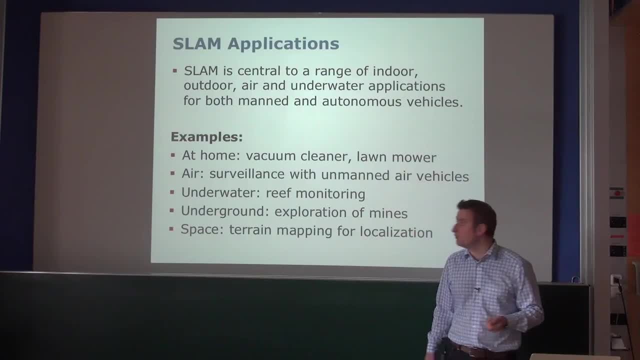 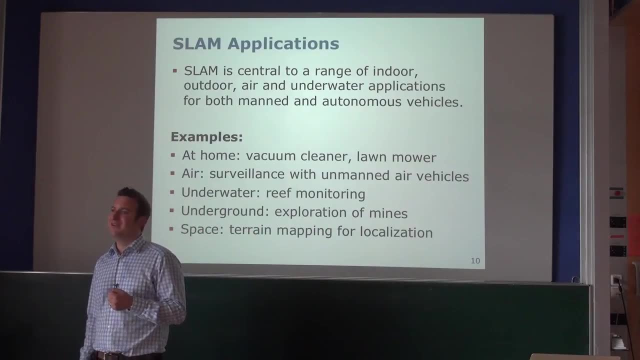 which is kind of the one of the cheapest robots you can have for roving your ground. This robot actually has also an interesting strategy that it says: I actually ignore the SLAM problem, I just do random walk, I just drive randomly through the environment. 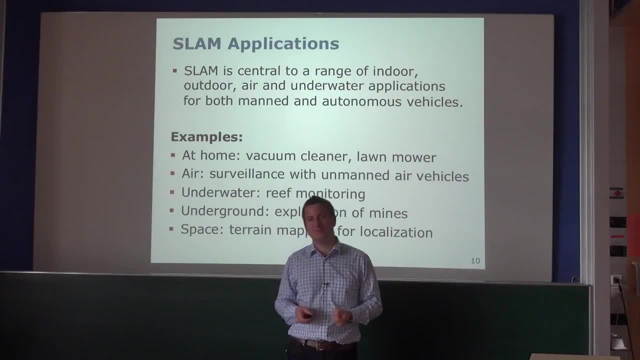 and as time goes to infinity, I will have cleaned that room. The advantage is that your room is small. This time it doesn't really need infinity. It doesn't need to approach infinity to actually clean your room. but it's kind of the very uninformed. 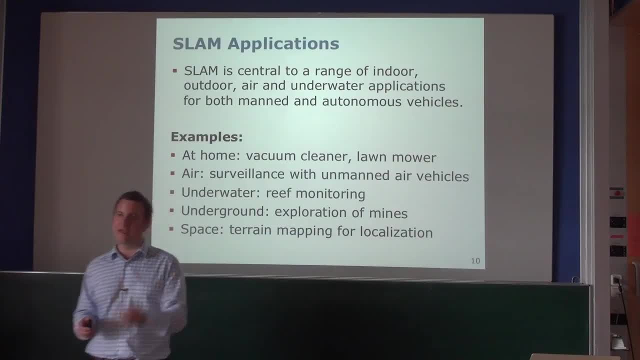 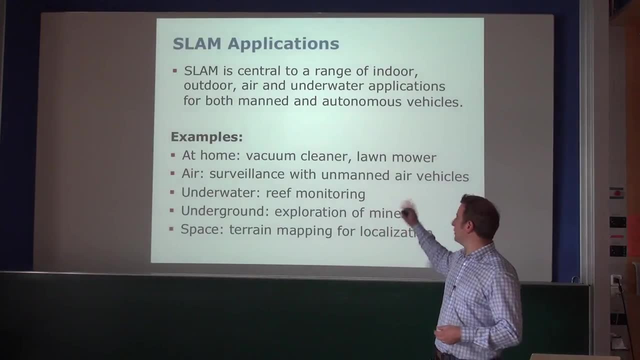 very, very trivial approach. Whenever you want to have some systematic cleaning or some guarantees you can provide, then you would need to go beyond that. It gets a little bit more tricky for lawn mowers, So autonomous lawn mowing is also something where 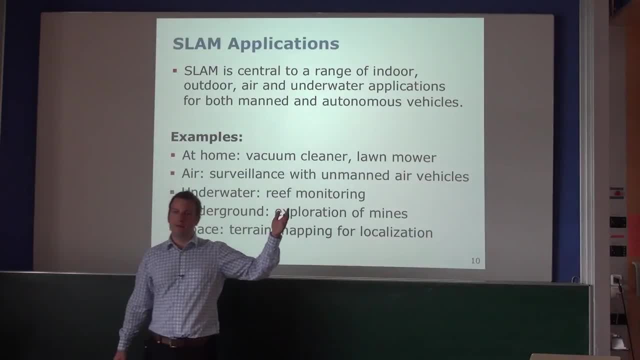 you can actually not buy. go to whatever every big Home Depot-like store and for whatever less than 2,000 euro you will actually find an autonomous lawn mower. They get a little bit better in that sense. Also, they typically don't. 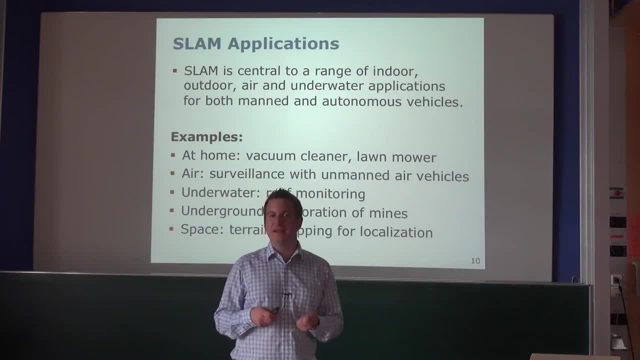 explicitly build a map, but they typically need- want to know where their charging station is, because at some point in time they need to go back. So again, here's kind of they typically do a compromise here, so you have to install. 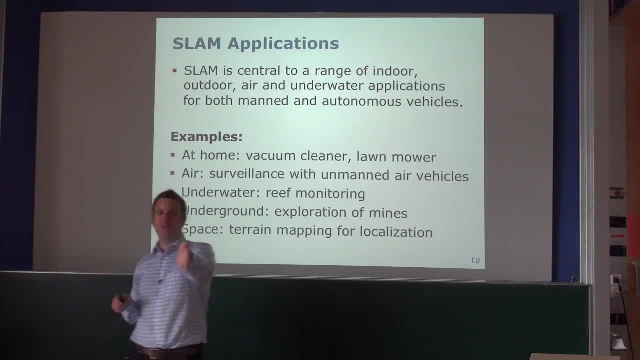 some wires in your garden. Whenever the robot drives over this wire, it can actually say: okay, I shouldn't go here. So therefore you can prevent your robot whatever falling in your pool or whatever can happen. So it also helps the robot. 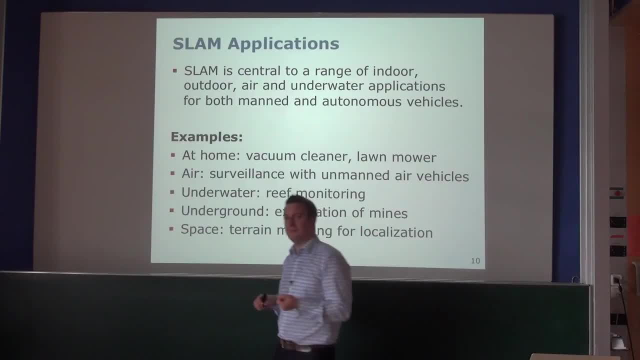 maybe drive back to its base station, for example, recharge. So they compromise. but the lawn mowing industry right now is really, really interested in getting that SLAM problem solved in a really, really robust manner, because they wonder what the people need. 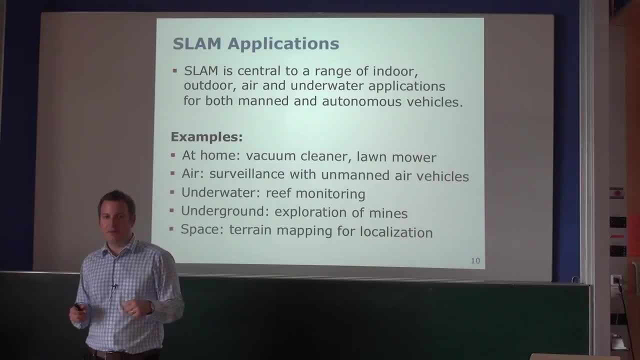 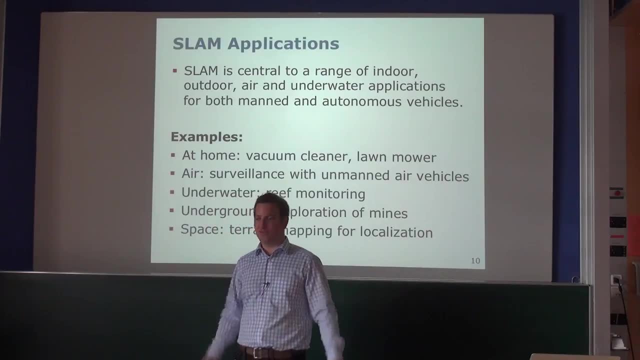 to install this wire below their lawn that allows the robot to work safely or operate safely. So there's real interest in kind of getting rid of that. just putting the robot there, switching it on, maybe telling him: don't go here. 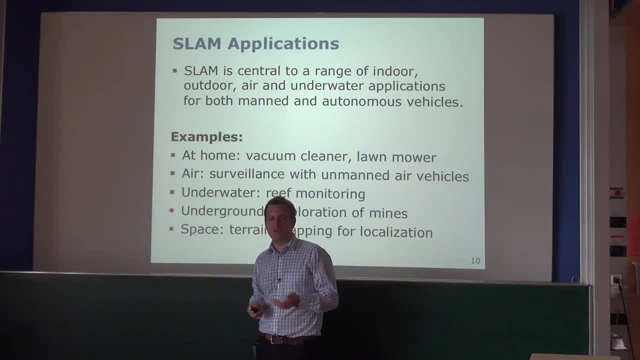 don't go there, but then go ahead and start working without having whatever an expensive or time-consuming installation which needs to be done, And so that's another application. There are other applications, like unmanned aerial vehicles, surveillance tasks, for example, or land monitoring tasks. 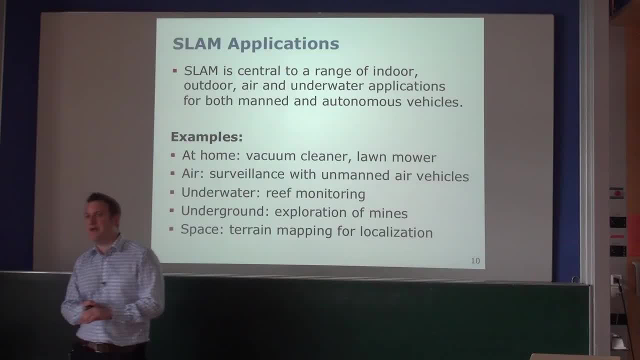 after disaster missions or for, for example, petroling and estimating the quality of the ground crops. crop sensing is also kind of a big agricultural application for autonomous airplanes or autonomous helicopters, So different kinds of surveillance tasks actually require to know where the robot actually is. 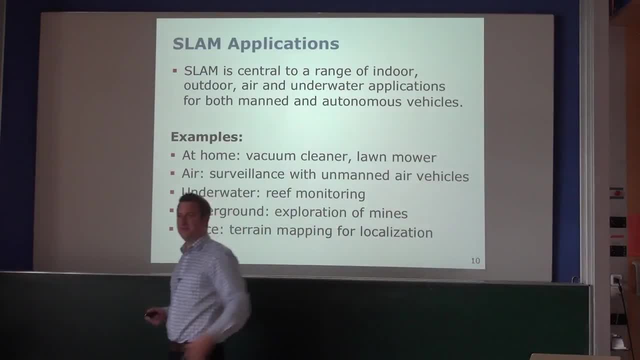 The advantage is for flying outdoor vehicles, at least if they are on a larger scale. GPS is a pretty good post-estimation technique, So they actually a lot of the problems simplify if you have those means at hand. but you may have applications. 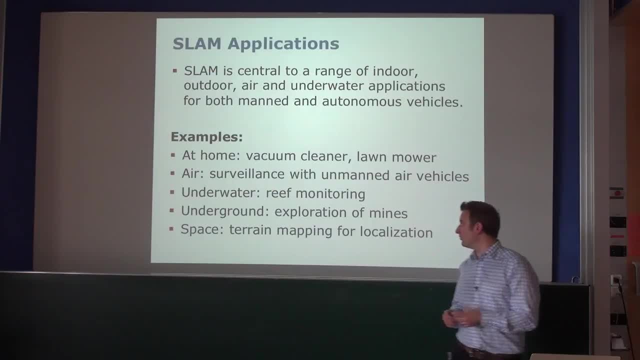 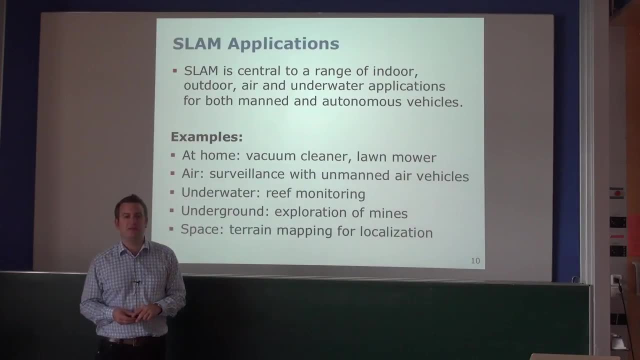 where you don't want to rely on GPS or where GPS is simply not available: Underwater robots or reef monitoring tasks. this is a pretty well-studied- not well-studied, but intensively investigated- field in Australia, for example. 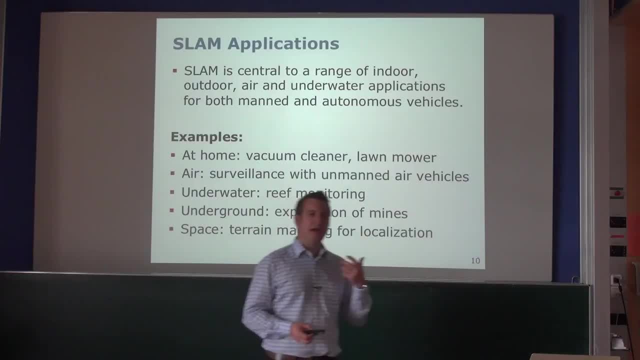 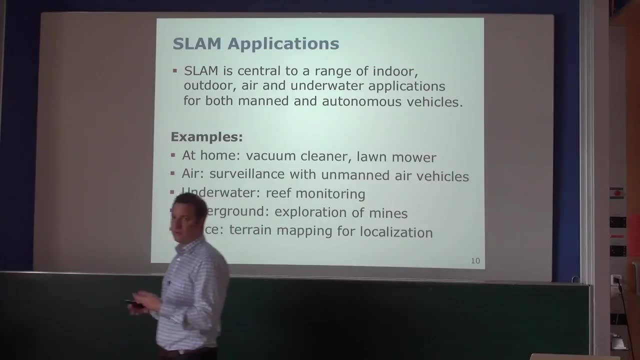 there's the Australian Center of Field Robotics in Sydney, which have a lot of boats, a lot of underwater robots that actually inspect reefs that met the ground and they want to, for example, also estimate how does the reef structure or the ground structure changes over time. 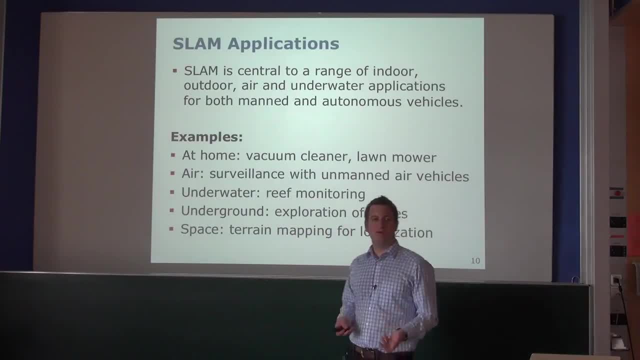 over the years, and so they want to be able to monitor the ground, build accurate models of the ground and relate missions over different years, estimating, hopefully, the same part of the environment. Then we have underground applications, whatever mine applications. 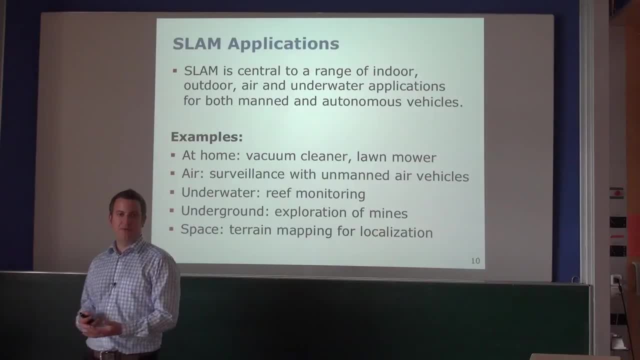 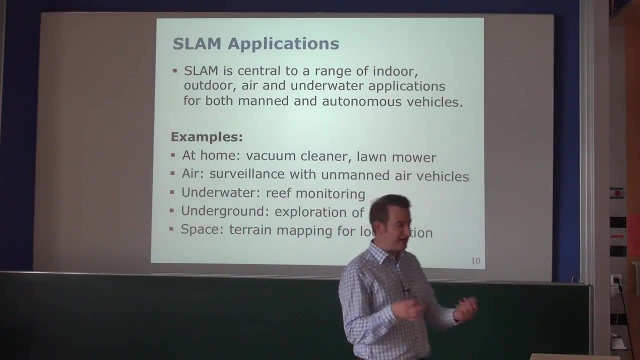 exploring mines. there are other applications which are of archaeological interest, where you want to have accurate 3D reconstruction of some small underground channels, paths, catacombs, whatever it is, and you also have space applications where you want to map an environment. 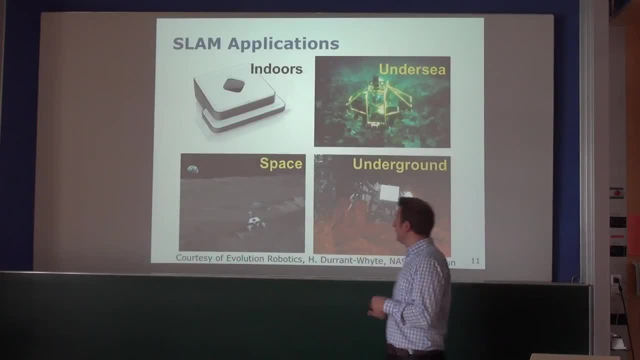 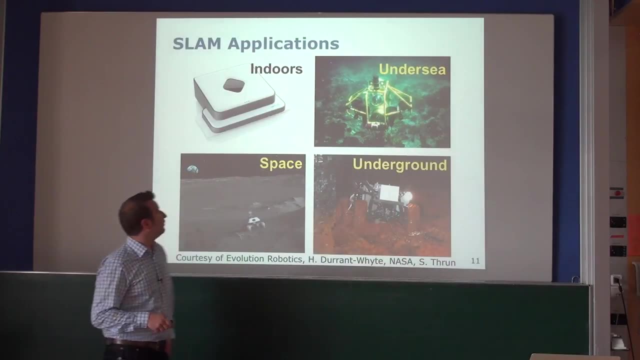 and do exploration missions in space. So these are typically, these are examples that you see. so what you see here is actually the Evolution Robotics Mint, now bought by iRobot, which is one of the kind of Swiffer-style robots. so you have kind of. 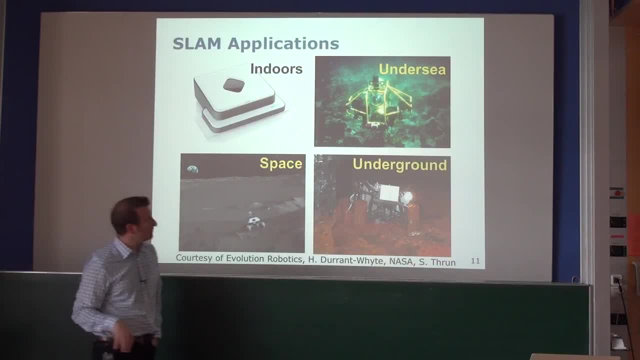 a Swiffer towel down here that would drive through the environment and systematically cleans your floor. This is one of Jeroen White's underwater robots at the Austrian Center of Field Robotics monitoring the ground. You have space exploration missions, or that's actually the exploration. 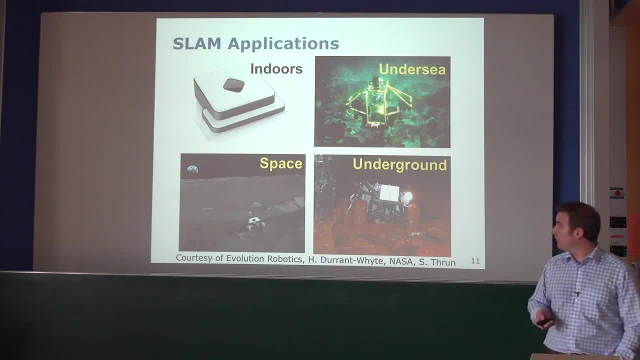 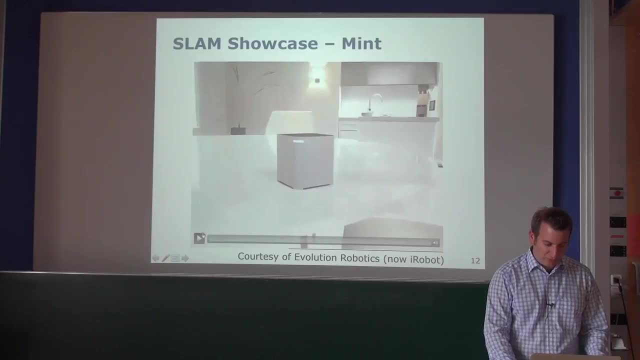 in close to Pittsburgh, done by Sebastian Thrun. So your typical applications that you find Also brought you a small video that's actually one of the showcase videos of the Mint system. Just let that play, see if it works. The secret is the revolutionary. 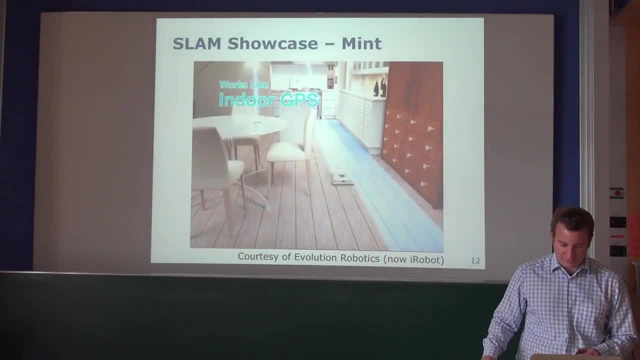 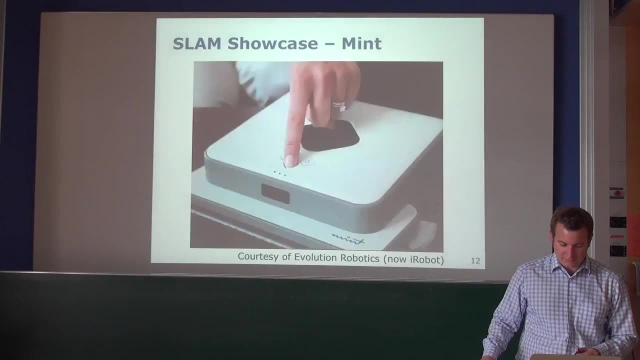 North Star navigation system. Simply place the North Star beacon in the area you want to clean and it works like indoor GPS so you can see where it cleans. so it sets Mint down on the floor and press run First. Mint covers the open floor area. 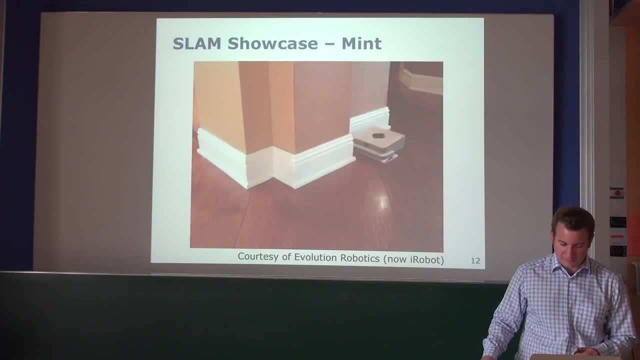 digitally mapping the room as it cleans. Then Mint spot cleans around furniture, legs or other obstacles. And finally, Mint meticulously cleans edges and corners using its advanced perfect edge technology. It doesn't rest until your floors are spotless. and Mint isn't just. 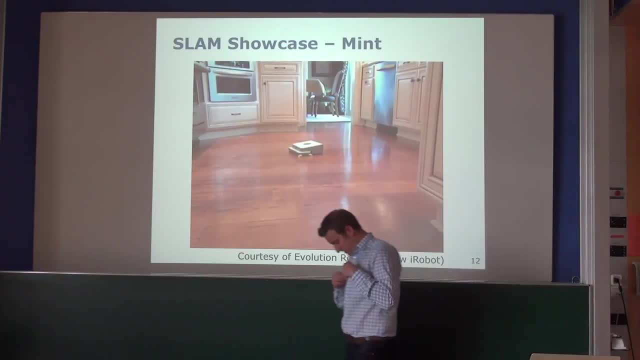 for dry cleaning. it mops too, Okay. so, as you could see here, you can see that the robot has a different slam problem in different ways. So there's a small box that you put on your table or somewhere in the environment that projects. 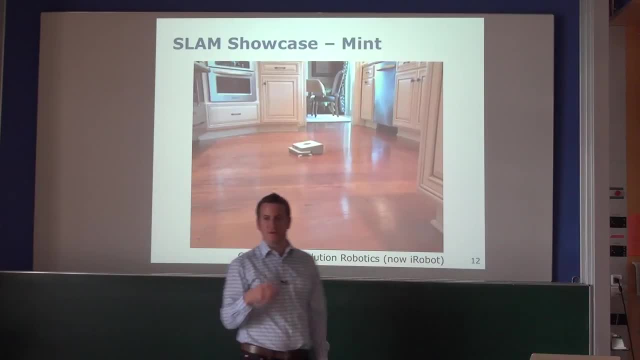 an infrared pattern to the ceiling, And so this is kind of turns out to be the map for the robot or the means for localizing. The robot has upwards facing infrared cameras and observes this pattern and therefore knows where it is. So it actually. 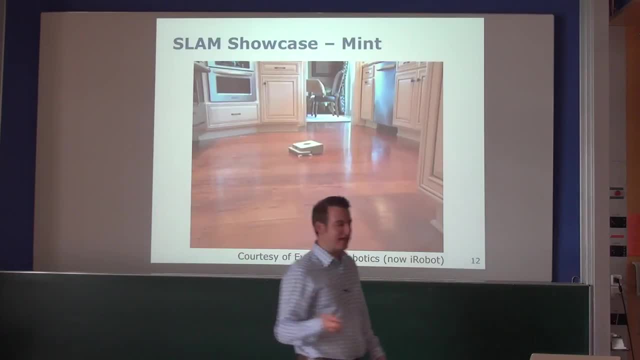 estimates its pose on the backs of the chairs and things like that, And so that's kind of one way how they solved the- actually in a quite elegant way- the pose estimation problem, because there's no expensive setup, you just need to put that box somewhere. 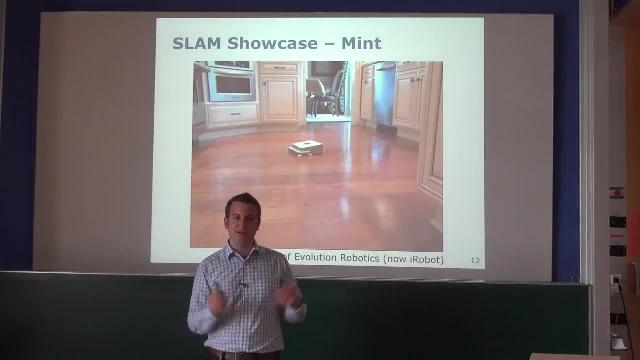 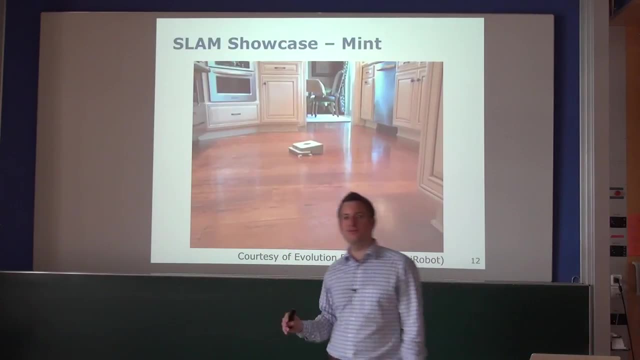 switch it on and it's an invisible pattern at your ceiling. But, for example, I'm not sure how well it works if you have these really old buildings with really high ceiling- that's questionable. Or if you have a robot which goes to different rooms. 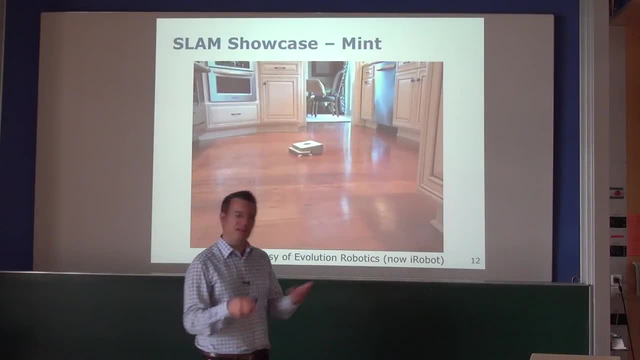 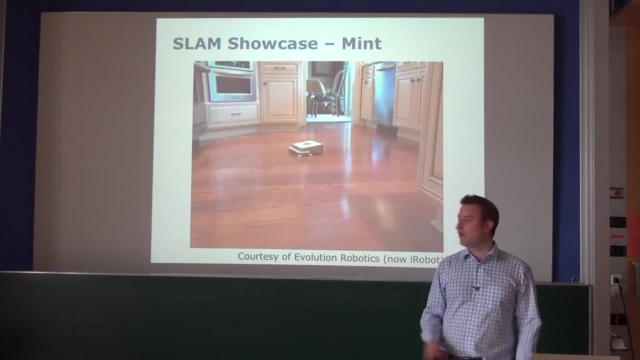 you would have multiple of those different base stations somewhere, let's say, sub-optimal compared to having a system which could solve the same problem completely on its own. But of course the advantage here for those products is price and those devices are. 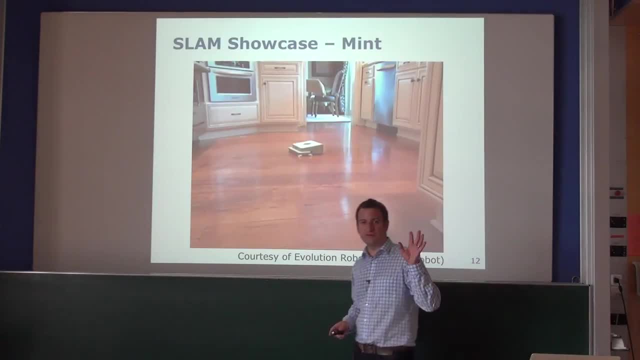 I'm not sure what the current price for this is, but last year it was, or two years ago it was in the order of 400 to 500 US dollars, so whatever- 300 Euro. So if you have devices at that price, 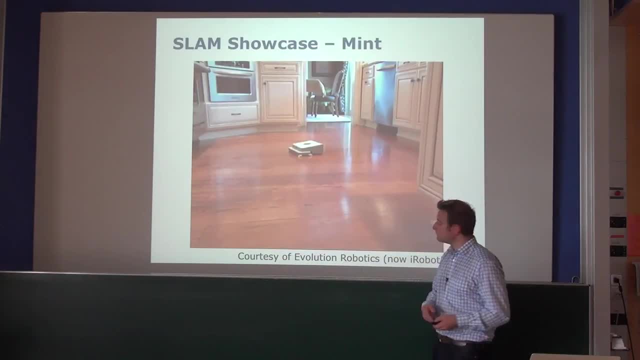 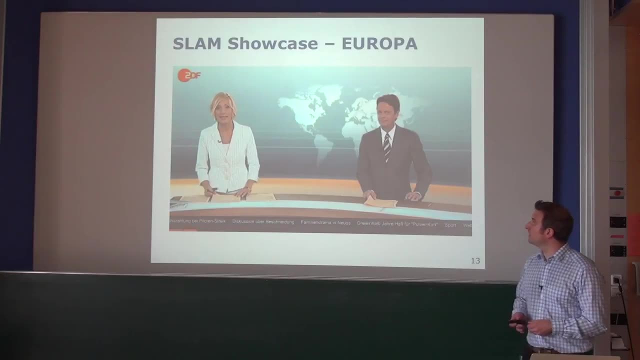 you typically need to make compromises at some point. We have another showcase, which is actually here from Freiburg, which is the Europa project. That's a project we conducted here on urban navigation. We had a robot which was navigating through the environment and it was. 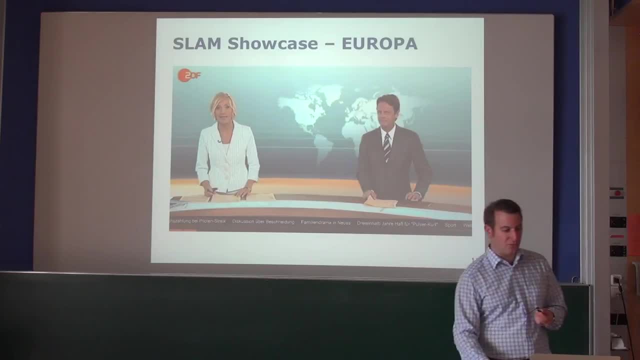 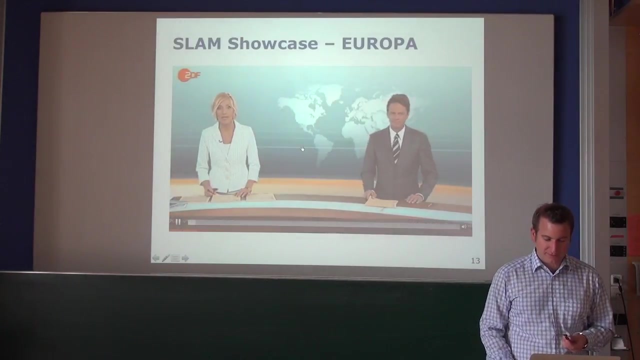 summer last year, when it made it through, starting from here, going to Freiburg downtown and navigating autonomously, which is also required by some mapping tasks in Europe. Einen Roboter auf Wanderschaft in Freiburg zeigen wir Ihnen Von Wissenschaftlern. 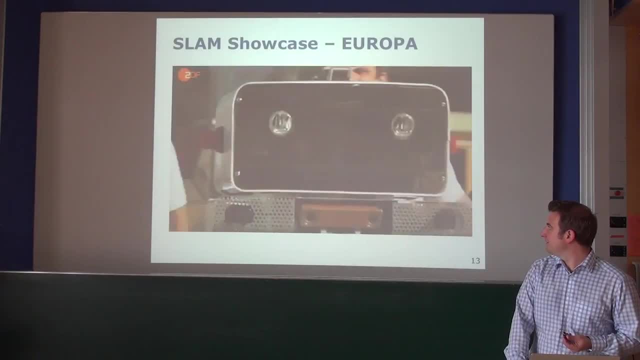 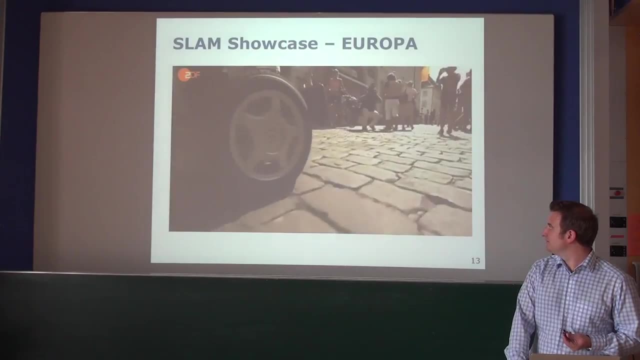 begleitet, musste die Maschine selbstständig ihren vier Kilometer langen Weg in die Innenstadt finden. Das klappt mit Hilfe von Sensoren und Scannern, die zehn Mal pro Sekunde die Umgebung analysieren. 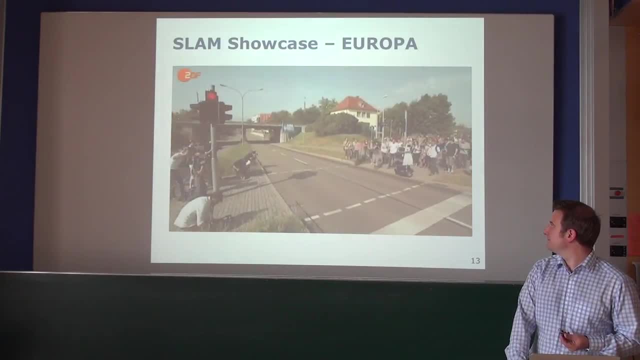 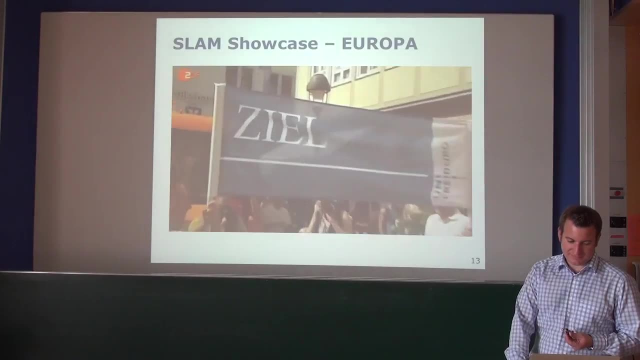 Nur an Ampeln mussten die Begleiter dem Roboter helfen. Farben erkennt er nämlich noch nicht. Nach zwei Stunden kam der Hightech-Wanderbursche unfallfrei ins Ziel. Solche wie Ihnen will die Roboterforschung. 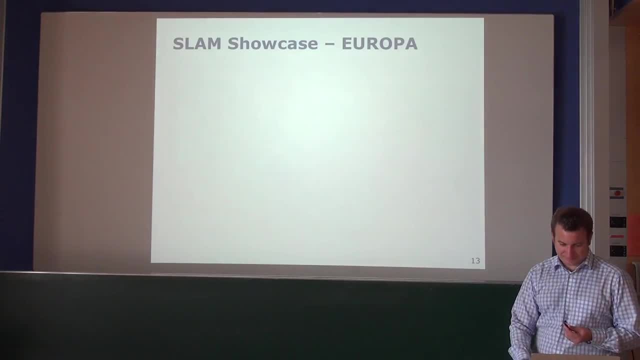 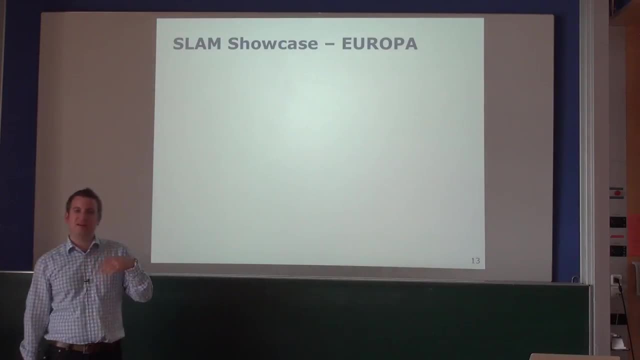 zu nützlichen Helfern entwickeln. Okay, So there are also other applications where this technology is used for building systems that navigate autonomously through the environment, and this is, for example, one of the technologies that you could imagine to work on autonomous transportation systems. 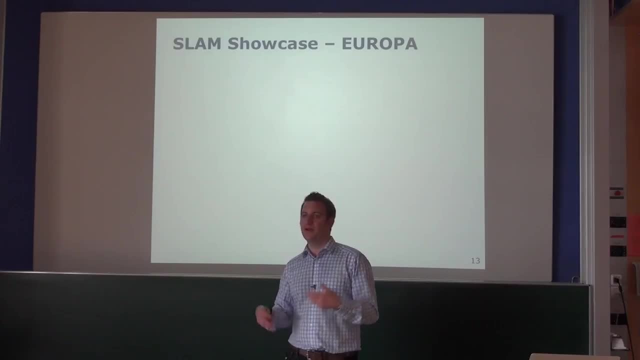 autonomous wheelchairs or other applications where you want to not modify the environment, so you don't want to put any beacons in downtown in order to go there. You want to have a system which carries also sensors, estimates where it can go, knows its pose. 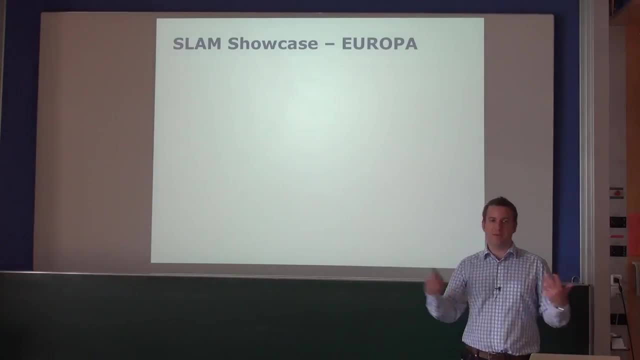 within a map and in this way solve the SRAM problem, which allows it to autonomously navigate. So navigation was kind of the key objective here. but in order to solve the navigation problem we actually needed to build accurate maps of the environment. This is another. 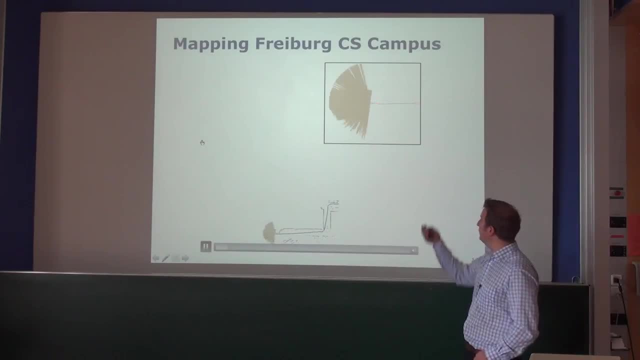 short example here: one of the mapping systems mapping our campus here. so that's a closed up view. This is a robot and this is kind of the proximity sensor which gives a distance to the closest obstacles. so the robot is driving around here, so you may start. 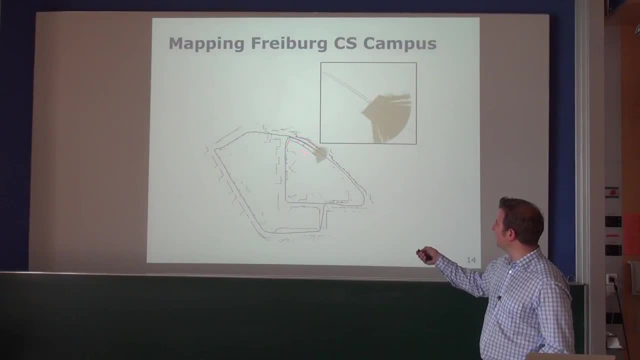 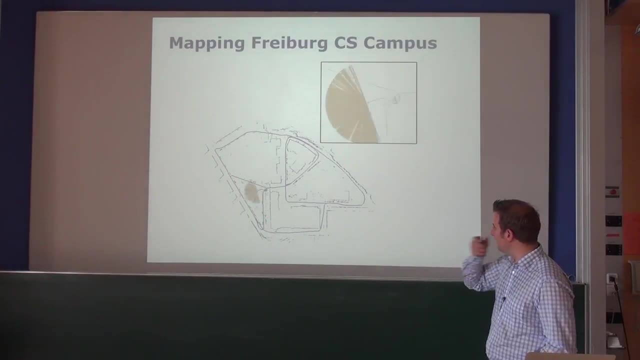 realizing what you see here. This is building 79.. This is the Mensa building. This is where the S-PAN goes. We are sitting in this building over here. That's the Dodge-Köhler Alley, and so you see the robot. 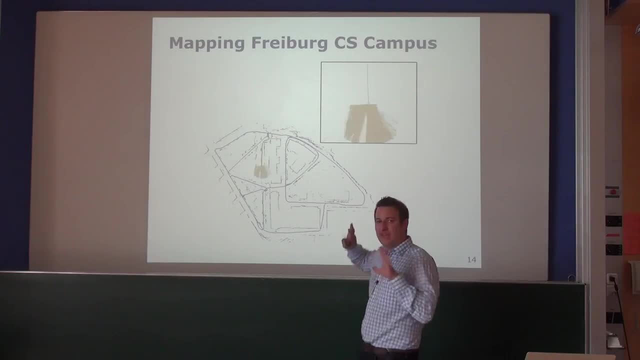 moving through the environment. Sometimes you see that map shaking a little bit. That's one of the post corrections that are conducted and so you can see. while the robot is moving through the environment, you can actually see the structure of those buildings, and this information is sufficient. 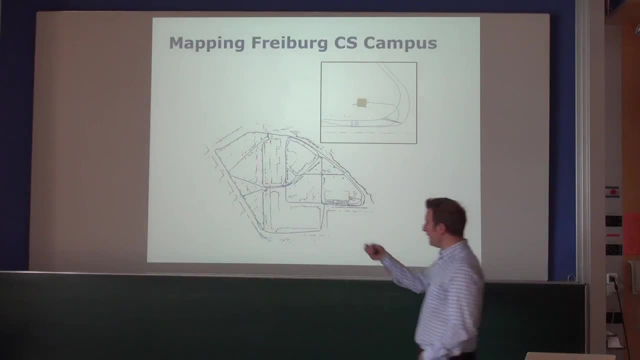 for example, for a robot to localize and navigate on campus. here, You may observe that the robot hasn't seen everything. so there are kind of white spots down here and there are other areas where part of the building structure is missing. That's just the reason for that. 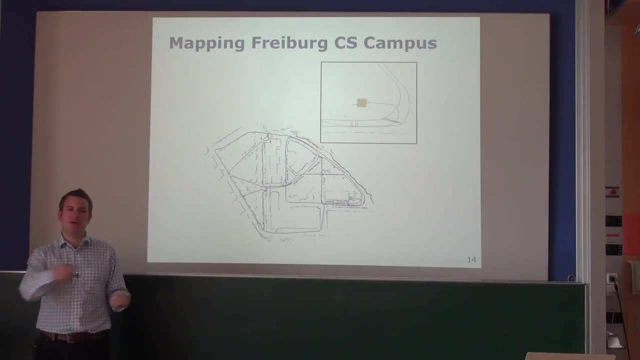 is that this is kind of a passive process. So someone drives the robot around, the robot records the map, but the SLAM system itself doesn't tell the robot where it should go to collect the information. Therefore, you have missed information, like down here in that area. 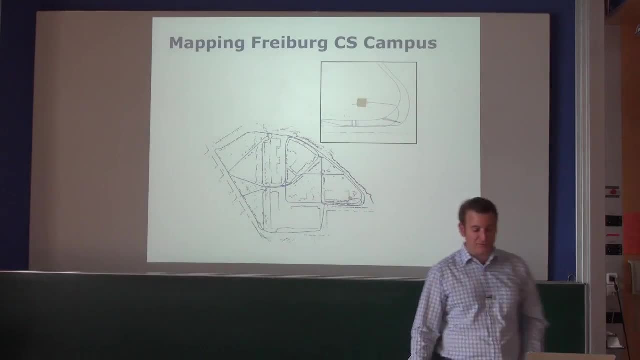 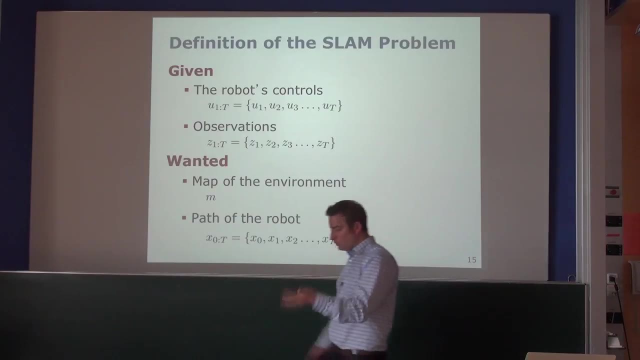 But that's kind of the typical result of SLAM algorithms. Okay, So let's dive a little bit deeper into that. What is typically? what do we have? what do we want? What we have is we have a sequence of control commands which tells me: 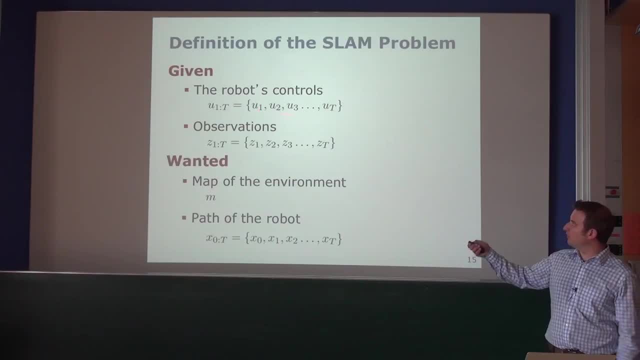 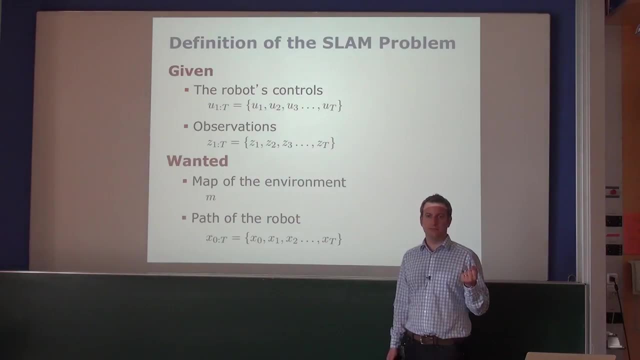 what are the commands I gave to the robot. This is what we call U1 to UT, So UT can be the command like: drive one meter forward, Or stop immediately, Or turn 20 degree to your left hand side. These are commands that are sent to the robot. 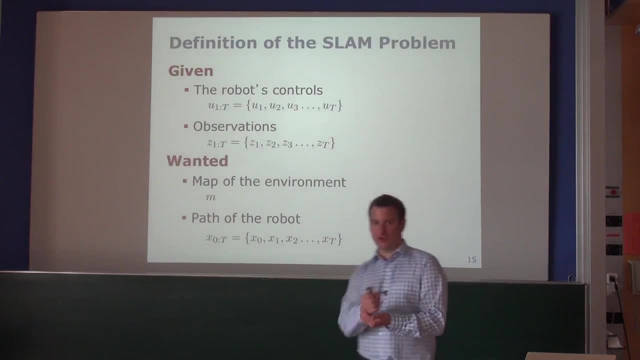 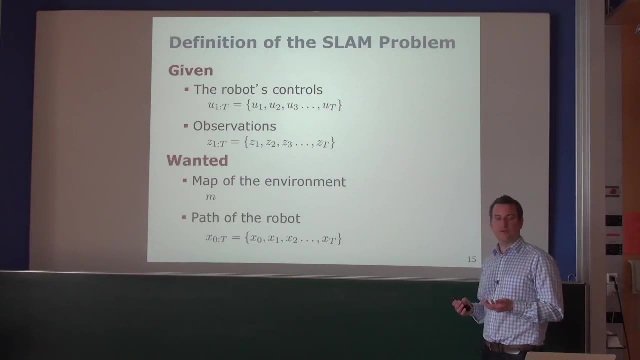 For example, why aren't persons operating the robot with a joystick? Or why an autonomous planning system, Whatever They are, controls and the robot tries to execute these controls, And these are specified by U1 to UT. So whenever you see a U in this course, 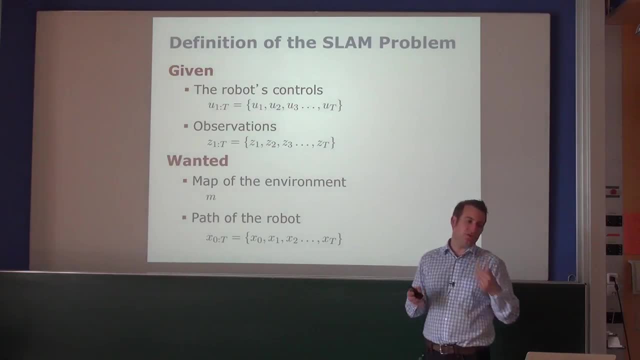 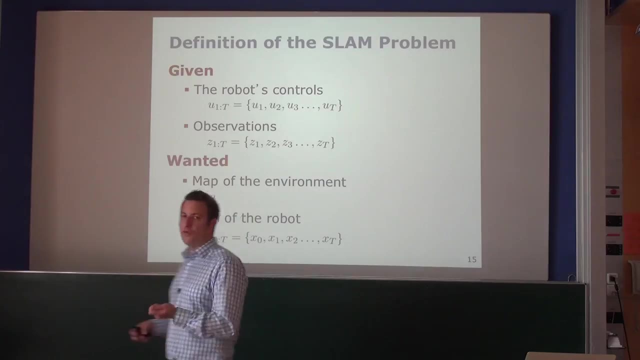 it means that's a control, Or sometimes we use- or we use actually controls and odometry information for actually the same thing. The difference is the control command is actually something which you physically sent to the robot, So like drive a meter forward. Odometry is something. 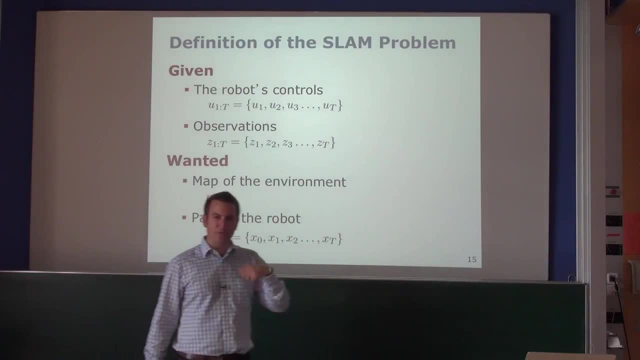 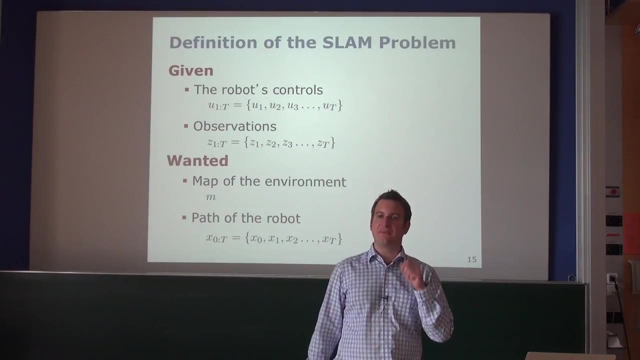 which, if the robot counts the revolution of its wheels to estimate how far has it gone, and reports this back. this is something which we call odometry. So it's already the first feedback from the system what it did. So it's one meter forward and the robot drives. 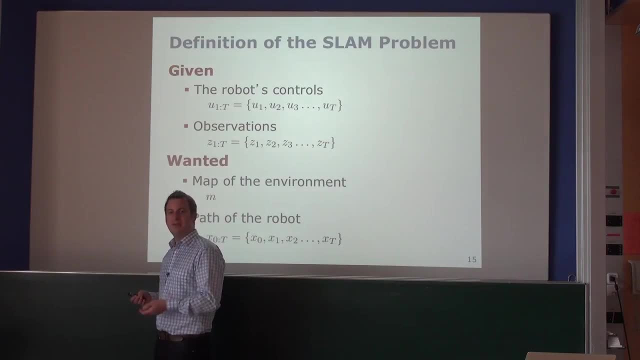 and stops and only drove 99 centimeters forward. Odometry may tell me you drove 99 centimeters, although the command was one meter. So it's kind of the it's already. actually it's already using sensor information, which is typically some encoder which counts the revolution. 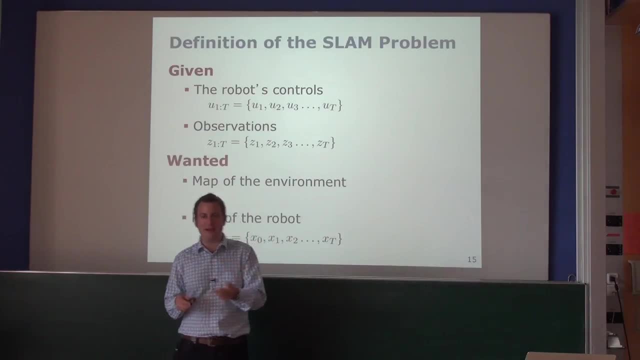 of the wheels And we typically use this as the command just because it's more accurate and we more or less get that for free from those platforms. But in theory it would be sufficient to just take the commands that are sent to the robot. The second thing: 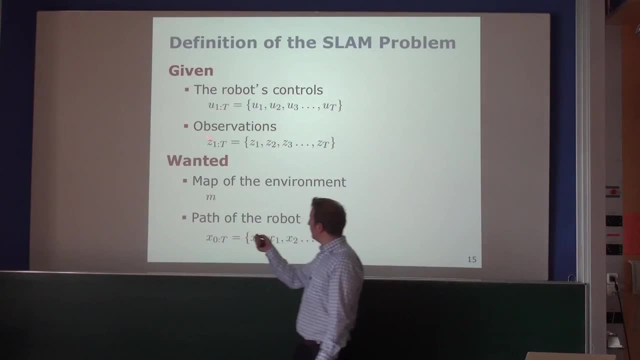 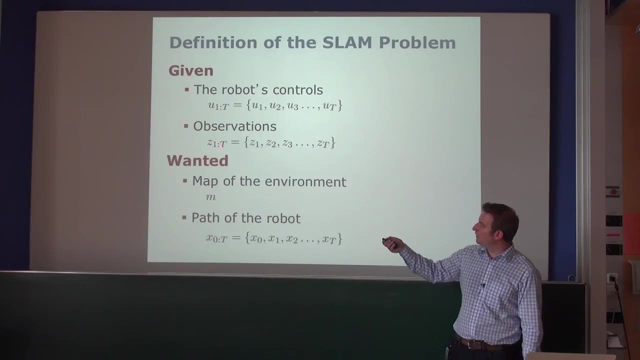 which is very important for us are observations, Typically always called Z or Z 1 to T. so these are these: 1 to T means at different points in time. so if I write it like this, 1 means 1 to T, so it means observation 1. 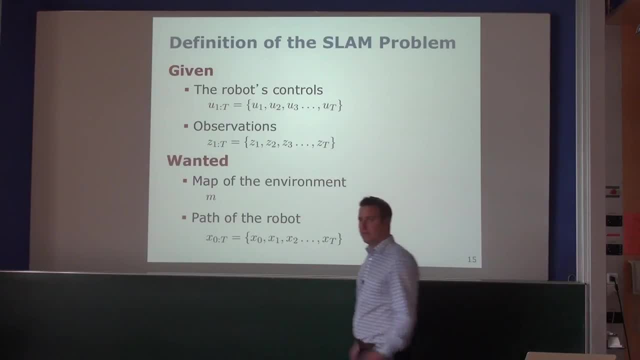 observation 2, observation 3 until observation T, So just different observations. These observations can be laser scans, So a single laser scan which tells me the proximity to the closest obstacle. It can be a camera image, whatever my robot has in terms of sensing capabilities. 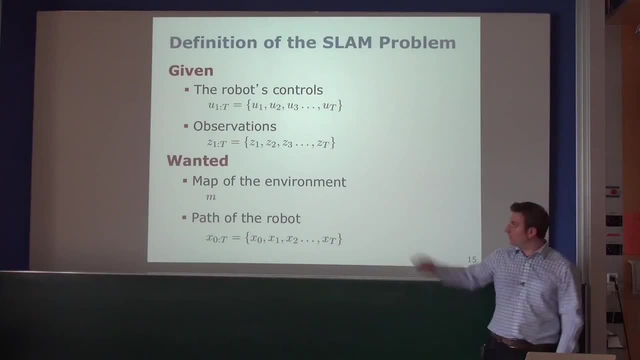 So these are my observations And what we so this is given, we have assumed to have that. What we want to do with that, we want to estimate a map of the environment, so what the environment looks like and the path of the robot. Note that the path. 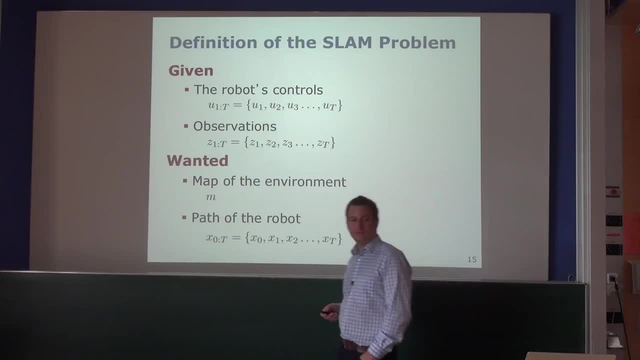 has typically one index, more so from X0 to T, whereas the commands go from 1 to T. The reason is, if I have a sequence of, let's say, 3 poses, between those 3 poses I can only execute 2. commands Go from 0 to 1. 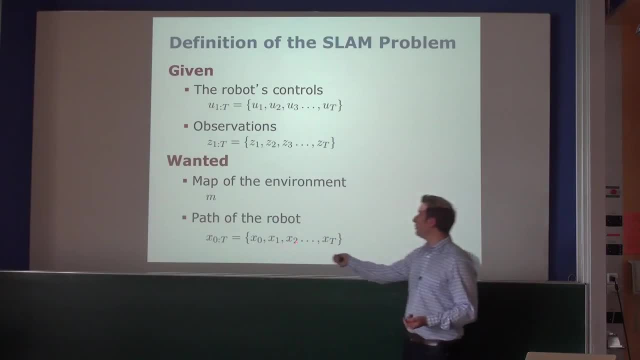 from 1 to 2. And therefore I typically have always 1 pose more than I have control commands. Yes, please, Shouldn't the observations too, start at 0, since you can't observe, You can have, but you typically the reason why it typically doesn't do that. 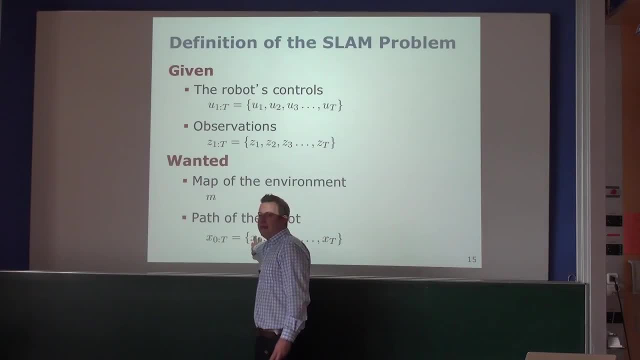 is that you use X0 to define the center of your coordinate system and then you start estimating with 1.. That's kind of the why you technically don't do that. You could also get an observation at the first point in time. that's absolutely right. 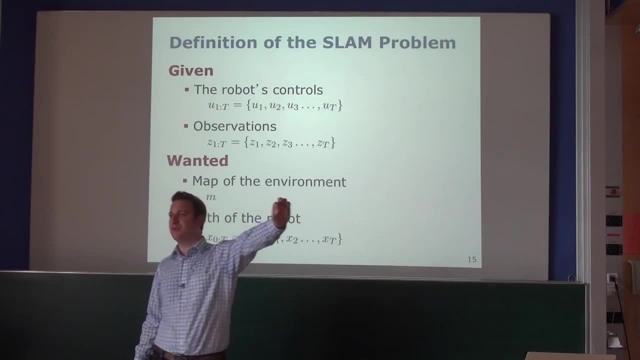 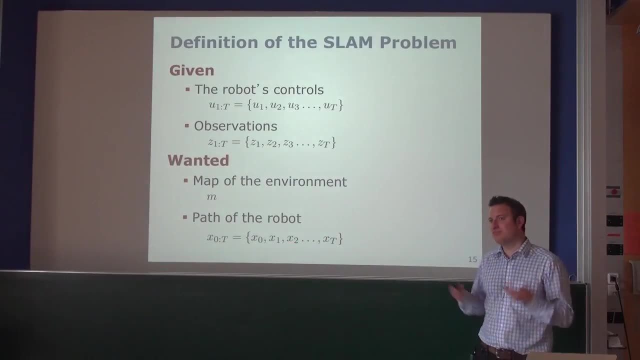 Quite often this X0 is just used to kind of fix a coordinate frame and then you start the estimation process with X1. But that's kind of more technical detail or something which is kind of typically used in the community to do it in that way. 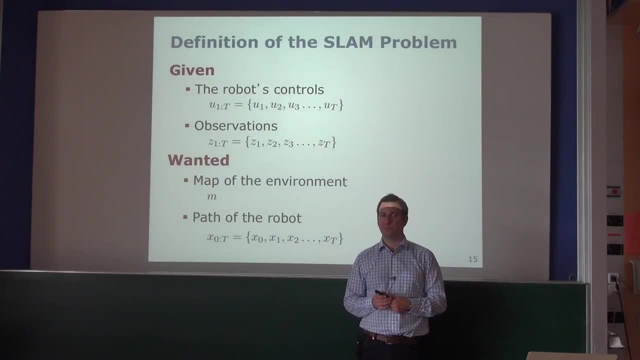 But in theory you're absolutely right. You could do that. Any further questions at that point in time. Okay, One important thing to note is these quantities here. they are not free of errors. They contain errors. This can be observation, noise, This can be. 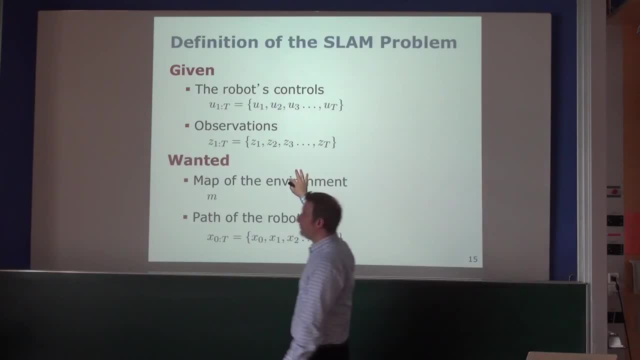 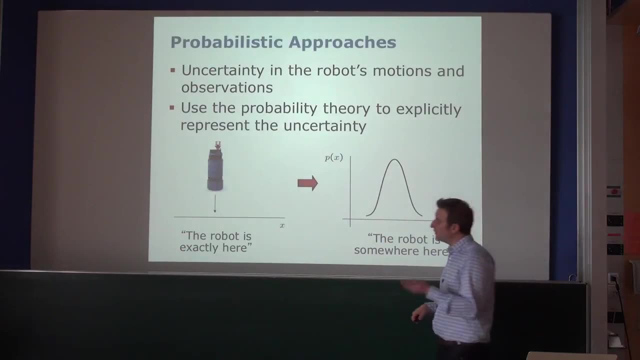 completely bad data associations. This data is not free of errors And therefore we typically use probabilistic approaches to address the SLAM problem. The same holds for mapping and for localization. Most of these techniques, at least the robust and successful ones, most of them. 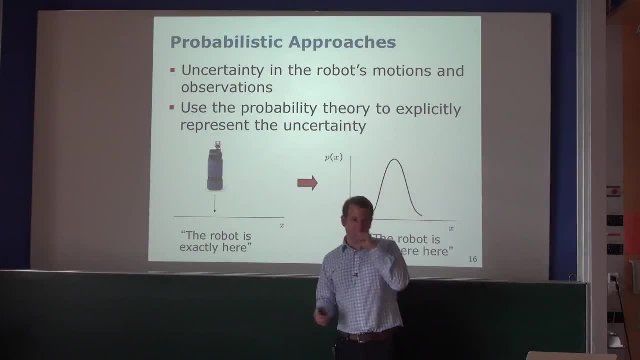 use probabilistic techniques. So to illustrate what that means using a probabilistic technique, you can describe that by looking at the distance between the robot is exactly here to the robot is somewhere over here. It's simply wrong to assume that you know where the robot. 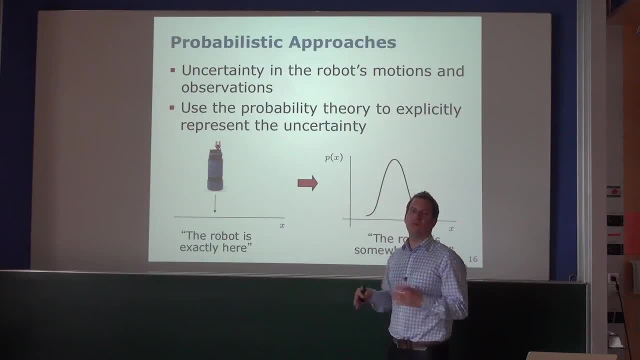 is perfectly, Even if you say, okay, the robot is here, I start on the robot and everything I do I do relative to the reference frame where the robot is right now. So the robot starts at 0, 0, 0, x0, y0. 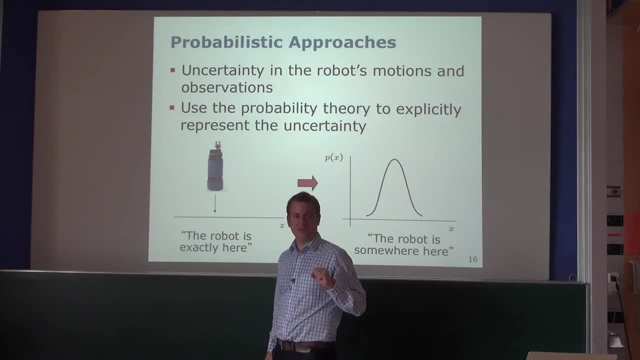 orientation 0. but if I say the robot go a meter forward, the robot may not be at 1 meter- x equals 1 meter- but at 99.99999 centimeters. So there's no. what I want to illustrate is that there's no way for us. 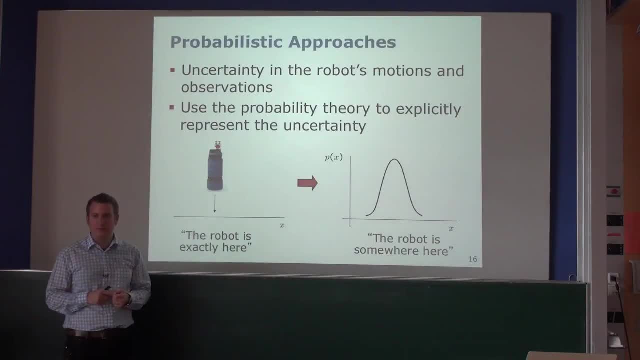 to tell that the robot exactly executed what we told it. We may argue that if the error is extremely small, we can actually neglect the uncertainty, which is true. So if this uncertainty, so this would be a sketch of a Gaussian distribution. if the uncertainty approaches: 0. 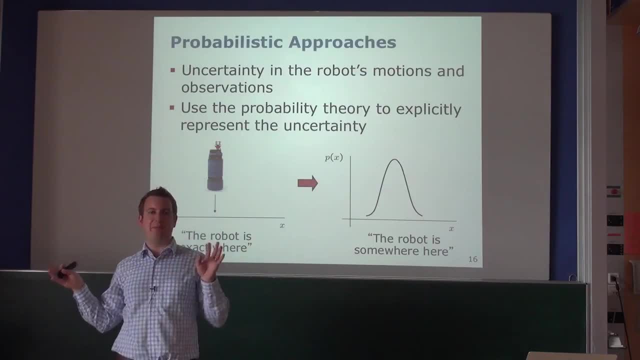 and I just get an extremely peak distribution. I may be completely happy with ignoring probabilities and just assuming I perfectly know where I am, But in most real world situations this is not the case. So we typically have an error which is non-neglectable. 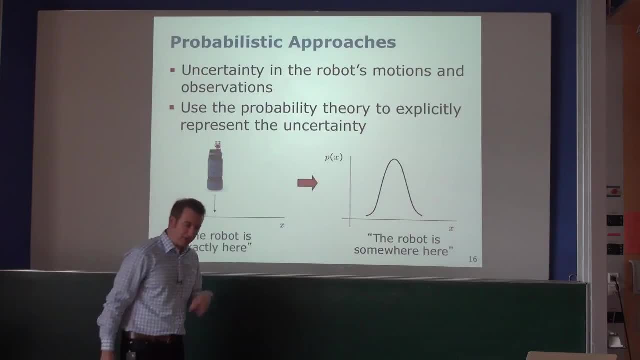 and typically the error even accumulates over time. So if I then say: go another meter forward, another meter forward, another meter forward, the error actually accumulates and gets larger and larger and larger. Therefore, at least at some point in time we need to take into account. 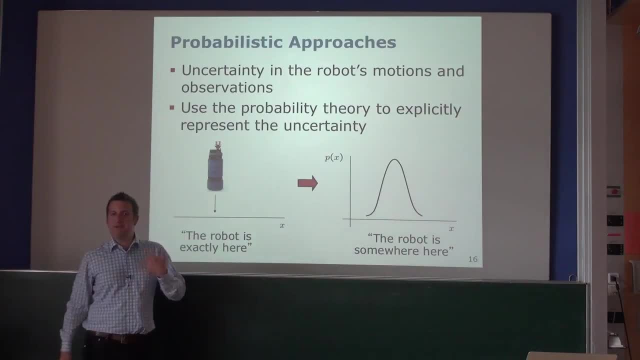 probabilistic approaches to appropriately model this uncertainty and maybe take this uncertainty into account. So if you consider the example of an extremely long corridor as a narrow doorway, at the end you start the robot in the middle of the corridor. the robot drives through the environment it completely ignores. 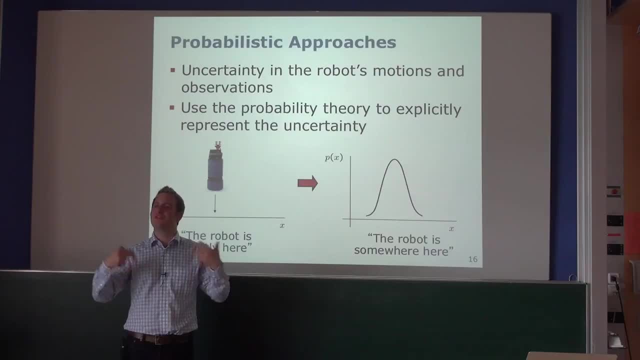 its observation because it has the perfect, or close to perfect, motion estimation system by just counting the revolution of the wheels. At some point in time it will make a small error to the right and left hand side At some point in time. it's super tiny. 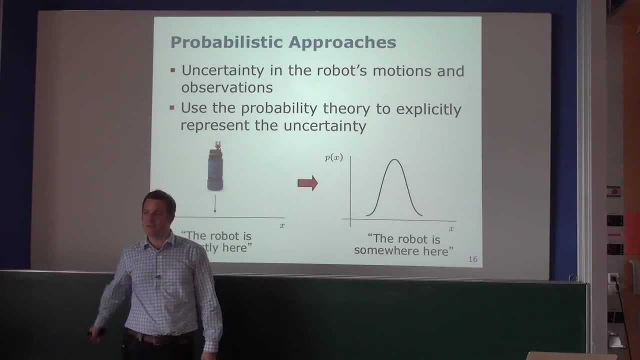 but as the corridor is very long, it may not pass through the door at the end of the corridor at all. And if you say, but I'm still super, super accurate, I just say, yeah, just make the corridor ten times longer, one hundred times longer, one thousand times longer. 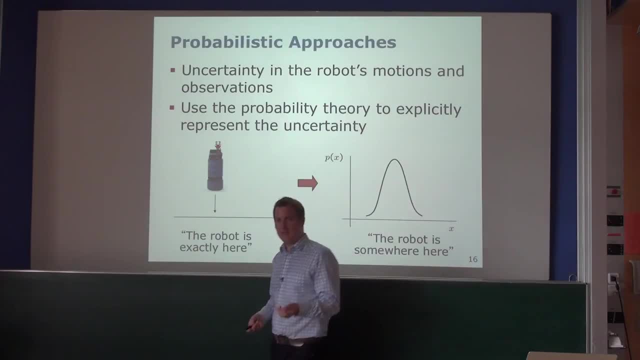 At some point in time you will actually collapse. And the same with these probabilistic techniques, in uncertainty. It may be the case that your sensor or your motion execution system is so accurate that you can ignore that, ignore the uncertainty, But if you scale up, 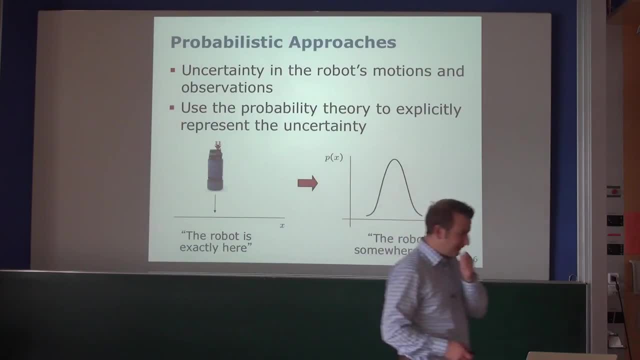 your problem at some point in time you typically run into problems again, And that's the reason why we use these probabilistic approaches for most of the techniques we do work here in robotics, so not only for mapping and localization, but for most of the real world. 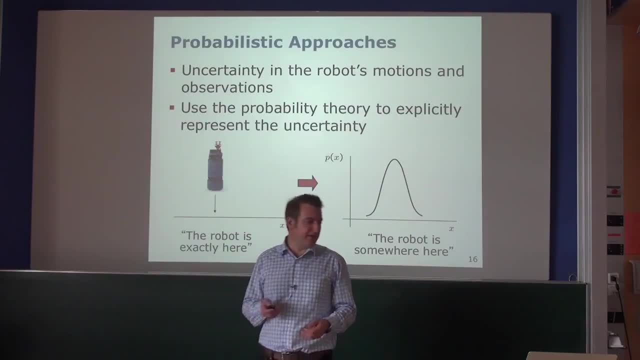 problems in robotics that we do. We use these probabilistic techniques because they're just very, very great tools to reason about uncertainty. They come at a price because modeling that is typically very challenging and computationally very expensive, and one often has to make simplifying assumptions. 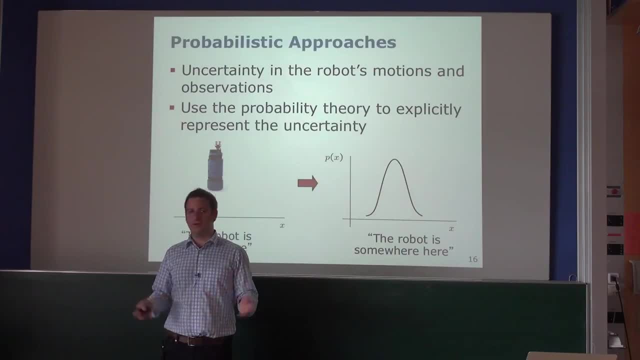 like the error is distributed according to a Gaussian distribution or something like that, but nevertheless it's better than saying there is no error. I perfectly know what the world looks like. OK, So what does it mean in the probabilistic world We said we want to solve? 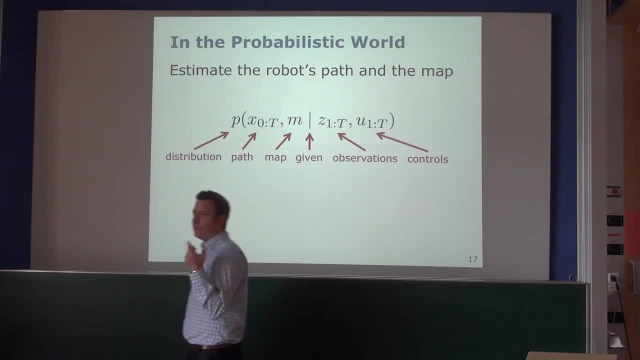 the SLAM problem. we want to estimate the path of the robot and what the environment looks like, So we can specify this in that way. So we have this p, of which is probability distribution. Then we have this x0 to t, which is the path. 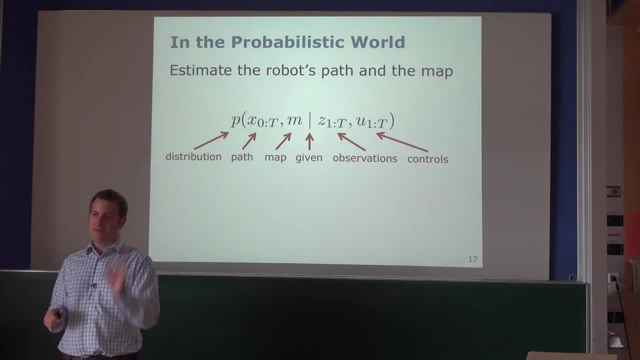 of the robot through the environment, its trajectory. It's going to fit the pose of the robot at discrete points in time. And then we also have the map that we want to know about. And then we have this strange vertical bar over here, which means given. 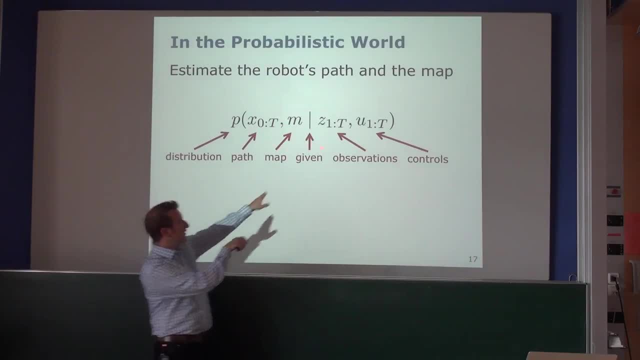 So we want to estimate the stuff which is here written in the front, given that we know what's written here behind that, that vertical line. What do we have here? We have our observations and we have our control commands or our odometry information And the whole thing. 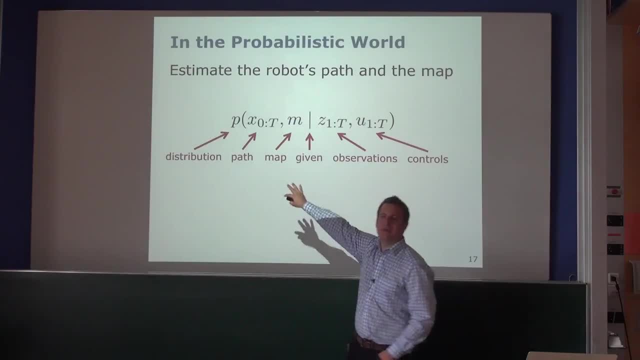 we're going to do in this course is just how can we actually estimate that probability distribution? That's kind of if I should present the course in one slide. that's actually what we're going to do And we're using different techniques to in order to get. 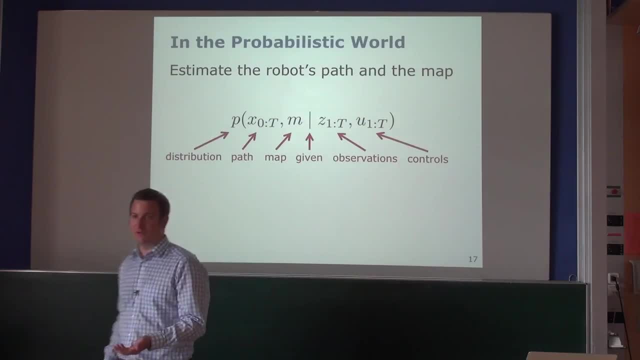 a hopefully good estimate about where the robot is and what the world looks like, And the choice of the technique that we use depends on the assumptions that we can make, If we can make assumptions- let's say we have distinct landmarks in the environment, We have certain 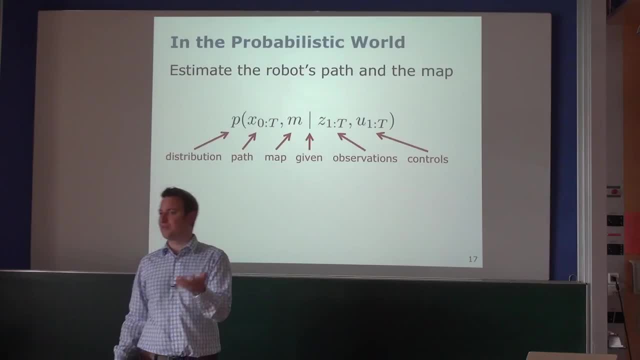 sensing probabilities, like if a sensor has a Gaussian error. there are certain estimation techniques which are well suited to solve that problem. If you say we have, we don't have landmarks. we just want to build a dense model of the environment so really represent all the physical surfaces. 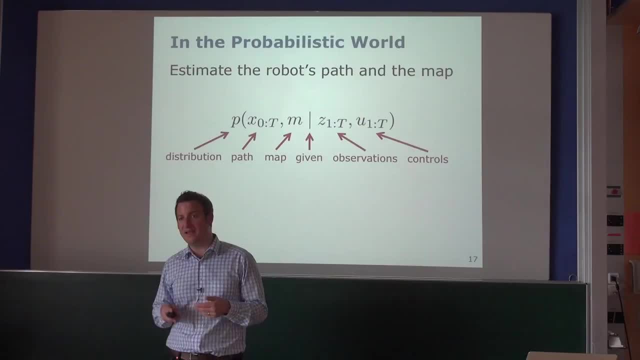 for example, in the scene, We may use something else. or if you say we have really really weird sensing properties like this- it's not at all a Gaussian, it's some other weird multimodal distribution- Then other estimation techniques should be used in order to get a good estimate. 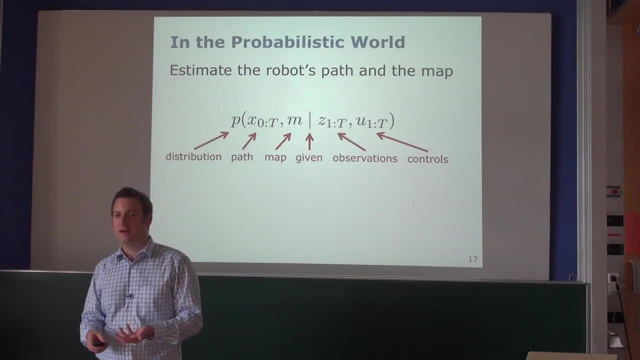 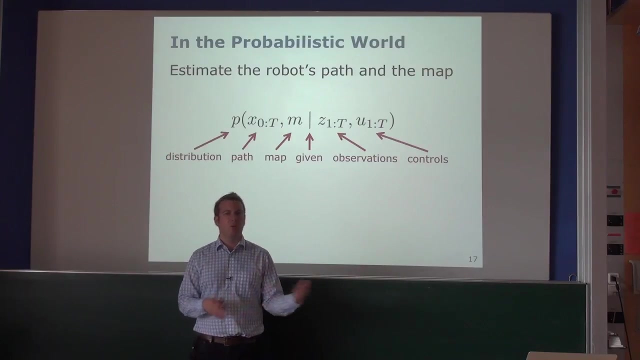 So all these estimation techniques make assumptions and some may be more restrictive in their assumptions. but then let's say, easier to implement, more efficient to execute, it can have an advantage if I can assume that these assumptions hold for the technique that I'm investigating, Or I may relax. 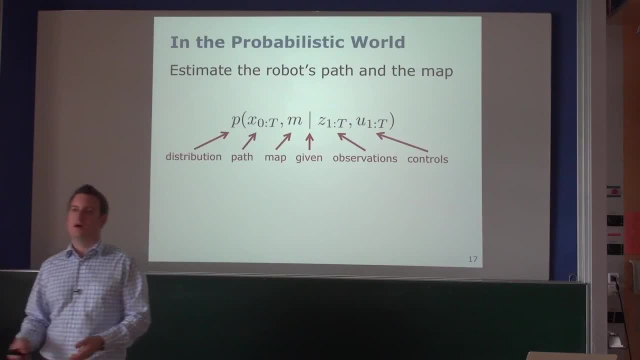 some assumptions, this may get computationally more expensive, but that's kind of the choice of the designer. We will look into three different paradigms here. One is a Kalman filter and family which is made for Gaussian distribution with particle filter based techniques which can have 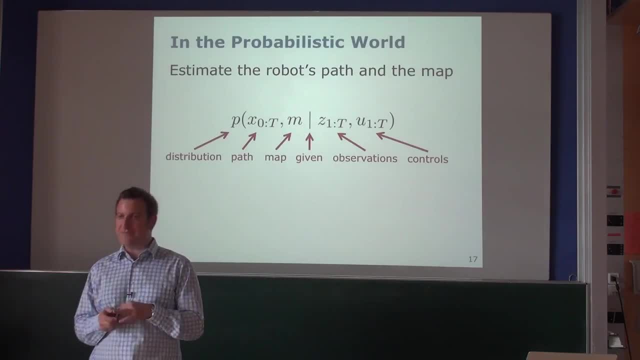 multimodal distributions and we have graph based approaches, which often assume Gaussians as well, but can relax it to a certain degree and better deal with outliers. They're computationally sometimes more demanding but have some other properties: that they are more flexible and how they can be used. 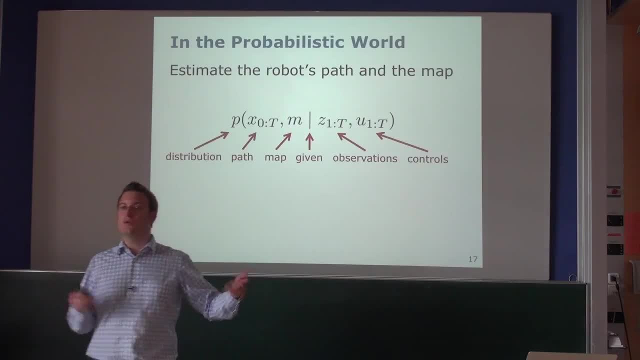 and can combine different sensing methodologies. We will look into these three different paradigms here and investigate them. Okay, so we said we want to estimate this guy over here, So this is something that we also call the full slam problem, And if you draw that, 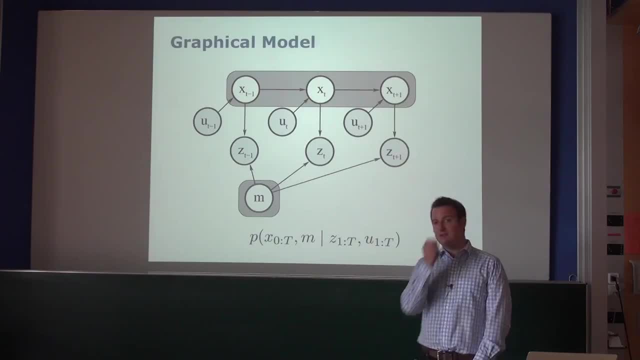 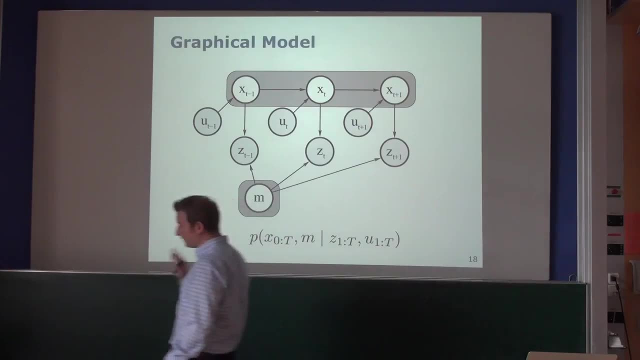 as a graphical model. it looks like this. So who of you has seen graphical models? Okay, so a bit more than half of that, Okay, so briefly explain what it is. So what you see here? you see these circles and you see variable names. 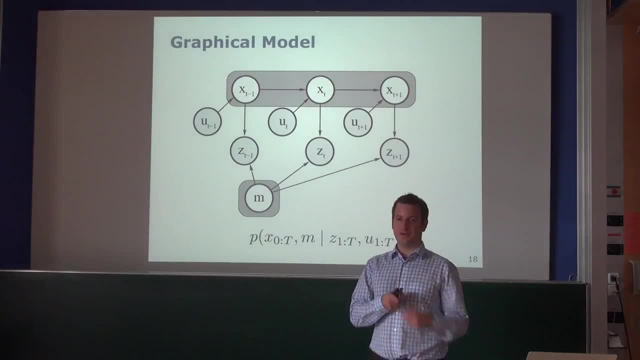 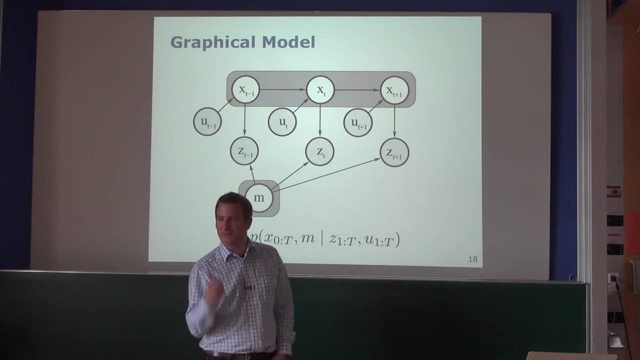 in these circles and those variable names you have seen before. So these are observations, these are controls, these are the positions of the robot, this is the map of the environment And these errors represent dependencies between those variables And you can actually read these errors as influences. 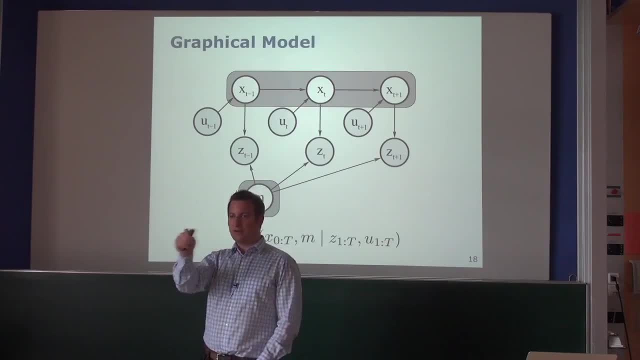 That's the easiest interpretation. Say: an error means influences. So, for example, if I'm interested in estimating the current pose xt of the robot, I look to the variable xt minus one. that is the position of the previous point in time, and there's an error. 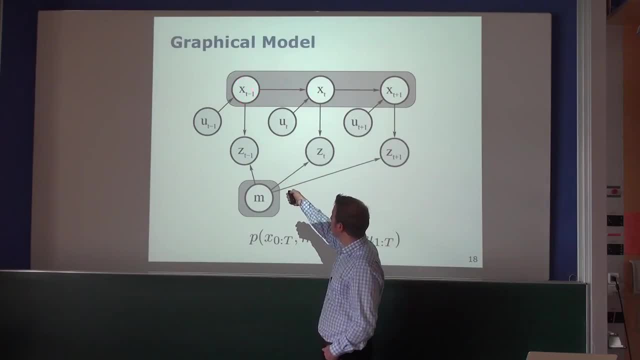 from xt minus one to xt, And I can see, I can read that, as xt minus one influences xt, Which makes absolutely sense if I know where I am right now or I have a pretty good estimate where I will be at the next point in time. 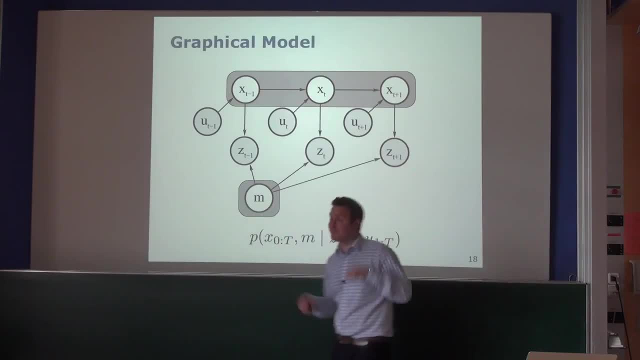 given that I cannot, whatever- travel at light speed somewhere else. So read those errors as influences. We can say, for example: here we have the previous pose and the odometry command executed. both influence the new position, If I know where I was and I know which. 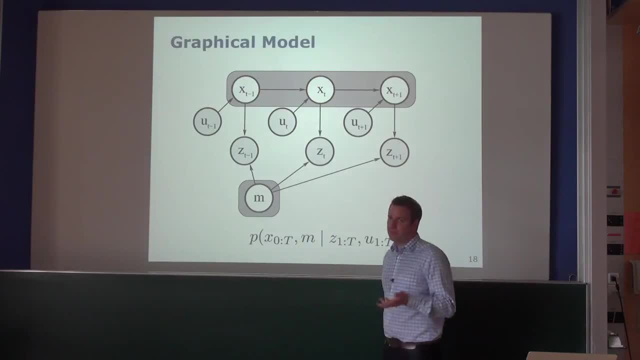 command I executed. I have a pretty good means to estimate where I am. So, given my, I've started here and I said: go one meter forward, go one meter forward. so I'm somewhere around this pose. with a quite high likelihood I'm not perfectly there. 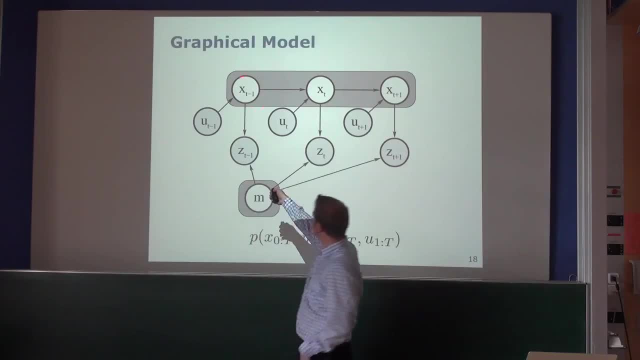 but I'm somewhere nearby And this can be expressed by this xt minus one error to xt and an error from ut minus one to ut. If you look to the observations, what we're going to observe depends on, for example, the landmark or the position of the whiteboard here. 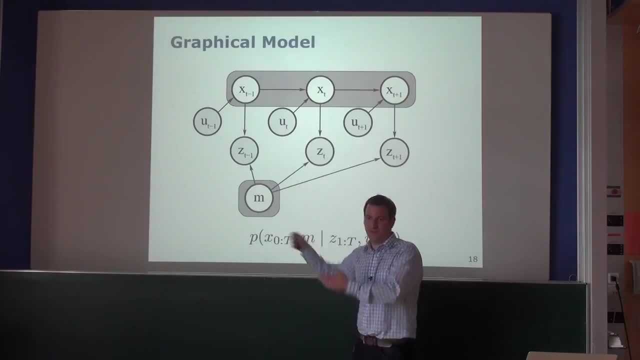 It depends what the world looks like. so where is the whiteboard in space? and it depends on where I am. If I'm here and observe the whiteboard, it would say, okay, it's a meter to my right hand side If I'm standing over here. 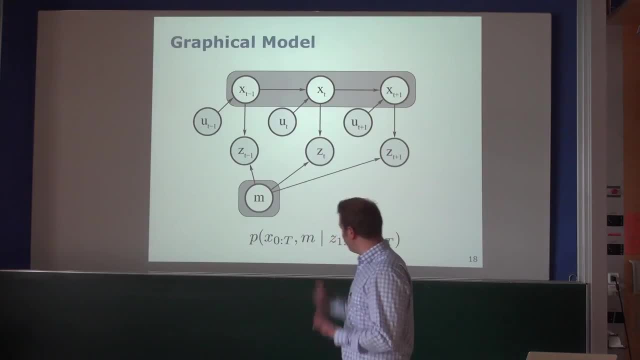 it would be two meters to my right hand side. So it first depends where is the whiteboard in the environment and where is the sensor, and if I have these two information I can probably get a good estimate of what I'm going to measure. And this please. 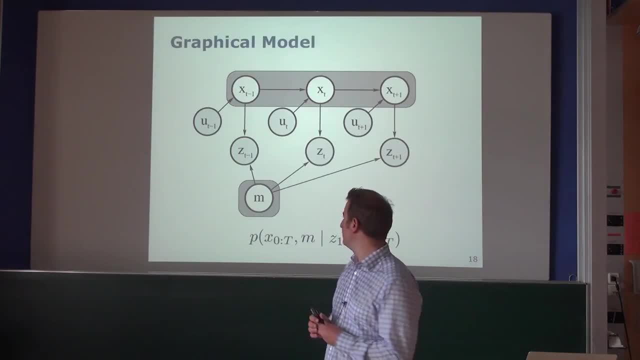 Is the m? is the map right, Yeah, or what? the environment, the environment. you can even see that at the environment. You can also see, if you see this as landmarks, let's say distinct landmarks. this is where are those landmarks in the world? So it's not the. 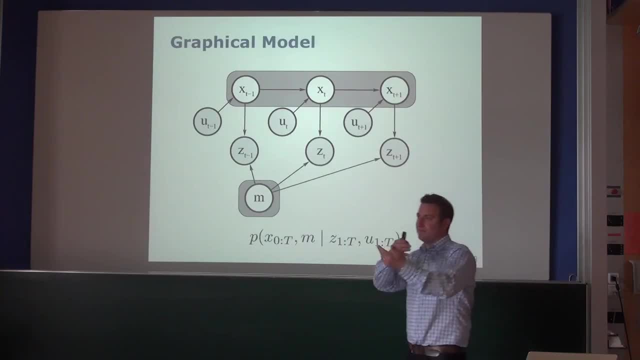 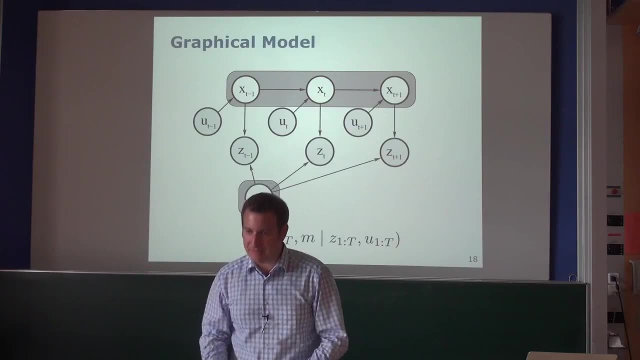 So it depends. so it's a good question. So the thing is, the important thing is what the world looks like. But given that I build a map, this map should tell me something what the world looks like. So the estimate, so my estimated map also tells me something about. 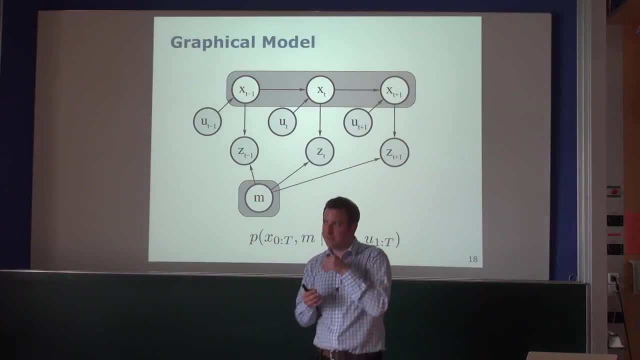 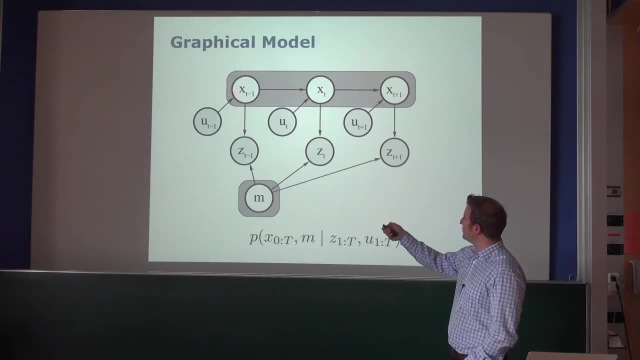 what I'm going to observe. But in general, you're right, What I'm interested in is the environment itself, Okay, And we have those variables which are here, which have this, this dark grey background over here. That means these are the variables we want to estimate. 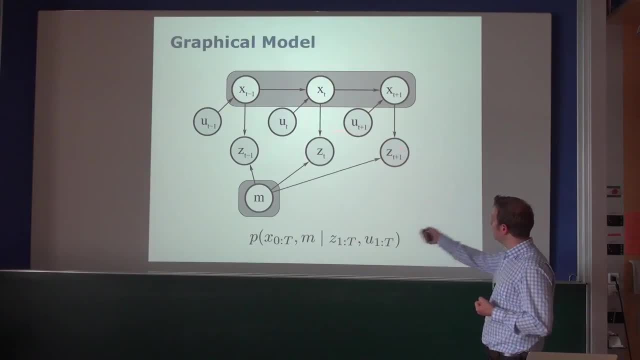 So these are our unknowns and the other variables, these grey variables here are our knowns. So these are the unknown quantities and these are the observed quantities And these graphical models. so we won't use them very often in this course. they're kind of a nice way. 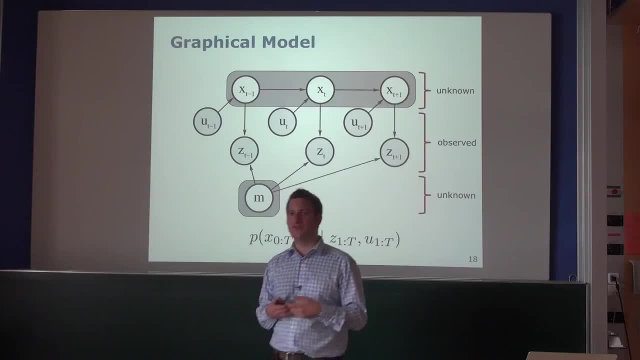 for illustrating dependencies and also assumptions, independence, assumptions that we make, Because if you have an arrow from here to here, it means if you want to estimate the xt, we should take into account those variables which have an arrow pointing to that variable, because it means they are influenced. 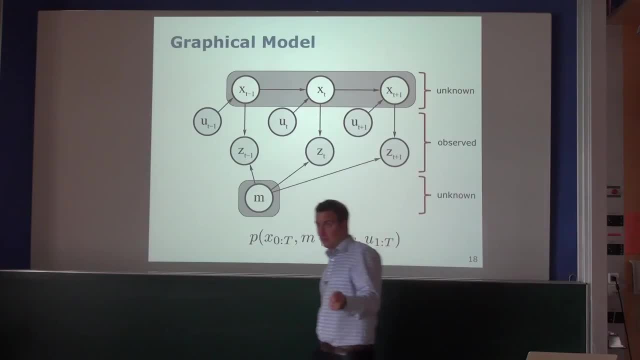 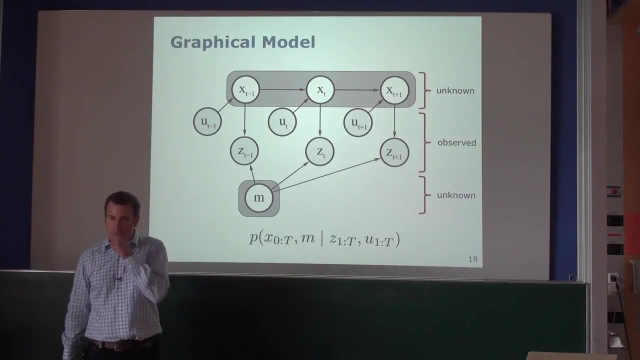 by. so xt is influenced by xt minus one. so if I know xt minus one I get a better estimate of xt And if I kind of drop an arrow somewhere, can quite nicely illustrate modelling assumptions with that, Because I can assume just a model I create. 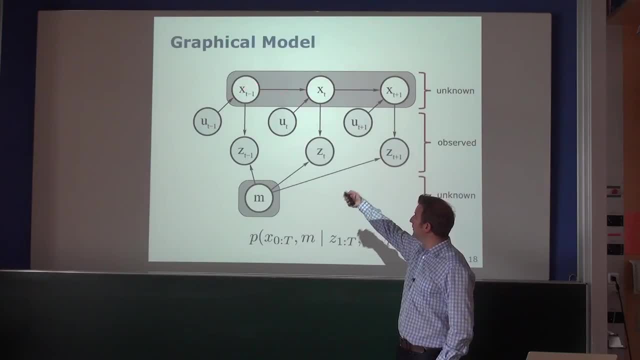 I can assume that the current pose of the robot doesn't depend on the previous pose. That's just my model of the world. If I make this assumption, it's quite likely that my estimate gets worse, But I can do that. and these graphical models? 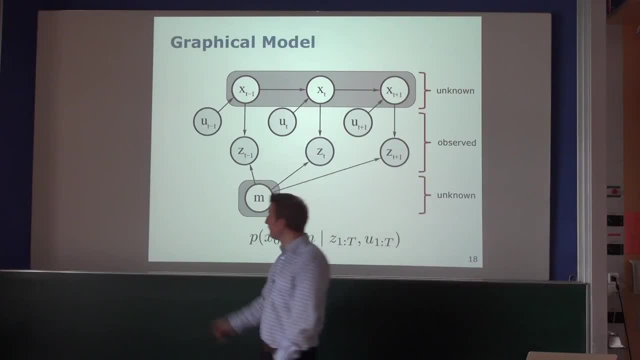 are kind of nice to illustrate those independence assumptions And this is what we call full SLAM. So we want to estimate the full trajectory of the robot and we want to estimate what the environment looks like. Sometimes one is not interested in full SLAM. 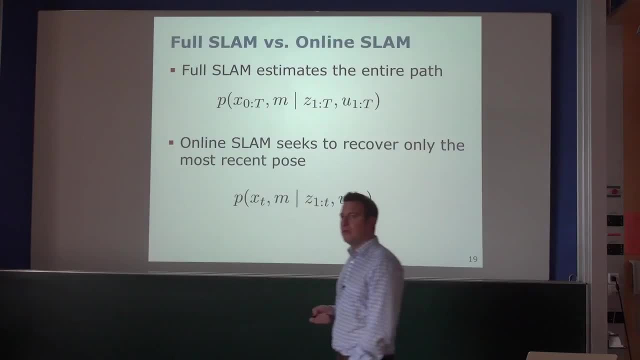 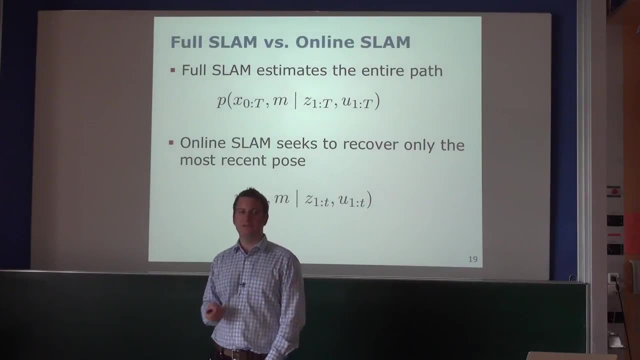 where I estimate the full path of the robot, but I'm interested in what we call online SLAM. I just want to estimate the current pose of the robot and the map built up to the current point in time. That's what is written here as small t. 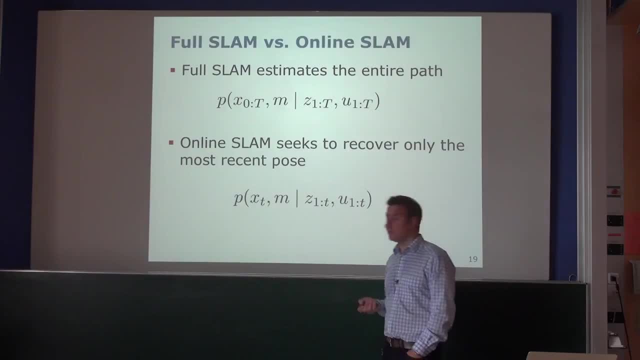 So it's not necessarily the whole sequence. So small t is within zero and large t, So I want to estimate where the robot currently and what does the environment currently look like. given all my previous sensor data, That's actually something that most robots will use. 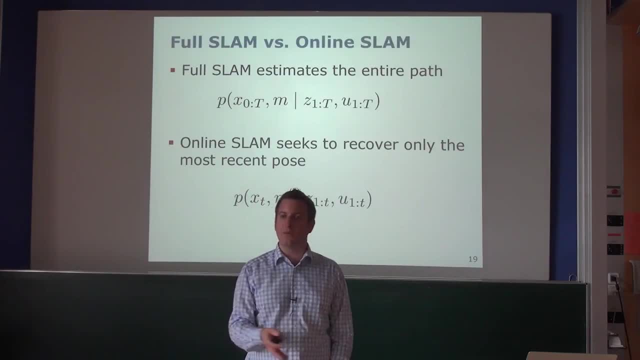 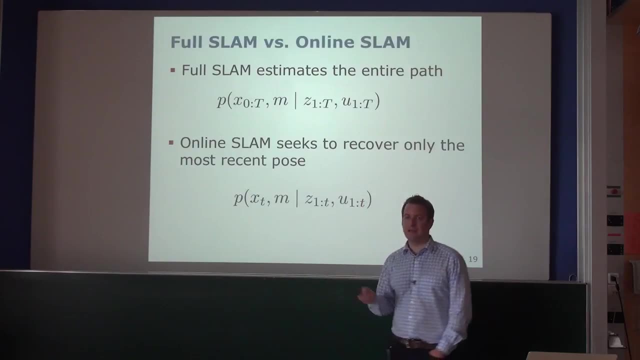 if they want to make decisions based on where they are and where they want to go. If I'm not interested in the past, given I have a map of the environment, I just want to know where I am right now. So for most real-world applications, 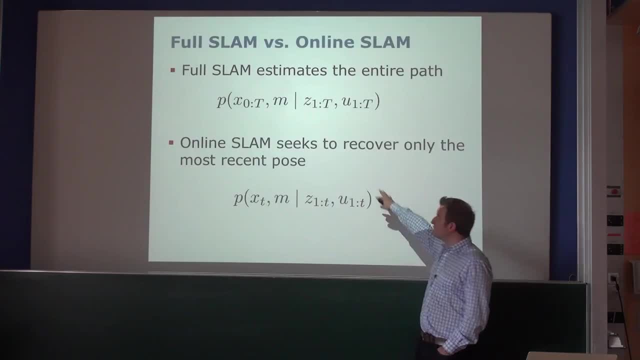 this online SLAM is actually the interesting property. I don't want to collect all the sensor information beforehand and then build a map and estimate where the robot was. I want to do it online right now. If you write that in the graphical model. 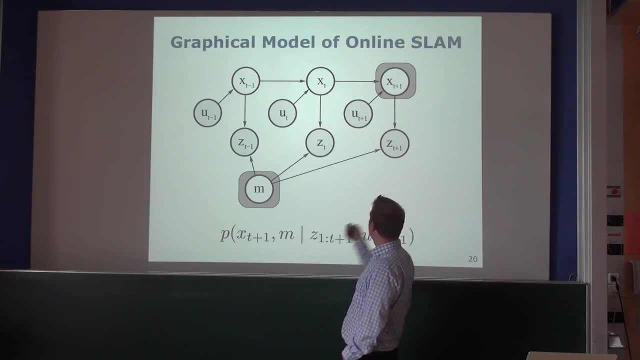 we have exactly the same structure over here, But we typically only have the great area of variables. so those variables that we want to estimate is only the last pose, And the previous ones are not interesting for me anymore From a mathematical point of view. 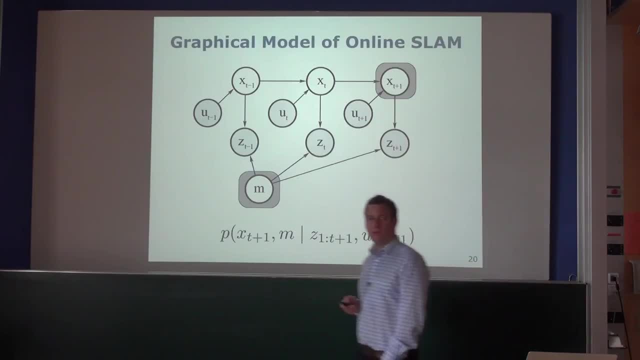 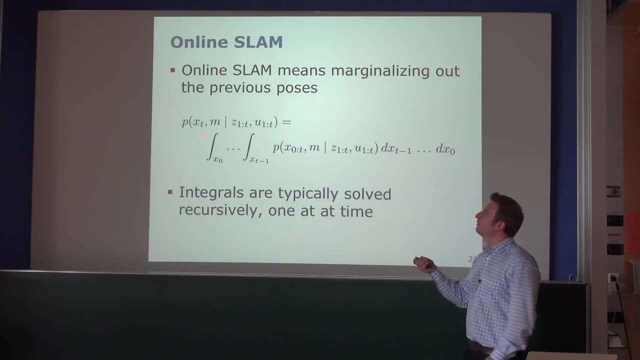 this means we need to integrate out all the previous poses. So if you're only interested in estimating the position at time t and the map of the environment, this is actually an integral over all the possible locations at x zero, all the possible locations at x one, x, two, x, three. 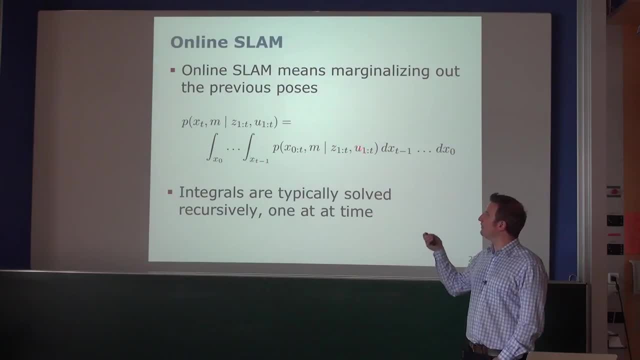 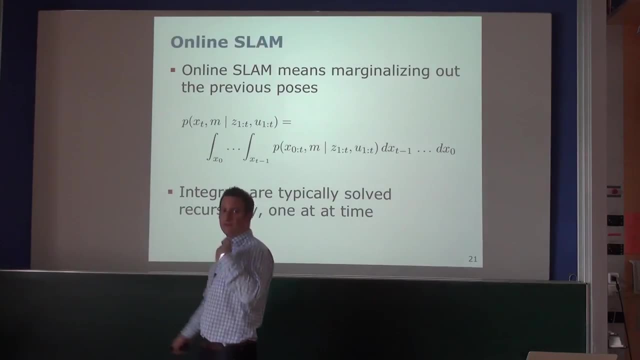 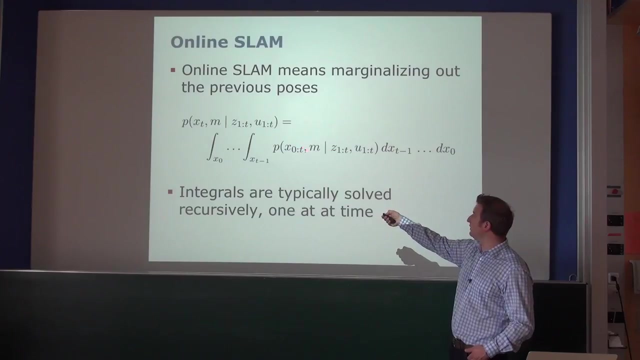 until x t, minus one of the full SLAM posterior Right. If I integrate out the variables, I kind of remove them from my estimate. So this is a full SLAM posterior. Here's x zero to x t. And if I integrate out, 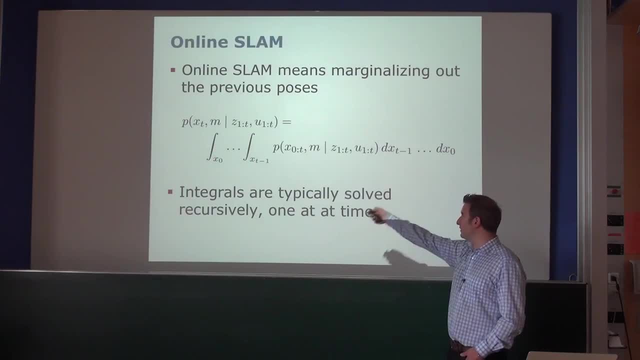 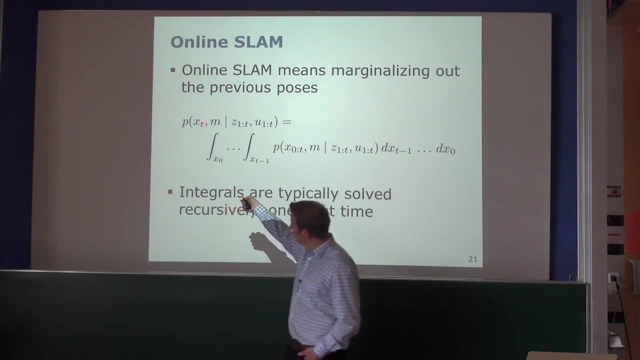 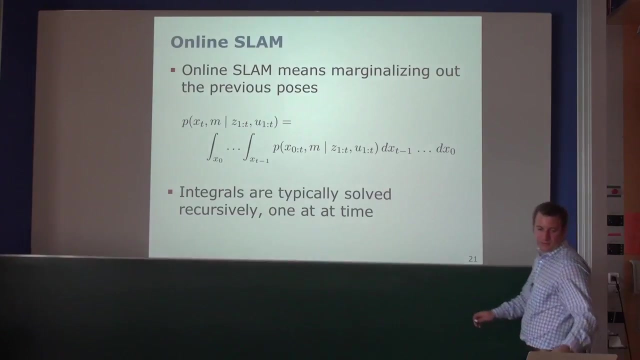 x zero to x t minus one, I actually get the probability distribution which is the variable x t, just the current point in time. This holds for all variables. So if I have a probability, a joint probability distribution, p, a and b, 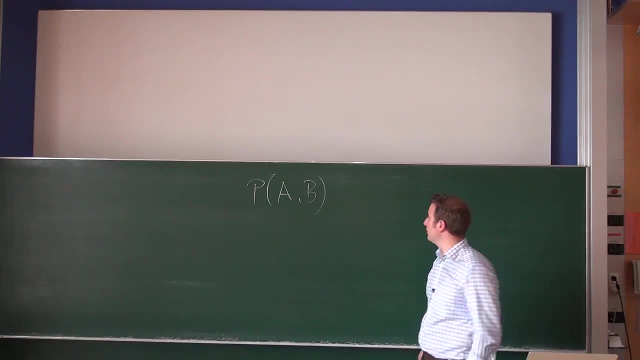 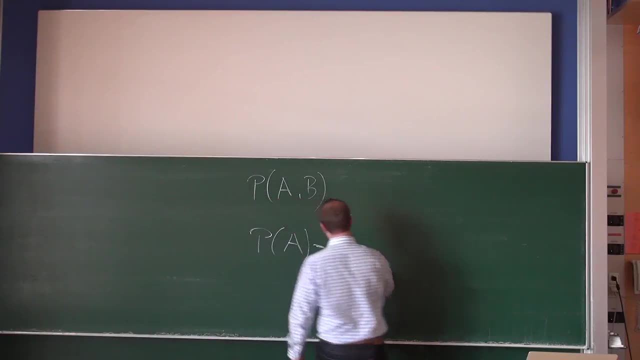 so just two. whatever quantities I want to estimate, I can actually say: p of a is the integral over all possible b's. Let's write it informally: I integrate over all b's of p of a and b, db. And so what remains? 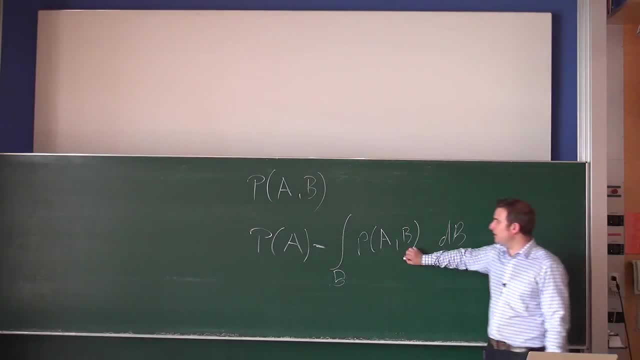 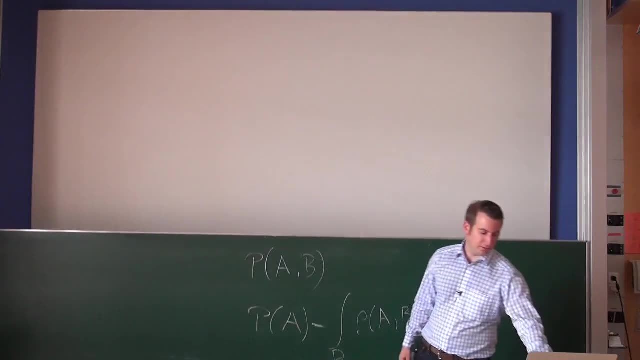 if I integrate over all possible outcomes that b can take, I end up having the probability distribution about a, And this is exactly the same thing I do here. So there's no black magic in there, It's just the integral of all those positions. 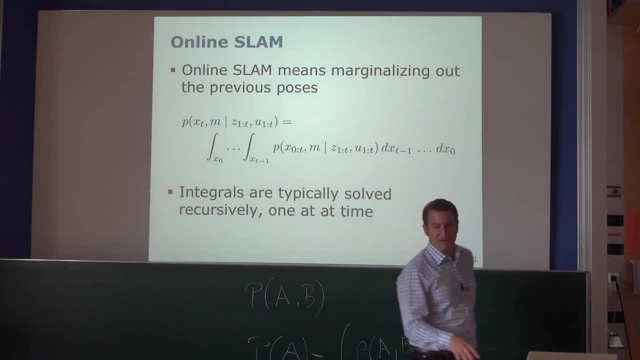 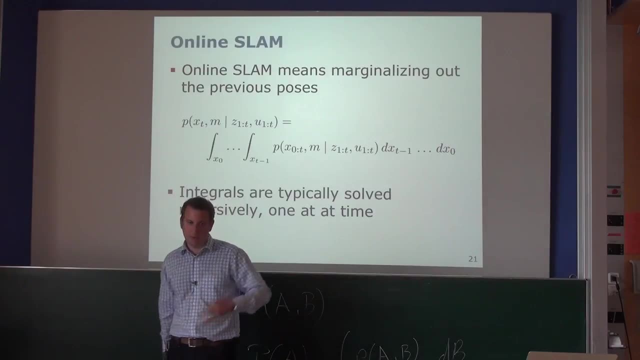 and how these integrals are solved is kind of recursively, one at a time. So if I go from x t, if I go from x zero to x one, I do that estimation step and get rid of x zero And then next point in time. 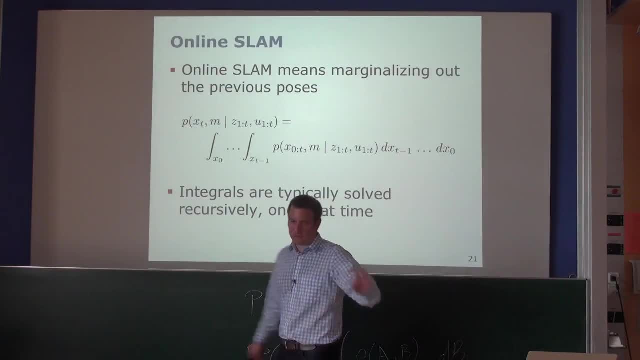 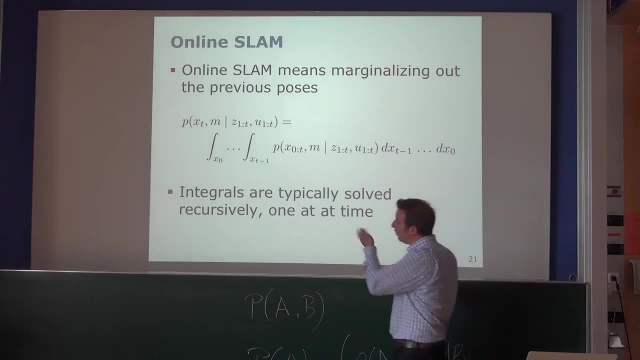 I move, the robot move from x one to x two. It moves from x one to x two and then integrates out x one, Kind of an successive iterative process, while the robot moves through the environment. So at every point in time one of those integrals is solved. 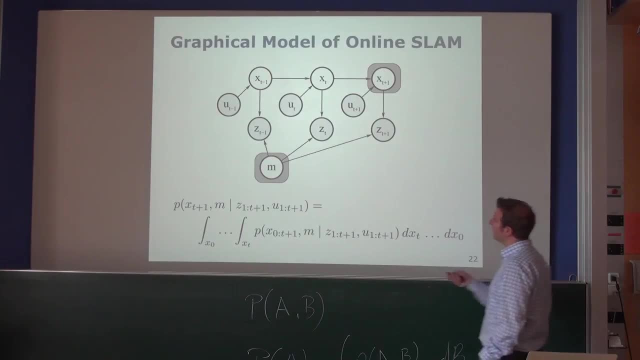 Okay, So that's kind of our graphical model for online SLAM and the corresponding distribution down here And different techniques we will see in this course solve the online SLAM problem or the full SLAM problem or a variant of that, And it just depends. 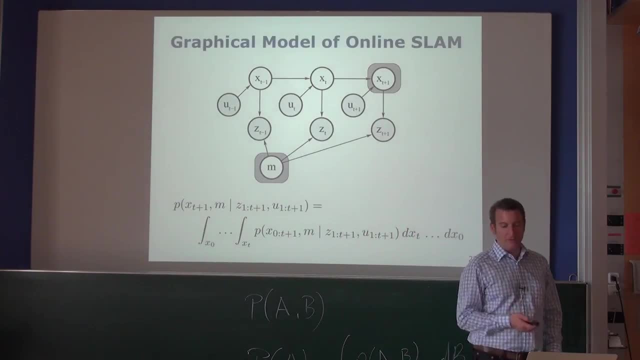 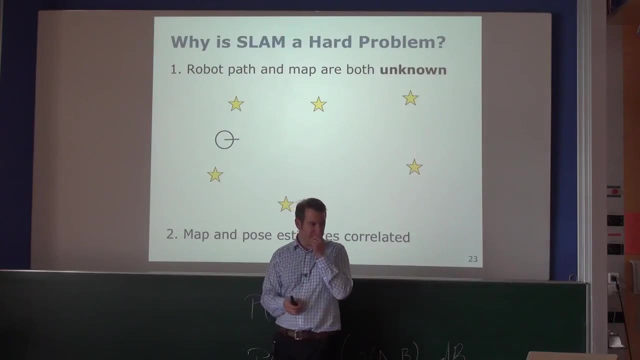 how I model my problem and which technique I'm going to apply to solve that. Okay, So one motivation just to say: why is SLAM actually a difficult problem? The first thing in reality, is what we have is that, the estimate of the path posterior. 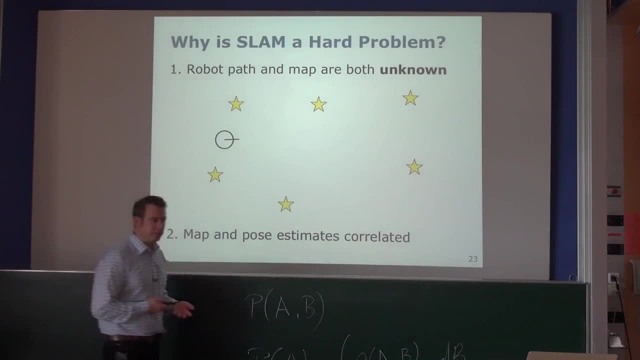 and the estimate of the map posterior. they actually correlated. They're both unknown and they're both correlated. So we don't know the path, We don't know what the environment looks like. We want to estimate both And at the same time. 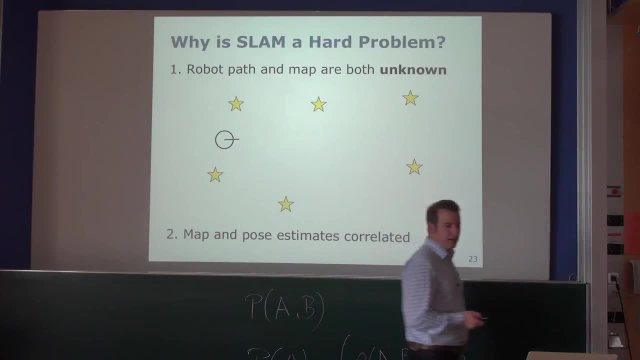 those estimates are correlated, So they depend on each other. So, okay, we have an example here. So that's a robot drive through the environment measures, those two landmarks moves on. So then this circle should represent actually the uncertainty it has about the position of those landmarks. 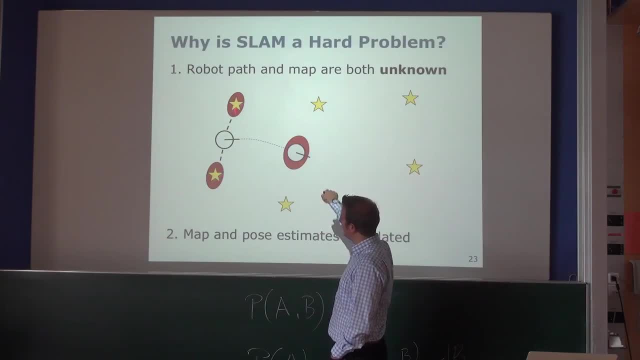 So it doesn't know anything. These are the true locations of those landmarks And so it estimates this guy is over here, this guy sits over there, And then the robot moves on. While it moves on, it ends up being here, but it doesn't really know where it is. 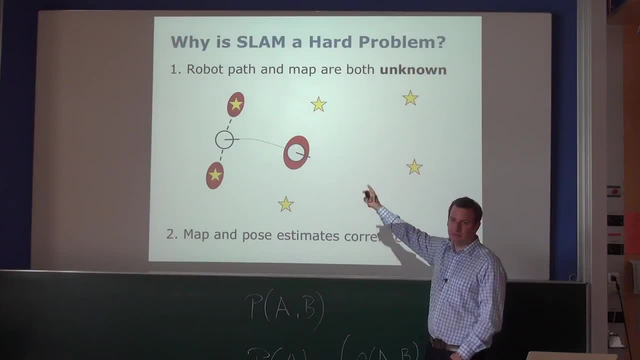 So it has kind of a mean estimate and an uncertainty, for example in here. So you can see that here the uncertainty was basically zero. It just started off the robot. It said, okay, I started, zero, zero, zero. That's the center of my reference frame. 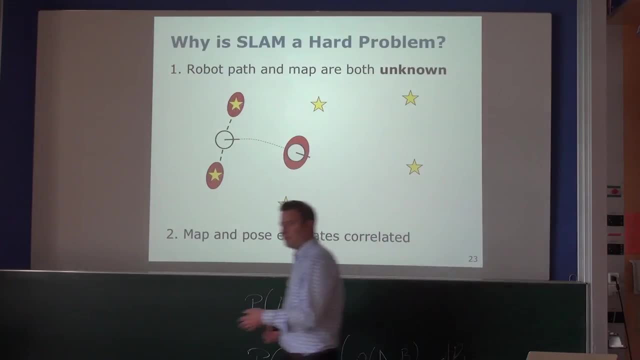 Here I go, Perfectly know where I am. Now I go five meters forward and I don't really know if I went five meters forward. maybe four meter fifty, maybe five meter fifty, maybe a little bit to the right or to the left-hand side. 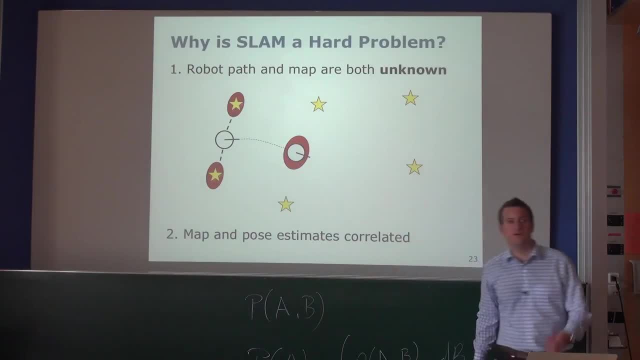 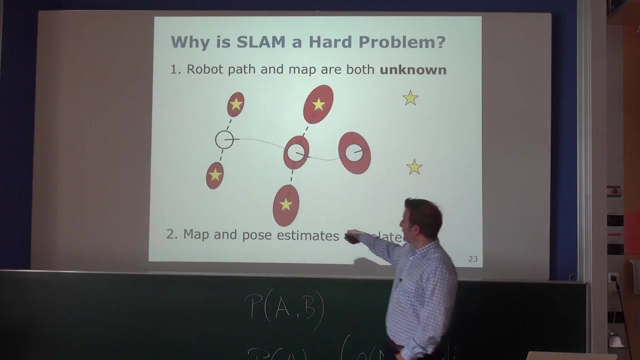 And therefore I have this uncertainty over here. So motion increases the uncertainty of the system. Right, Okay, Okay. Then again, the robot measures these two landmarks And you can see here also we used exactly the same sensor reading Same sensor. 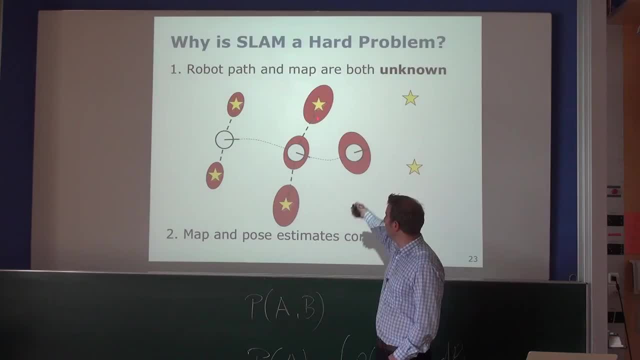 So the uncertainties around this landmark and this landmark should actually be the same than this landmark over here, But the reason why they are bigger is that I need to combine the uncertainty the robot has when it did the observation and the observation uncertainty, And therefore 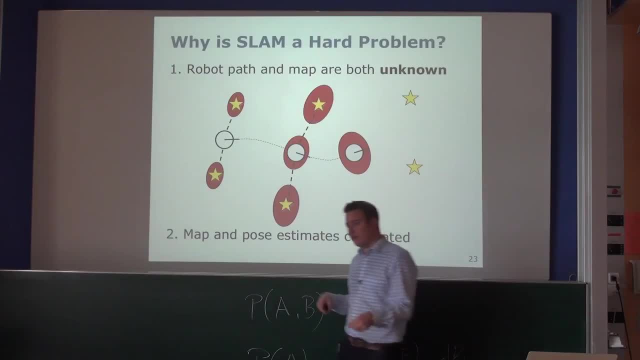 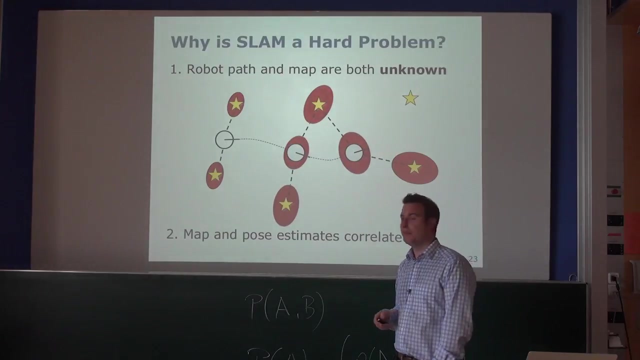 these ellipses are bigger because I still have some uncertainty, because I didn't really know where I was, plus the uncertainty of my sensor reading And the robot again. the robot continues, moves forward and now happens one thing: It actually observes, reobserves the landmark. 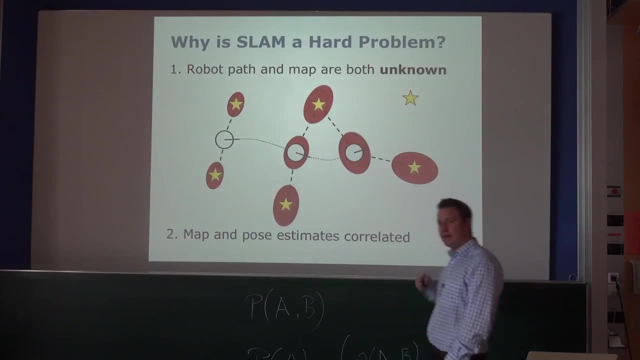 And by reobserving a landmark and say, okay, I get already a better estimate for where I am, because now it has an expectation of what it should measure. given the model, You can say, okay, I measure something else, so I actually can also. 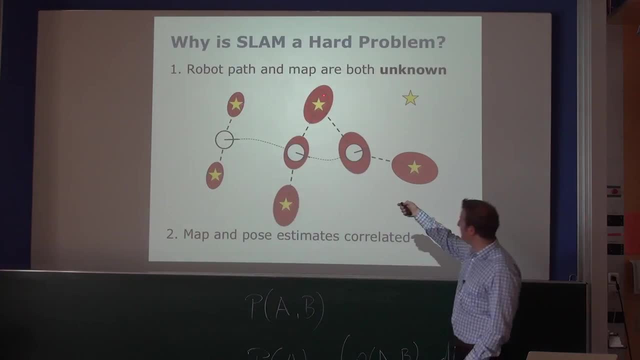 correct the map a little bit, And this is shown by this small black circles over here. So this is the uncertainty ellipse after the next update step, When the robot updates its map because it has reobserved something, So it gains more information. 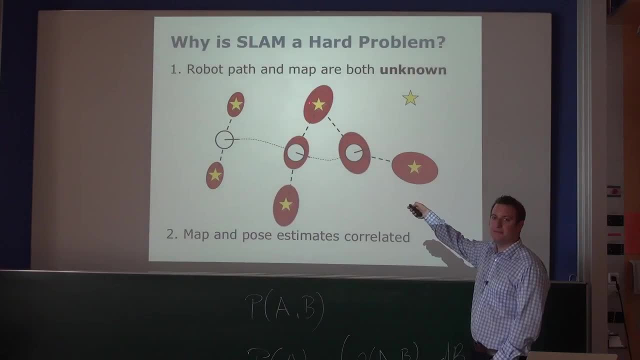 And you can see. also, it was just observing this landmark over here And if it gets more certain about the location of this landmark over here, it will automatically get more certain about where it has been before. Because if I know the position of this guy better, 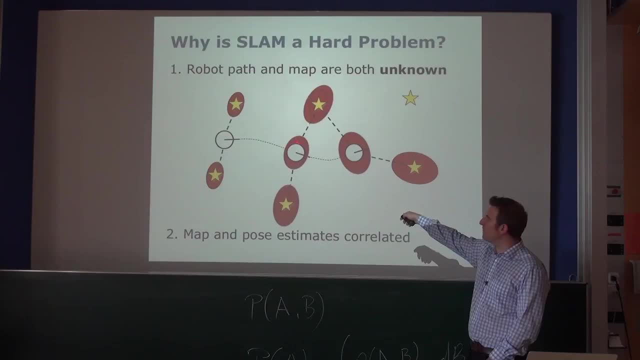 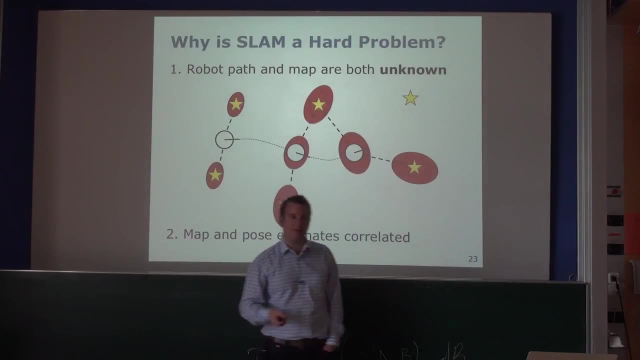 this will also reduce the uncertainty of this estimate, because I made an observation from here to that landmark beforehand And so all the map estimate the position of the landmarks in this case and the estimate about the poses where the robot has been. they are actually correlated. 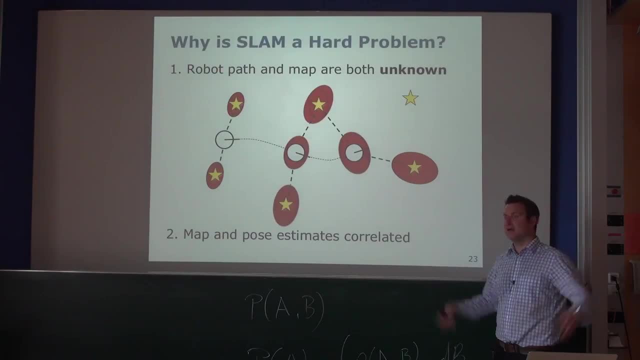 So if I gain information about one part, this impacts all the other, And so, given that dependency, that means I cannot estimate them separately. I cannot say I only estimate the poses and then solve the mapping problem. That's something which typically doesn't work. 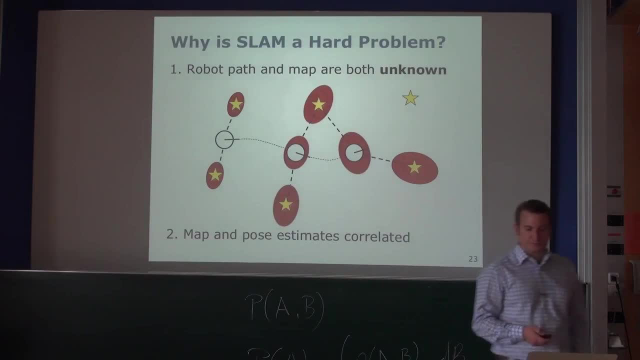 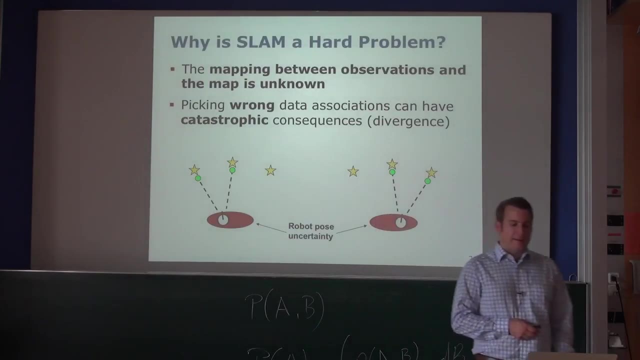 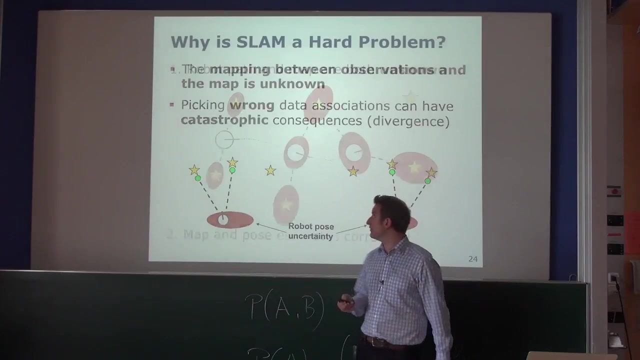 because you neglect the dependencies in here. The second thing why SLAM is a difficult problem is data association. So if the sensor observes something, I need to actually relate what I see to what I've seen before. So, for example, if I go back to this example, 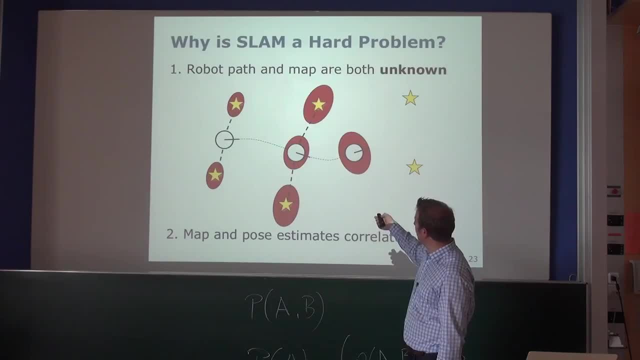 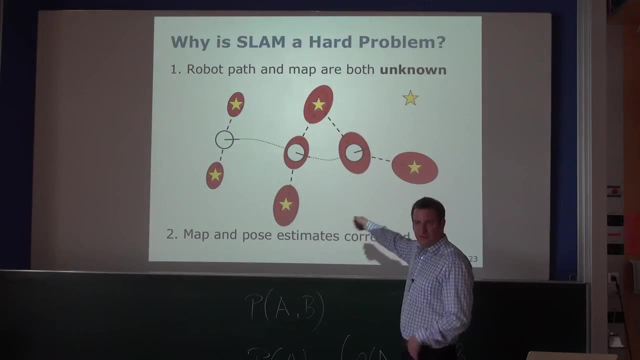 exactly in this situation. so next one here. the robot now makes a new perception and says: okay, what I've seen here is exactly the same landmark I've seen before. In this situation it may be easy because there are not many landmarks. 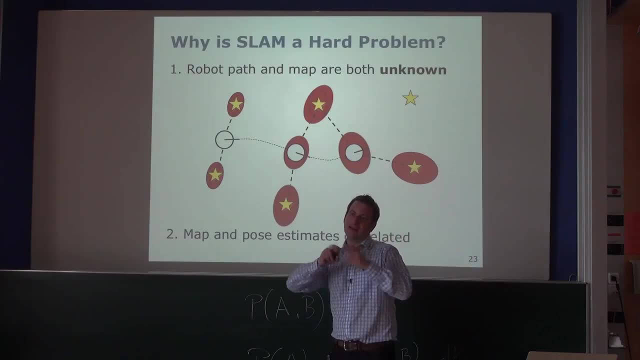 but assume that here are 10 landmarks really close together nearby. It's quite likely that you kind of flipped the association depending on how distinct those landmarks are. If these are all identically looking poles or trees, making data association errors is quite likely. 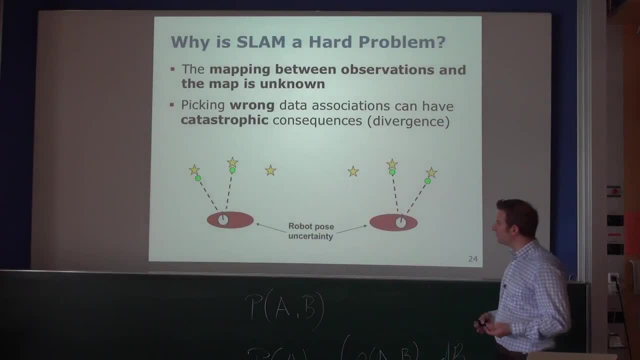 but if they are, let's say, a very good feature description. that may not happen that often, But in practice it happens from time to time that the robot confuses two places for two landmarks, And the other thing is that also the uncertainty. 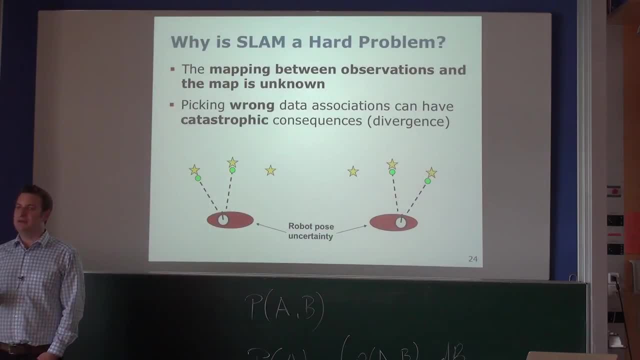 of the pose estimate impacts the data association. So let's say this is my uncertainty at the moment and I get an observation which is kind of: I see these two features, these green dots, So I can either be here sitting here on the left. 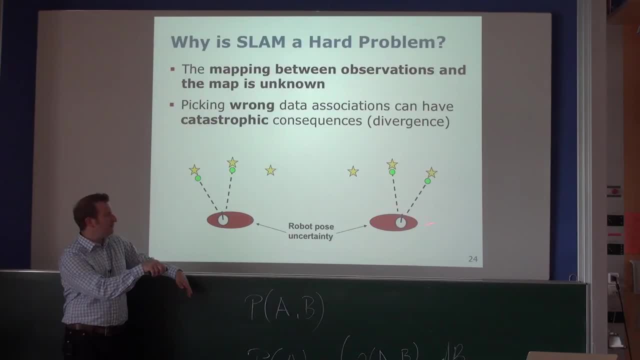 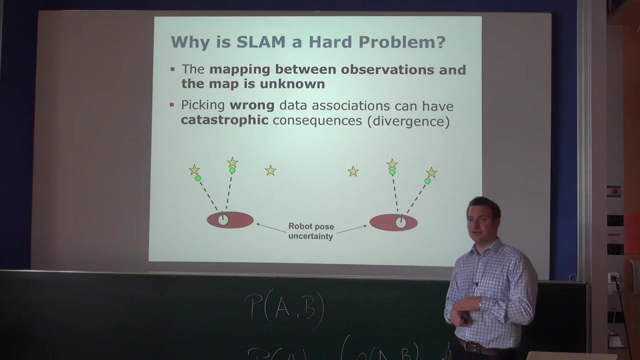 or I can be sitting on the right, And this situation is especially constructed to illustrate that both have exactly the same likelihood. So just because I have motion uncertainty or uncertainty in my current pose estimate, that makes data association harder. And the other thing is that 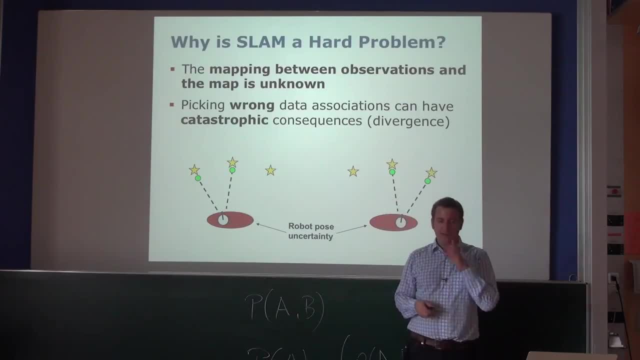 picking the wrong data association here actually leads to a wrong estimate, Because if I say, okay, this is the right data association, so I know I can't be here, so this uncertainty will get smaller and the mean will shift towards this position. 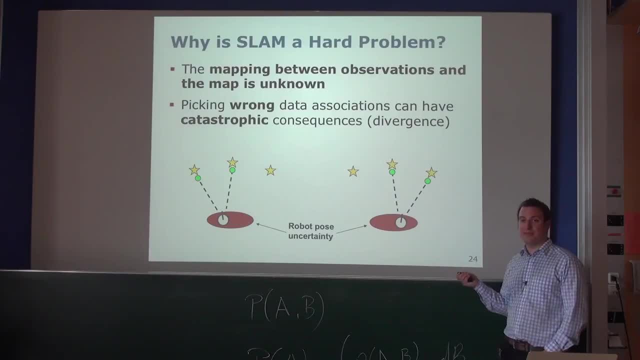 If I, on the other hand, say this was the right thing, then the position of the robot moves more to the right-hand side over here, And so then I get this observation, if I assume that this observation is right. And so in this situation, 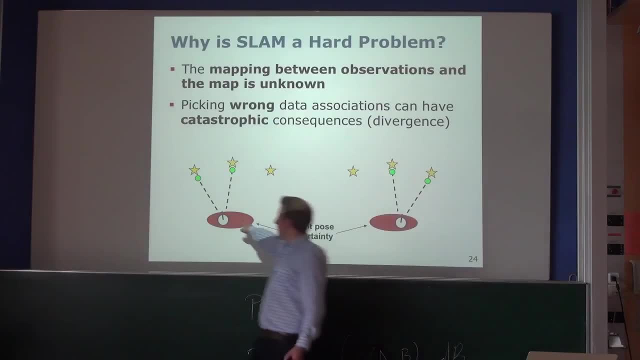 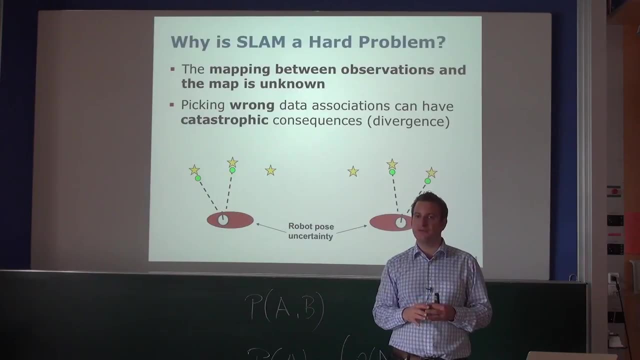 this would be the uncertainty of the robot, probably, And in this situation that would be the uncertainty of the robot. And so the uncertainty gets smaller, And if I did the wrong association, I get a wrong estimate of my uncertainty, And that's something. 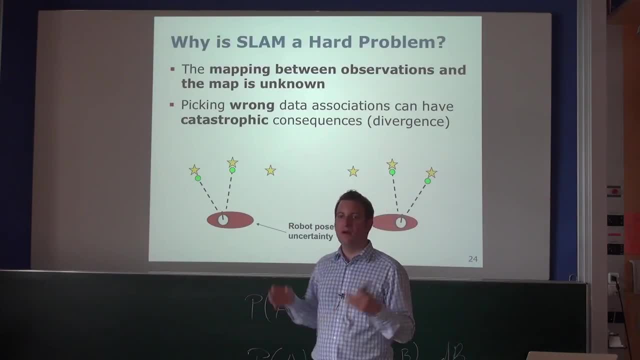 I don't want, Because I can't get typically get overly confident of where I am, which is- and this is something which is not true, So I get an inconsistent estimate. That's the kind of reasons why SLAM is a non-trivial problem. 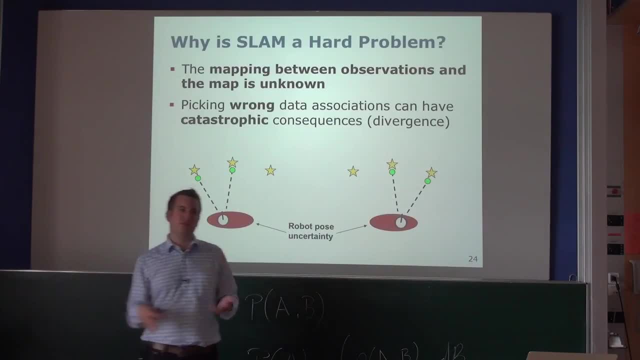 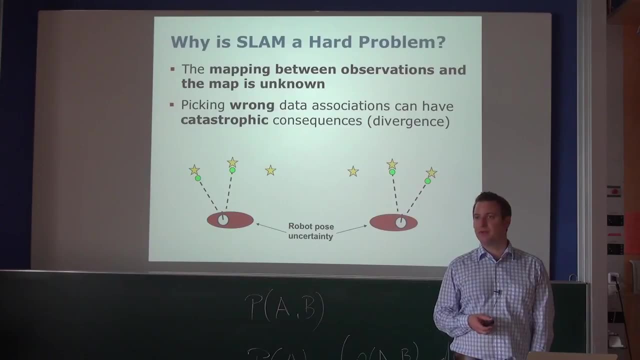 I have these dependencies between those variables and I also have these data association errors. These are two things why it is still a tricky problem At that point in time. are there any questions? Okay, So then we would like to go quickly through. 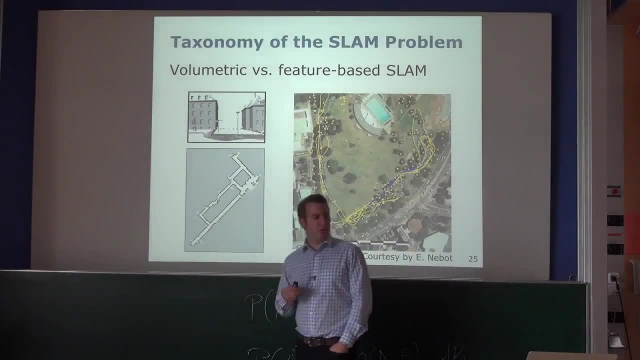 a typical taxonomy of SLAM algorithms. So how can you describe different SLAM algorithms? What makes it distinct? The first thing is on kind of. what kind of maps do they estimate? We have one class of approaches which generates volumetric representations. 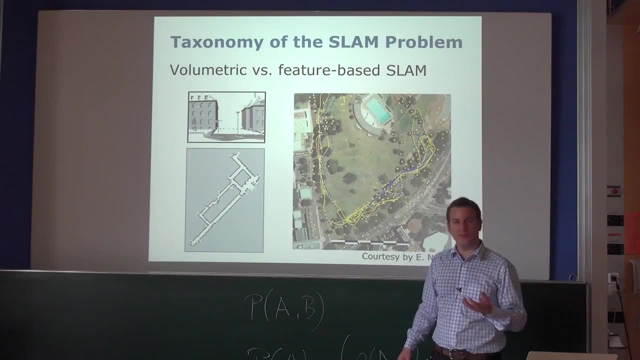 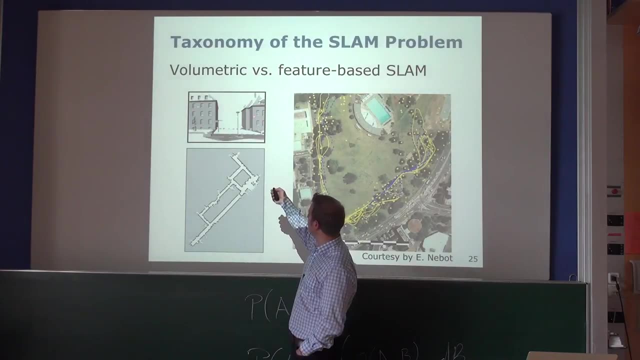 So like, for example, if you see this over here, that's actually building 52, that's actually building 50, that's actually building 50, that's actually building 52 and 51 on our campus, built with a robot. 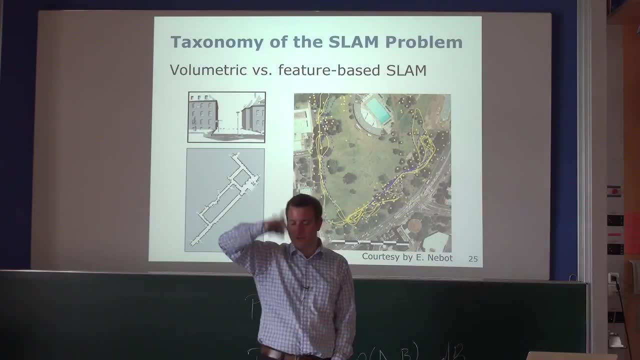 which was standing here having a Pentel laser scanner and building a map of the environment. So I get really this physical structure of all the surfaces, of all the points that I can observe. Or there's also something you will see quite often in this course. 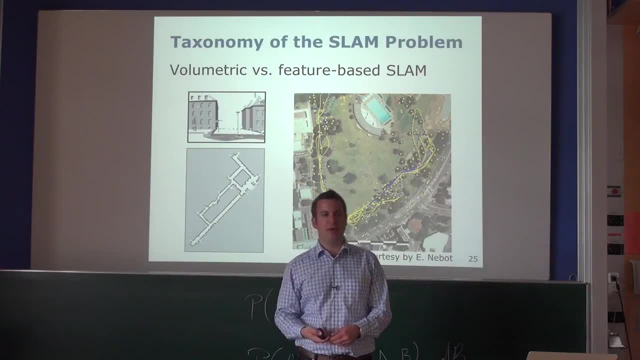 This is a typical 2D map. White means free space, black means occupied space and grey means I don't know. the robot has never seen that part, So this is like an architectural floor plan, but just adding all the stuff which lies around. 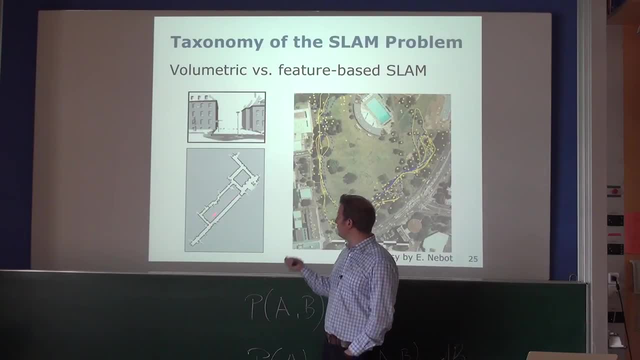 in the apartment or in the building, And so this is also a volumetric representation in 2D. So you have the free space over here and you have the black points, which are obstacle locations. In contrast to that, you may have feature-based approaches. 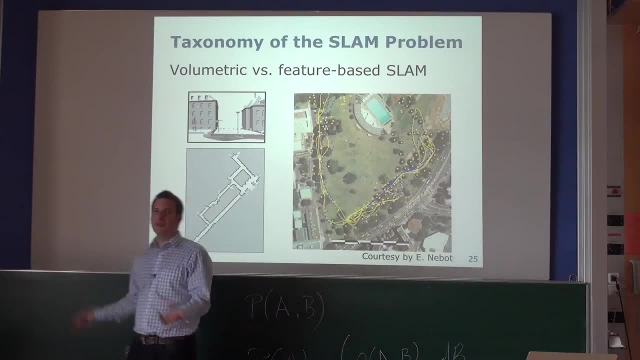 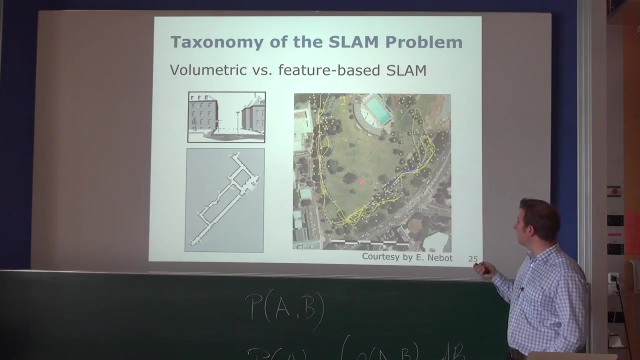 which do not attempt to model all the objects in the environment, but they just want to represent distinct landmarks. This example here, this is the Victoria Park at University of Sydney in Australia, And this is one of the very famous data sets they recorded a lot of time ago. 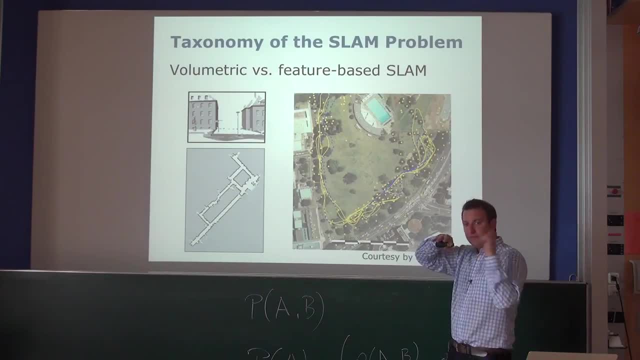 And they had trees over here and they had a laser scanner and was just estimating circular things. It was assumed to be the trunk of the tree and every tree trunk created a feature. So just drive around and just want to estimate the position of those features. 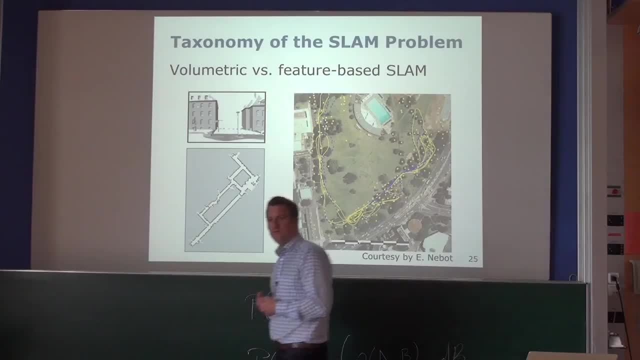 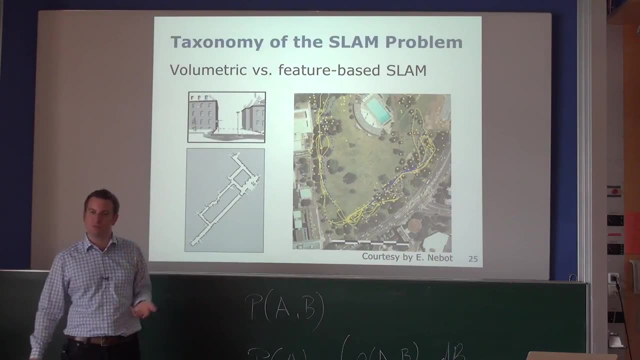 If you know where all the trees are, you can even localise the robot with this feature-based approach. The advantage of this feature-based approach is that it's typically a very compact representation. It's really nice from a robotics perspective, On the other hand. 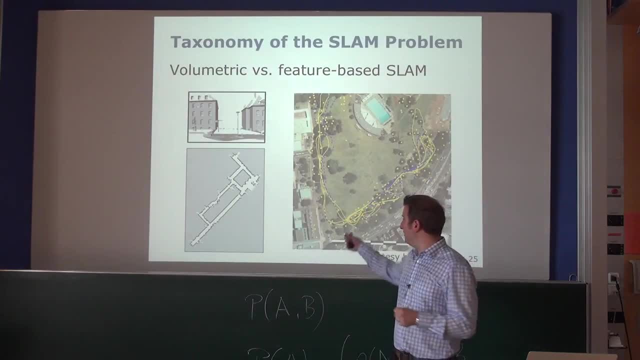 it requires to have means to say this feature. I see, here is exactly this tree there Which is often hard to do, Depending on your feature, depending on your sensor. it may be hard to do And these are kind of the disadvantages of those feature-based approaches. 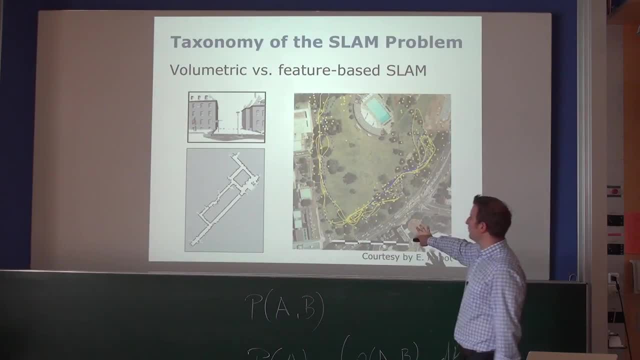 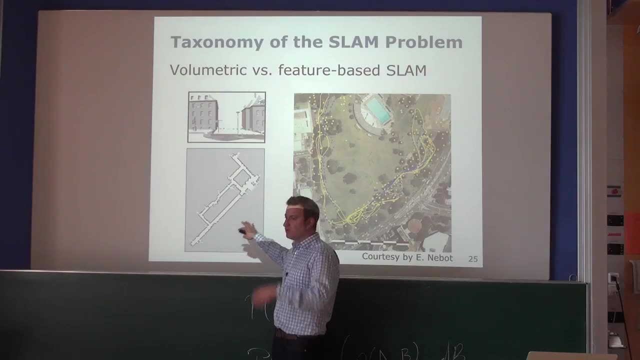 There's always a pro and a con for both sides. If you are happy on localising, you just want to. you have some distinct landmarks. feature-based is a nice approach If you don't know or you really want all the obstacles in the environment. 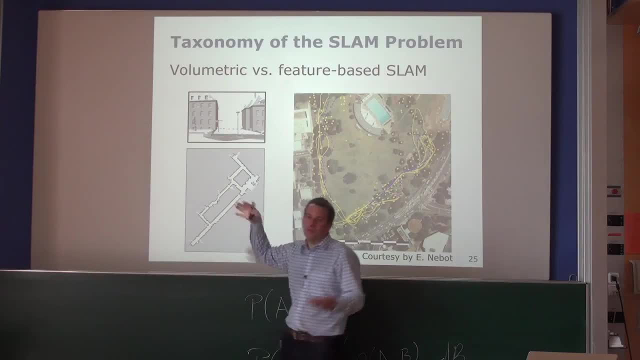 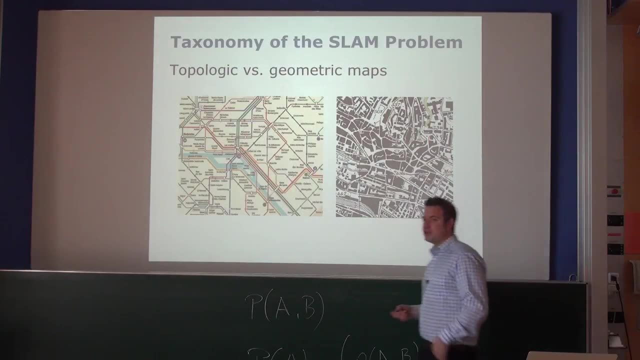 because you want to navigate with that and you need to do obstacle avoidance. this approach may be better Depends on your application, on your estimation technique. The second thing that people often differentiate are topological approaches versus geometric approaches. In one situation you try to estimate. 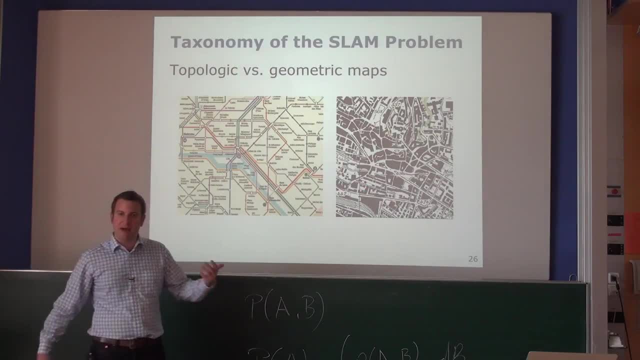 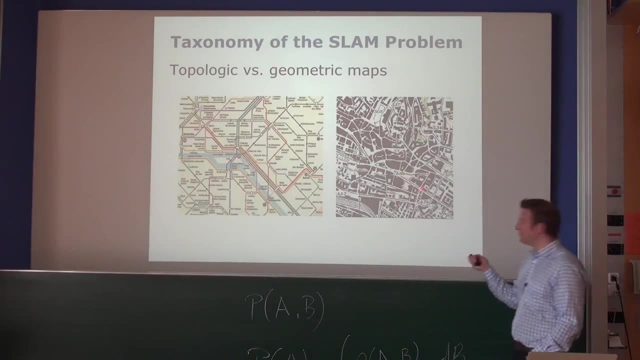 really the geometry. So this is kind of a typical map you can buy or get somewhere. So these are the streets. It's not Google Maps, It's kind of the old-style maps that look like that. I've never seen them. So these were the streets. 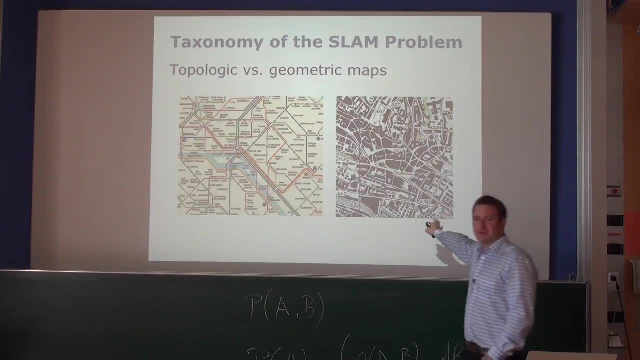 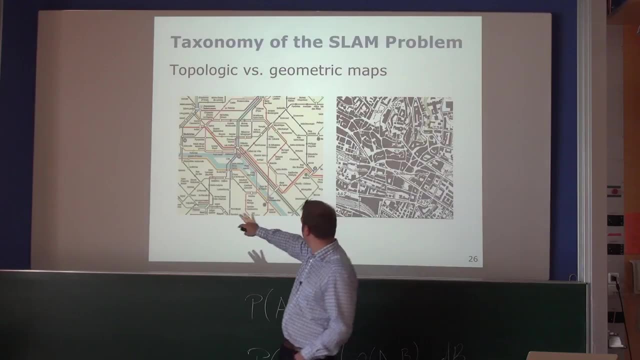 These were the buildings. So this is typical geometrical representation of the environment. What you see here is a subway map, and of Paris, I guess, Yeah, Paris. And what you see here only are the connections between places And even the position. 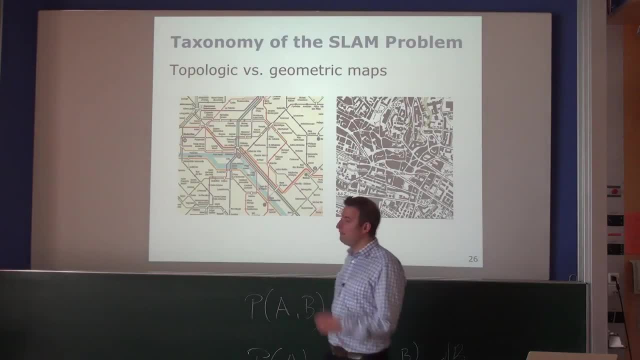 of those places may be not exactly at their geometric locations or the distance between those two places may be dramatically different than the distance between those two places. This just describes you. how do I get from A to B using the subway And for solving subway navigation: 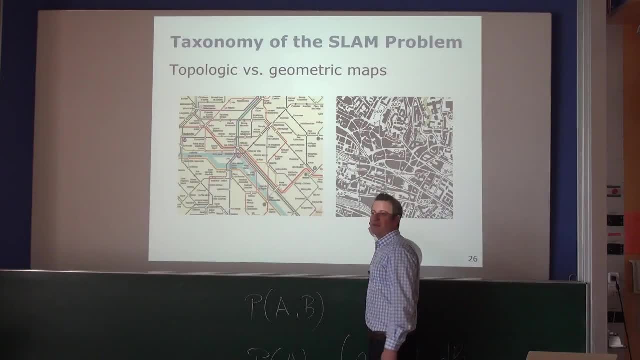 that's much more convenient than representing the subway in a geometrical way, because you don't care whether the subway train goes exactly just one node. if I board whatever train- number eight- I get to that station. So, depending on the application you're trying to solve, 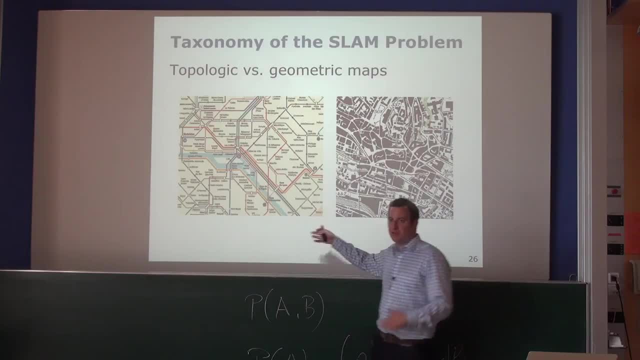 topological representations may be better than geometric representations, as well as the other way around. Again, topological maps are very compact. You can describe them in a nice graph. You can use standard planning algorithms, like A star, which operate on graphs. So using these, 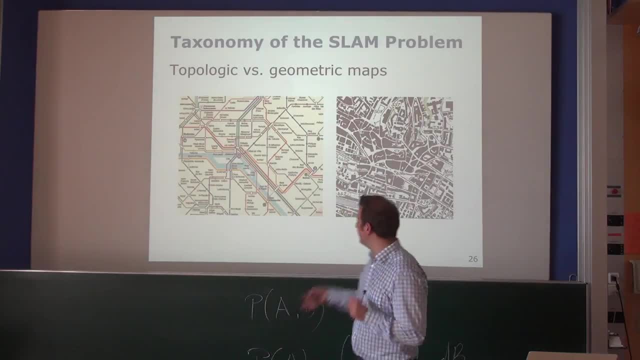 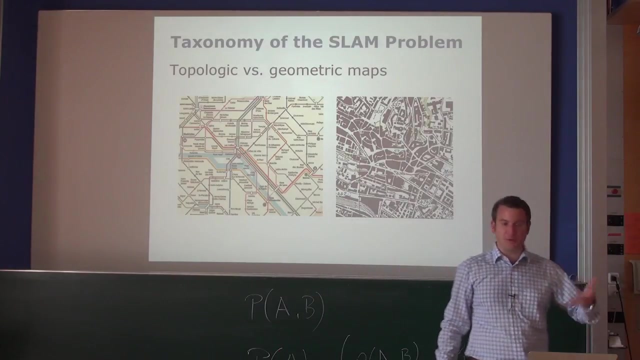 topological representations can be advantageous. Nevertheless, most approaches use geometric approaches, So topological approaches were pretty popular 10 years ago, something like that. There are some people who try to again reestablish topological approaches as some nice properties. They have some nice. 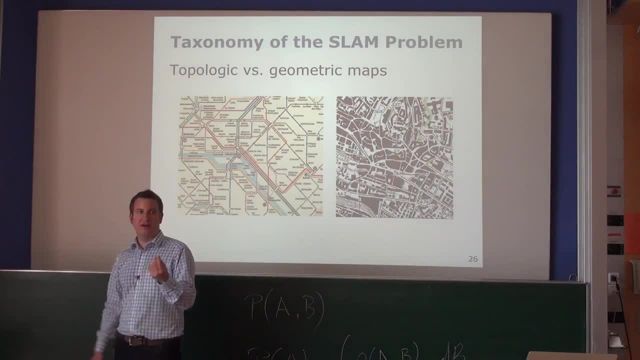 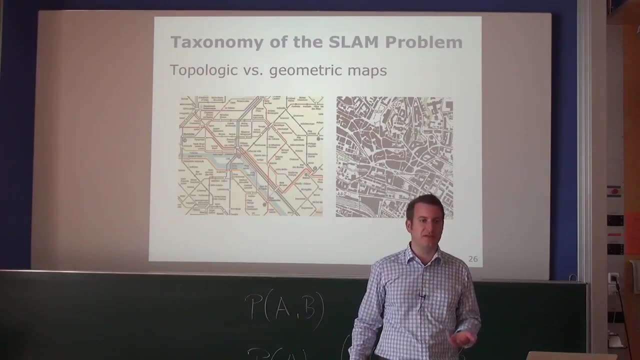 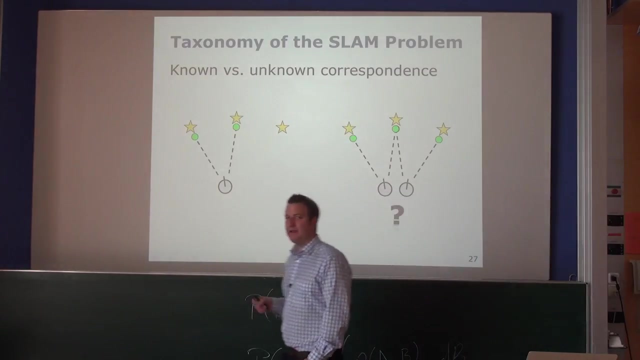 properties. I want to say the difference here. something else here, But for most robotic applications, geometric models are the models that are chosen and that people use. Other things is known versus unknown correspondences. So does a SLAM algorithm that I develop seem to have. 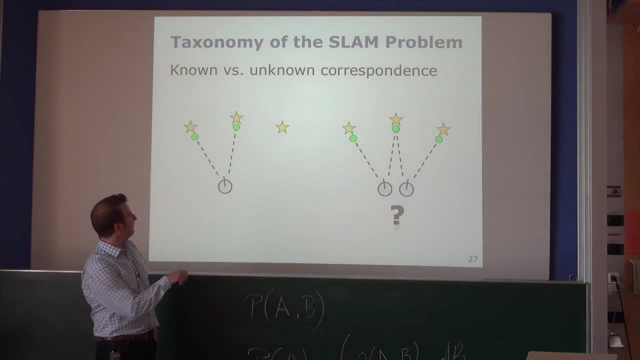 perfect data association. That was the example we had before. So, if I get this observation, do I know that these two landmarks or do I have simply no idea Some approaches make, or most approaches actually assume to have perfect data association? You see a feature. 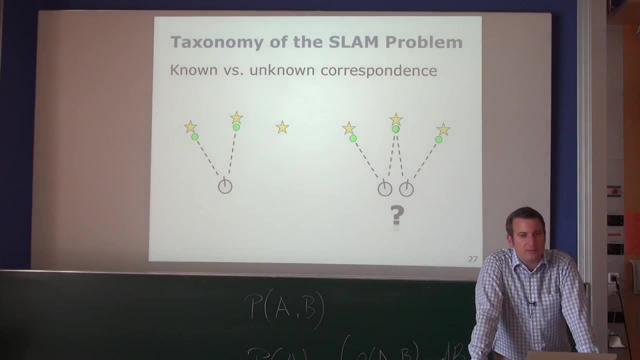 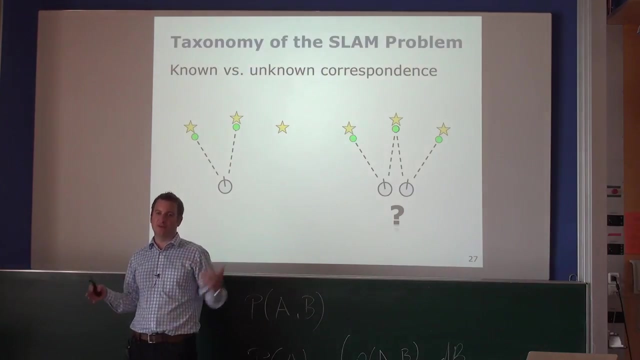 you know which feature it is. It's unrealistic, But it's pretty hard to track all possible data associations. There's a number of possible data. association explodes quite quickly. There are, however, approaches that say, okay, I assume to have a certain number of outliers. 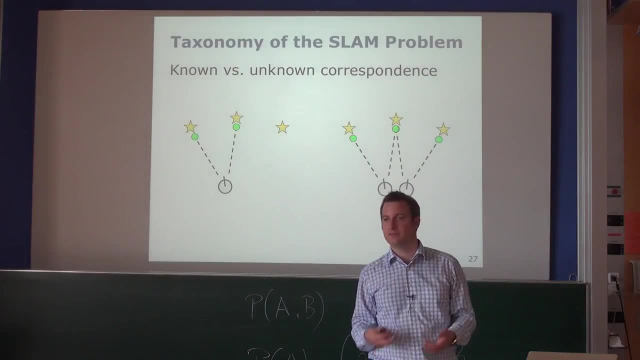 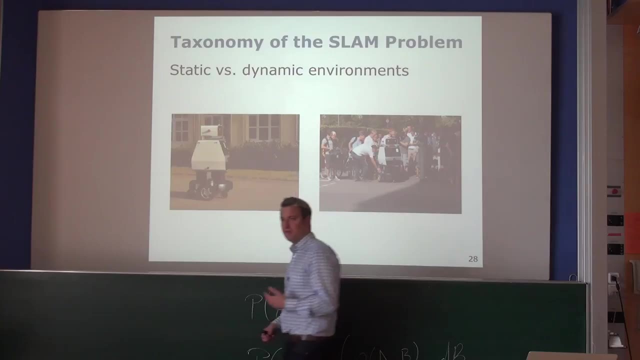 or wrong data associations in my incoming data and I try to deal with that. So it's just something you can differentiate. The other thing is what you often find is static versus dynamic environments. Is the environment not changing? Is it the same? Say this: 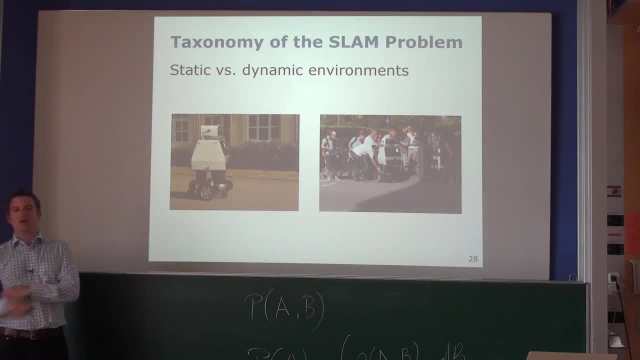 Our robot driving over campus, No one around. The plans are growing over time, but we can say that's a very, very small change. I ignore that, But if you're driving with people in your surrounding and the scene looks like this, it's highly dynamic. 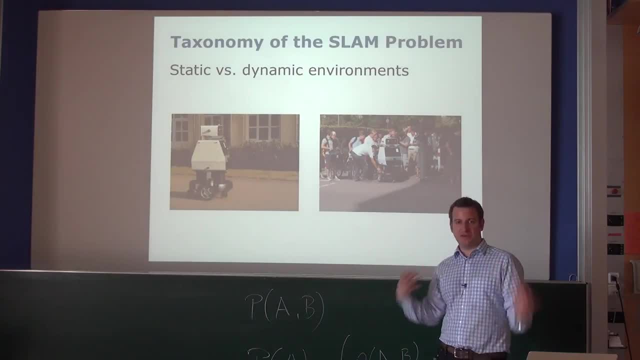 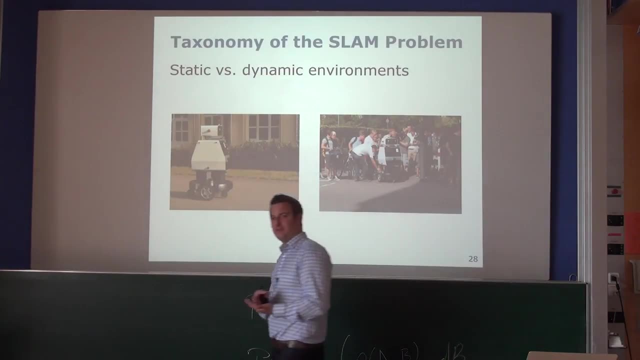 Things change, It's partially hard to recognize just because there are so many dynamic obstacles around. So there are approaches which explicitly say we want to get rid of the static world assumption and really want to allow to model dynamics or changing worlds, and that's a much more. 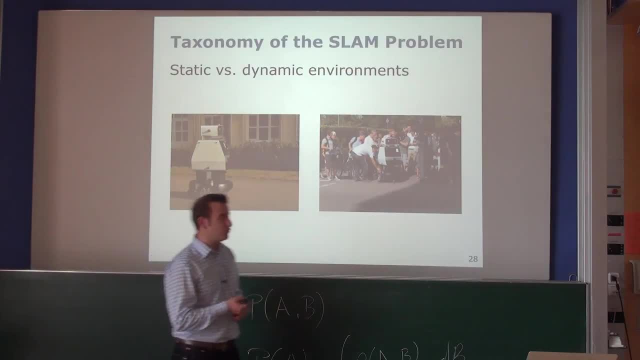 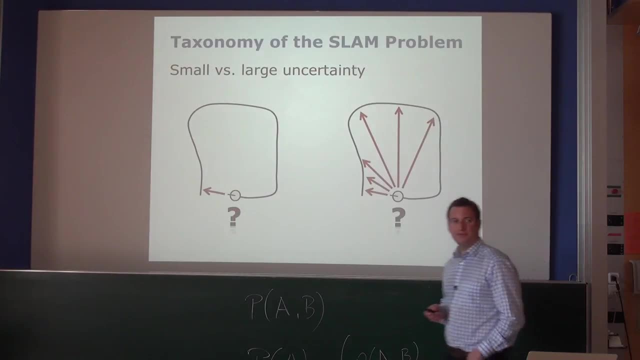 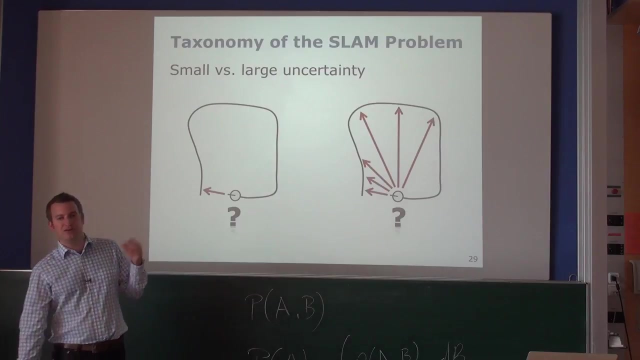 challenging problem than making the static world assumption which most approaches do. What can also differentiate approaches is the ability to represent uncertainty. Sometimes approaches- at least the way they are used- assume to have a small uncertainty in the pose estimate, So it cannot handle dramatic errors. 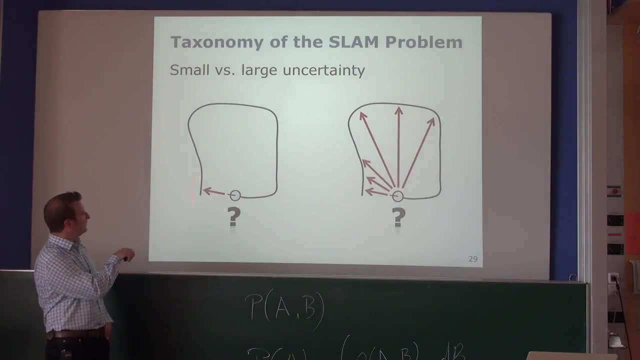 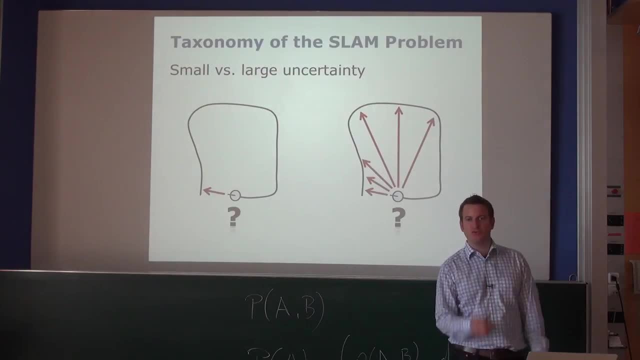 or the way the uncertainty is represented. For example, if I have a Gaussian distribution, I can simply increase my variance and I get a bigger uncertainty without making the representation itself more complex. If you use other ways of representing uncertainty, like sample based representations, you may need 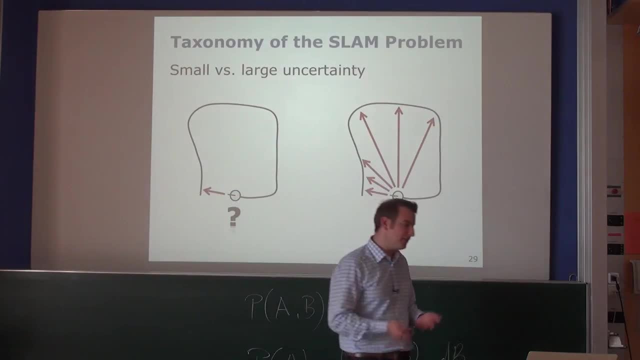 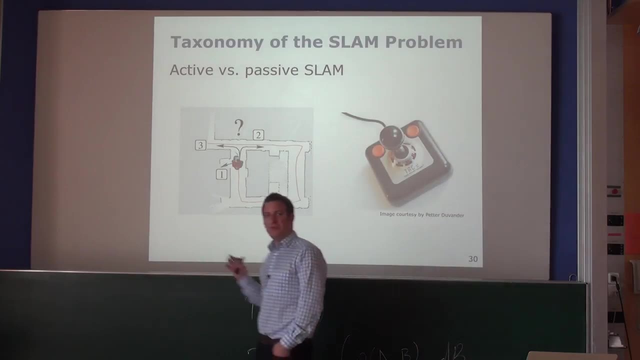 much more samples to actually represent uncertainty better. So that's kind of a difference. What also distinguishes approaches is active versus passive SLAM. So we will look mainly into passive SLAM here. That means we assume the robot is controlled by someone else. 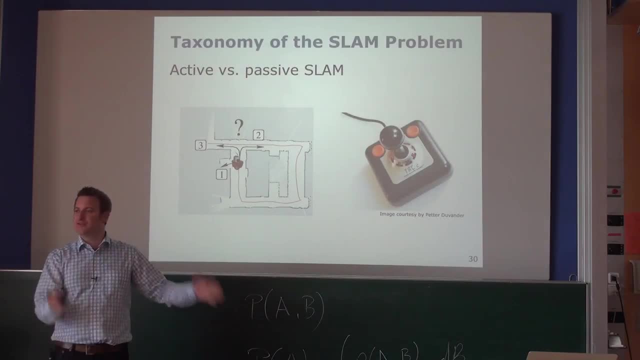 by some person, by some algorithm, We don't care. We just say here the incoming data stream and we work on that incoming data stream. That's standard SLAM, which is passive, However, approaches towards active SLAM, where the robot should make its own decisions. 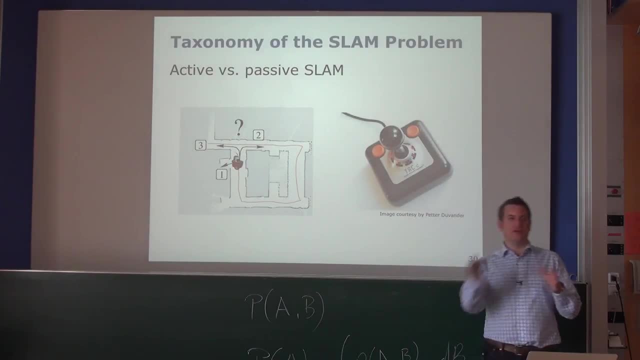 of where to go in order to build a good map of the environment. that, then, kind of involves also exploration. The robot should explore the environment or should decide where to go to get better maps. That's also sometimes referred to as active SLAM. We will mainly look. 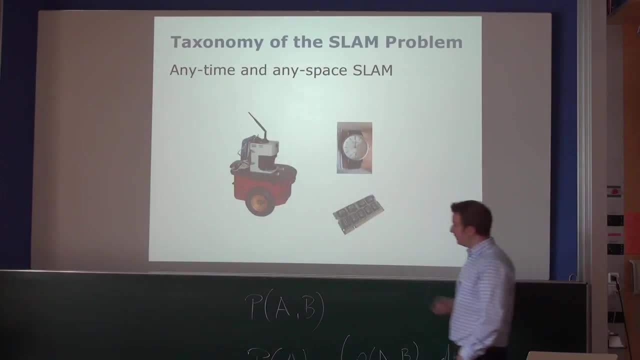 into passive SLAM so you can assume that someone drives the robot around with a joystick. The next thing we see is sometimes any time available, let's say whatever 20 milliseconds per observation that I'm allowed to spend on my estimation system. I don't have. 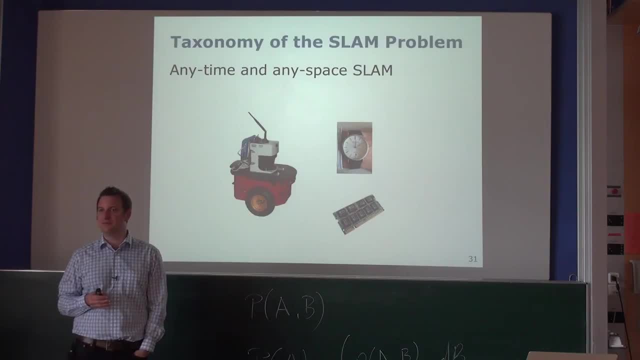 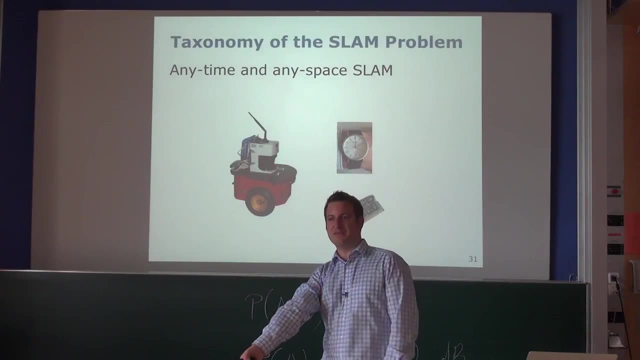 more resources. Do the best you can with this 20 milliseconds, Or say okay. the robot has only one kilobyte of RAM which it can donate to its map estimate, So this is not sufficient to represent the whole environment. What should the robot forget? 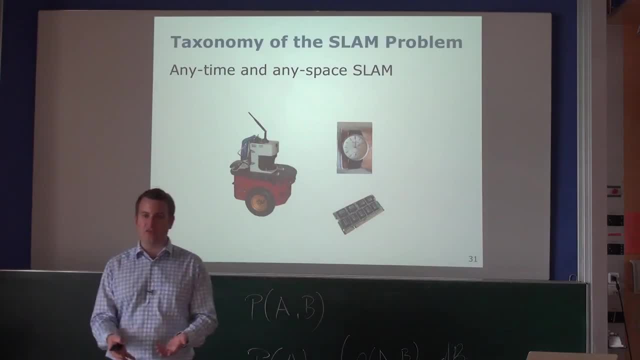 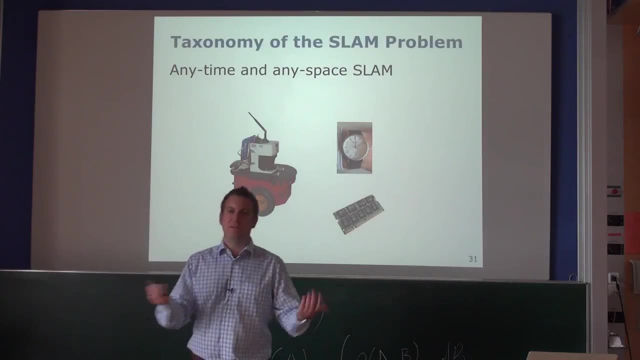 and what should the robot focus on? And if I increase its memory, how does it change? So the more time I have, the better, but what can I do with a certain amount of computational resources or certain amount of memory? That's also something you often find. 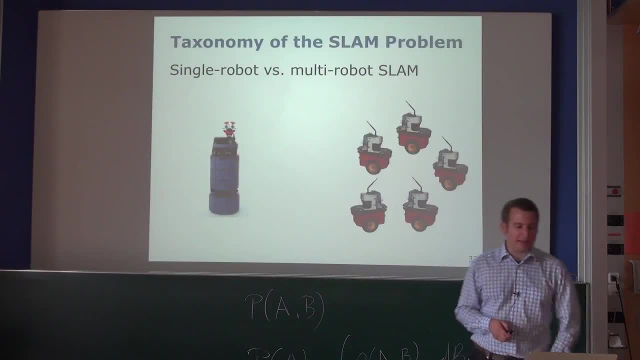 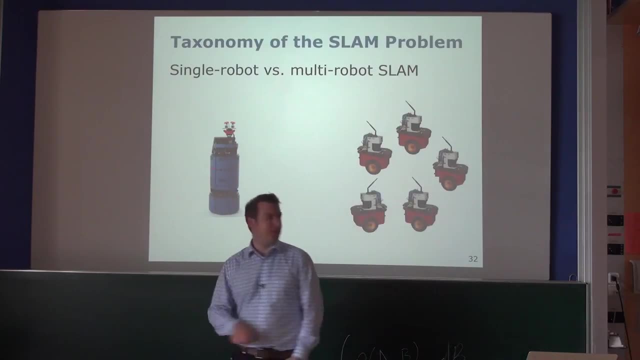 And then you have kind of single robot systems versus multi robot systems. So if you have a single robot which does SLAM or if you have multiple robots- because if you have multiple robots then you need to also make data stations among the platforms- It can be more tricky. 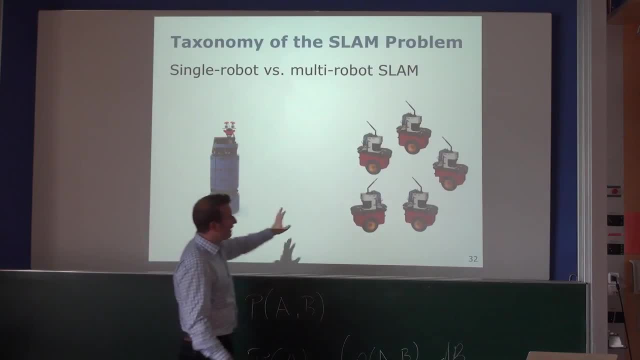 but with more modern approaches. with these graph based approaches, this problem is actually not that dramatic anymore, So it can be integrated nicely into the same framework and doesn't require some extra handling as it was the case before. So you don't find this distinction, single robot. 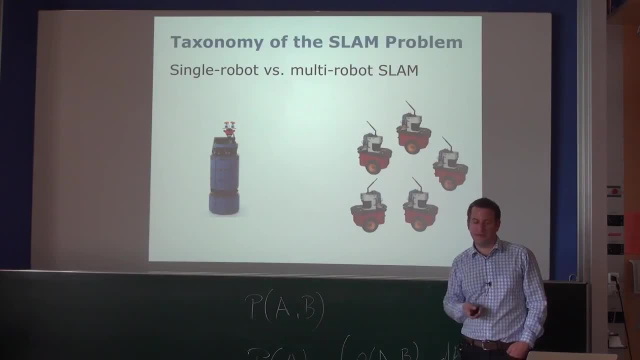 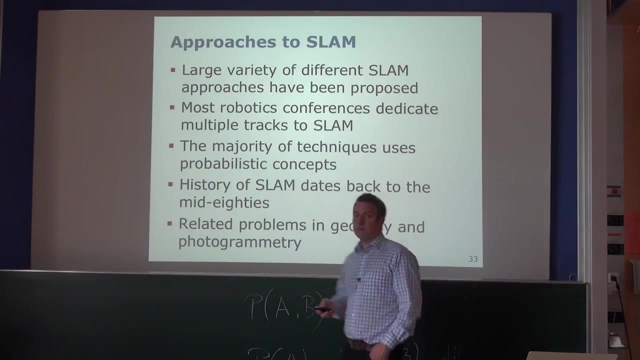 multi robot SLAM that often anymore, as it was done, let's say, five to ten years ago. Okay, so we have a large number of different properties of the SLAM algorithm, of those SLAM systems or requirements that we need to address, and there are a large number. 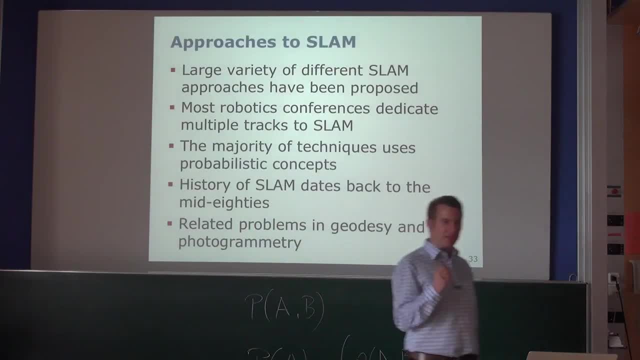 of different algorithms that we can use to solve the SLAM problem. They all have certain advantages in certain settings. under a certain assumption, this is the optimal approach, or under other assumptions, this is the best approximation that I can do where I can compute in a certain amount of time. 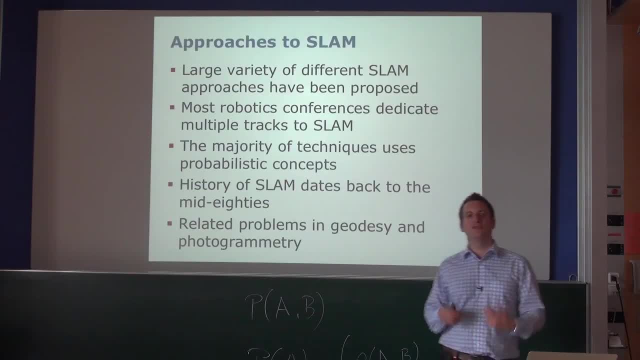 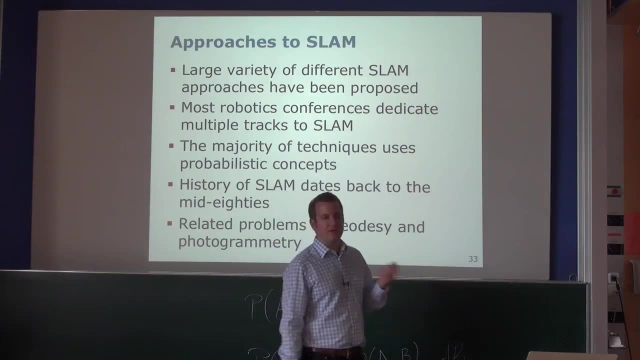 So there's a large number of approaches out there and still a large number of solutions are proposed these days. So if you go to a standard robotics conference, you find multiple tracks actually associated to SLAM problems or SLAM related problems, and there's also a big interest. 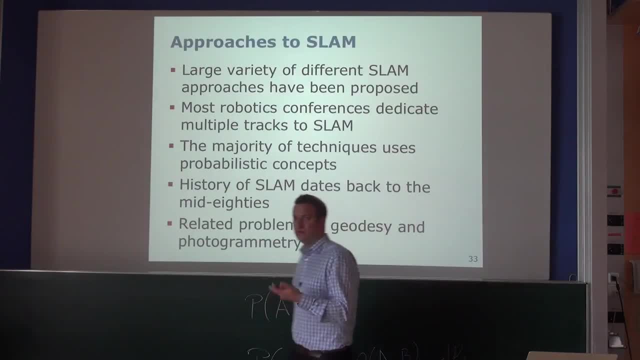 from commercial users these days which try to build robots or robotic devices, devices using robotics technology to model the environment, to estimate where the device actually is. Most of these approaches use probabilistic techniques. there are very, very few which ignore that and they're typically very efficient. 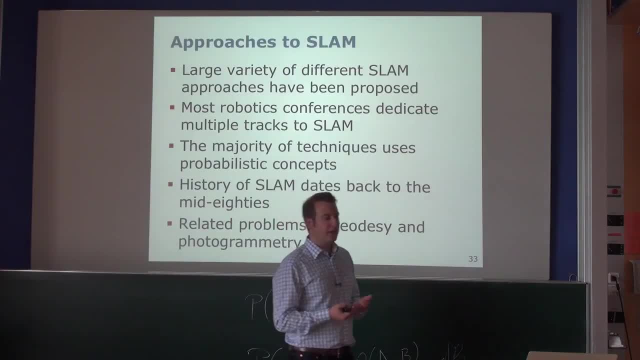 but not that great in performance and therefore there's no way around probabilistic techniques in the context of the SLAM problem these days. The history in SLAM, at least in robotics, goes back to, let's say, the mid-80s, when people started to investigate that. 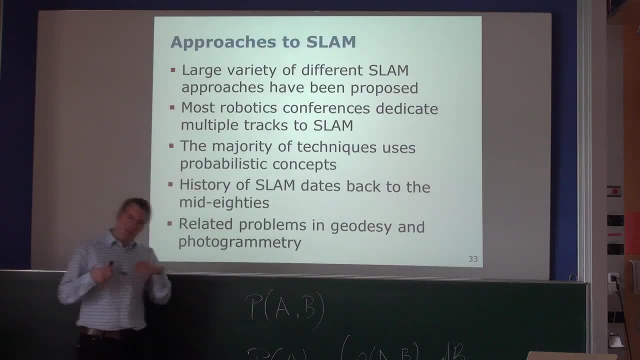 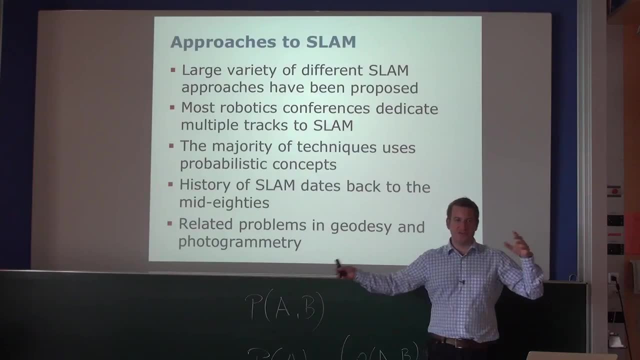 but it should be noted that there are other fields where similar problems have been addressed years ago. So if you look to geodesy- people measuring the Earth, measuring the size of countries where landmarks- they faced very similar problems, whatever the end, the end of the 1800s. 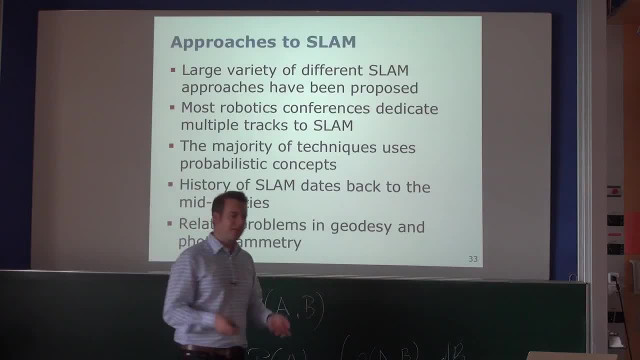 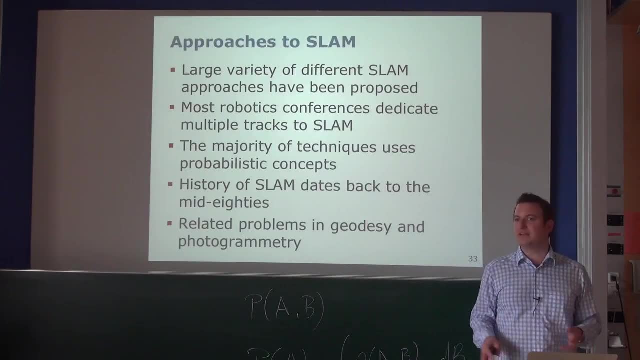 century, something like this. you have very interesting problems which arose years ago and people used methods which are still very related to what we are doing here today. We may have different requirements with robots and, let's say, some problems that they had these days. so computation time. 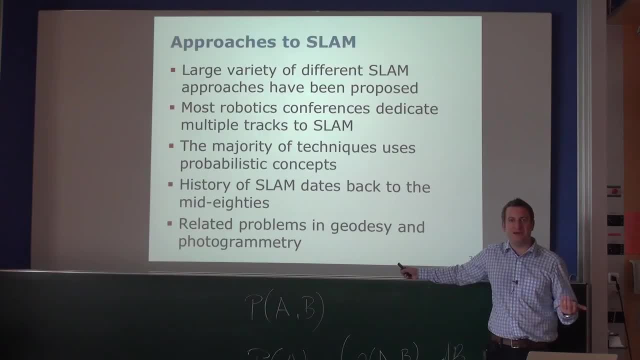 was really an issue 200, 300 years ago. everything had to be done by hand, so that other problems like calculation errors, which we can kind of ignore today and some of the focus was maybe somewhat different, but still they used or addressed very similar problems. 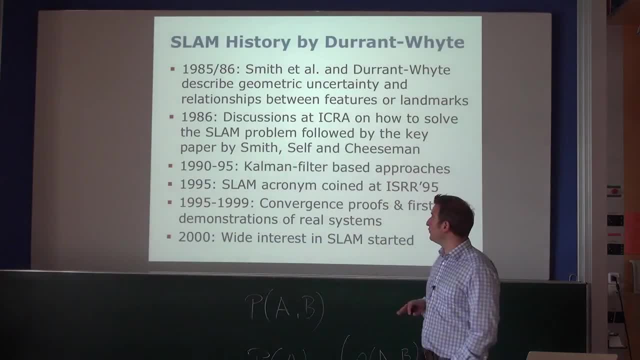 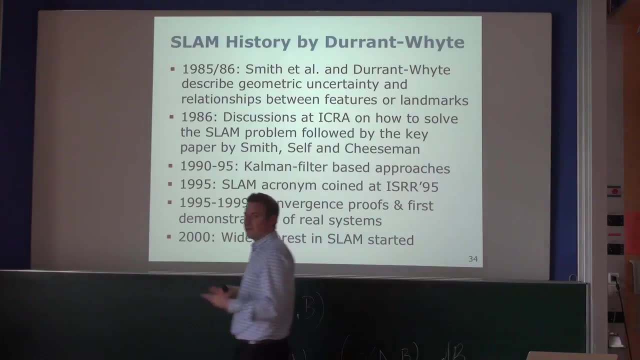 And if we go back at least to SLAM history in robotics, so it started in 85, 86 with, and his team as well as, started to describe or use concepts to describe the uncertainty in geometric relations between observations, between landmarks, and then they had been. 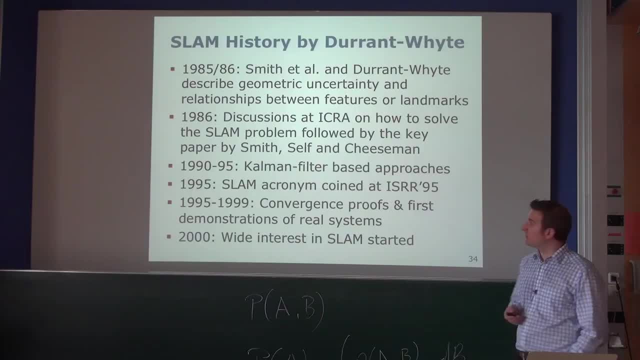 discussed at ICRA, which is the biggest robotics conference, so international conference on robotics and automation, on how to solve the SLAM problem, and then followed by one of the kind of seminal or key papers by Smith, South and Cheeseman In the beginning of the 90s. 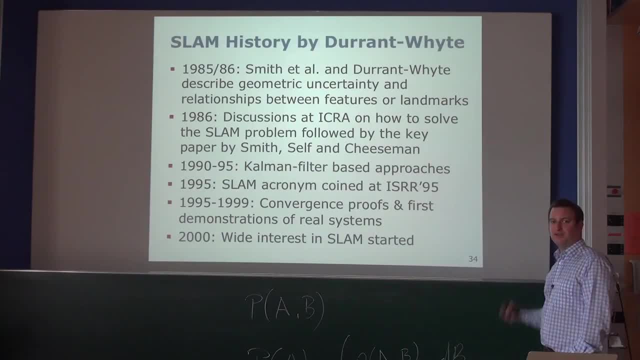 the Kalman filter based approaches became popular. this one estimation technique developed in around 1950. the Kalman filter, which is frequently used in robotics, and then actually the acronym SLAM, was coined at ISRR in a workshop at ISRR in 95. you sometimes find 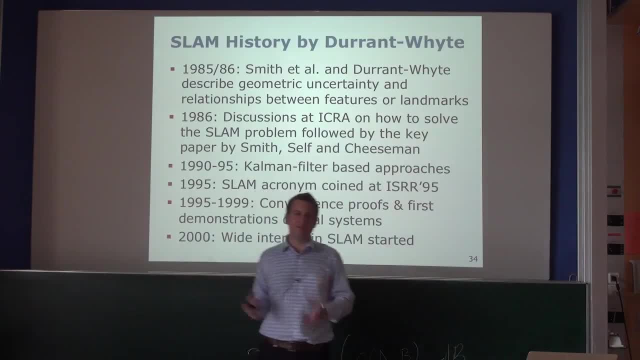 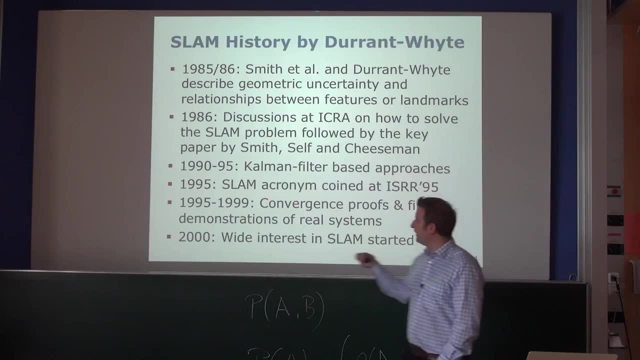 also CML for concurrent mapping and localization, but SLAM simply sounds better than CML and therefore people stick to SLAM. and then there were actually first convergence proofs in the late 90s so that they can show under certain conditions the system will actually converge. 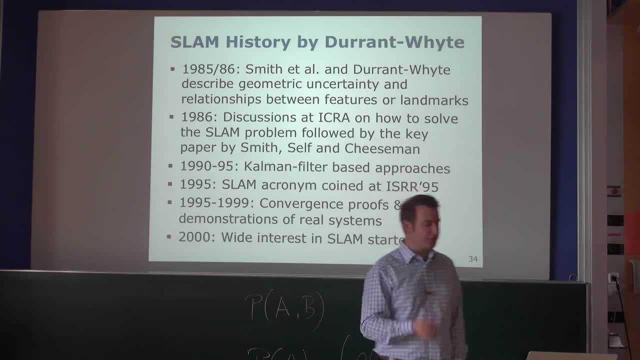 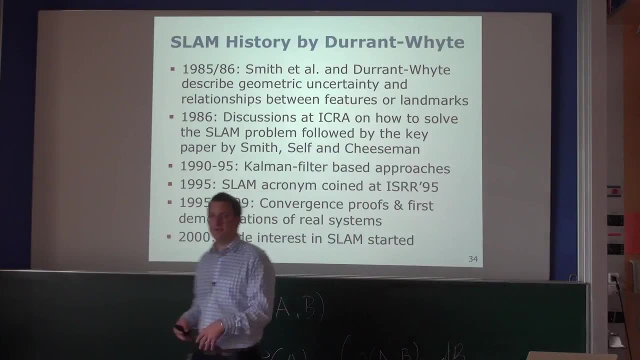 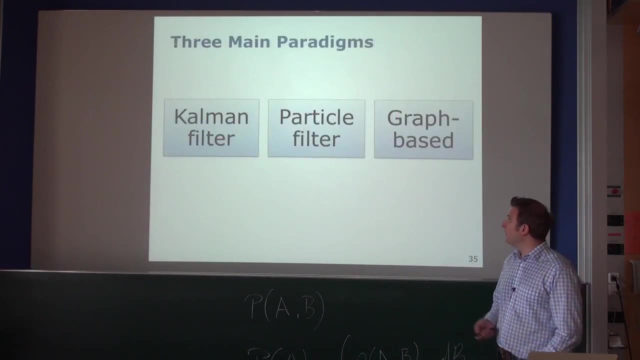 to the right solution under certain assumptions and the first real-world system that we're operating with those techniques and 2000 on it. so even new approaches were published, going beyond Kalman filters, using particle filter based approaches, and also the graph basic approach became more popular. 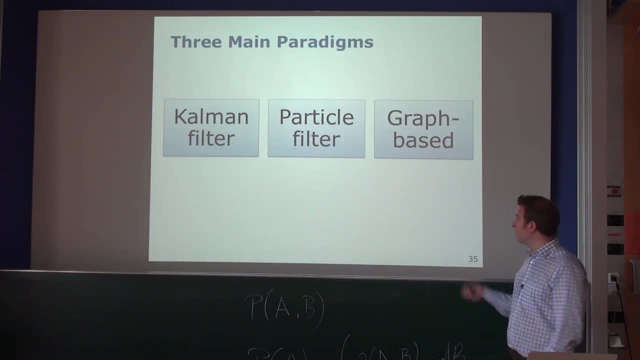 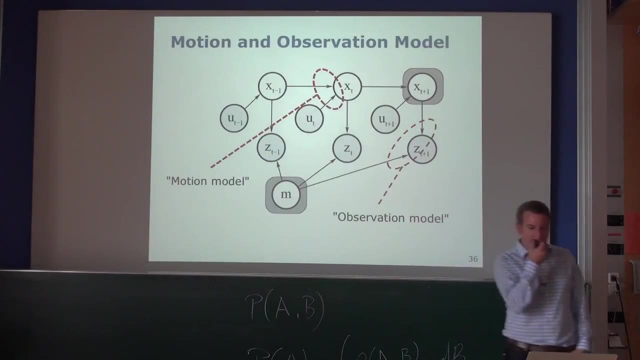 so in this course we will look into the three main paradigms- Kalman filter approaches, particle based approaches and graph based approaches- and in order to do that we can have a look to our graphical model. and all those approaches use two concepts. the first one is: 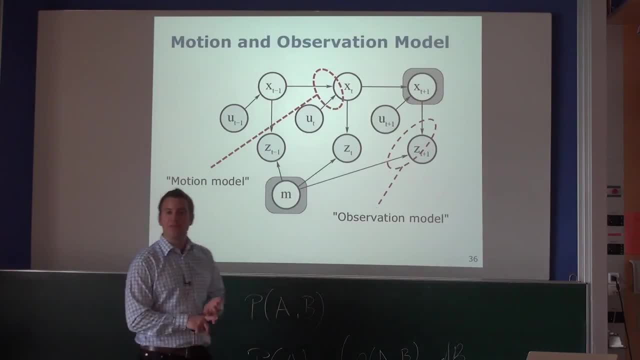 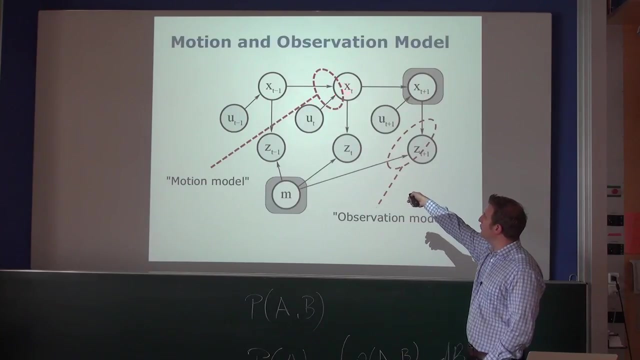 a motion model and the second thing is a so called observation model. the motion model tells me how does the robot move and the observation model is: how should I interpret my observation? and the motion model is actually this part over here in the graphical model. so how do I estimate? 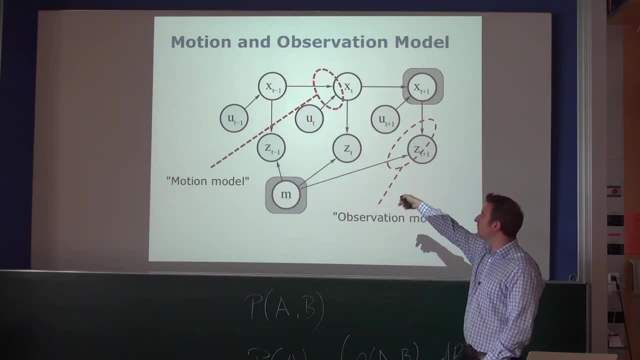 xt given I know xt minus one in ut. so this estimation process over here is what we call the motion model. so how do I get this guy given this one and this one and the observation model? what's the likelihood of an observation, given I know where the robot is. 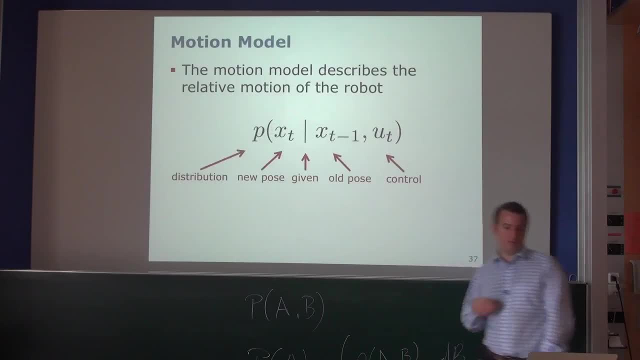 and given I know what the, what the world looks like, so motion model tells me what: the distribution about the new pose of the robot- given I know the old pose, sorry- and the control of the odometry command. so, given I know I was here, given I said 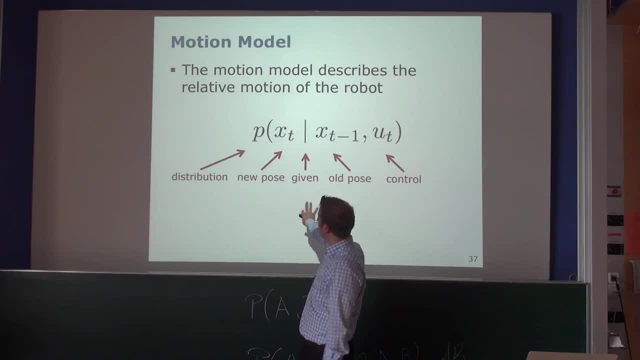 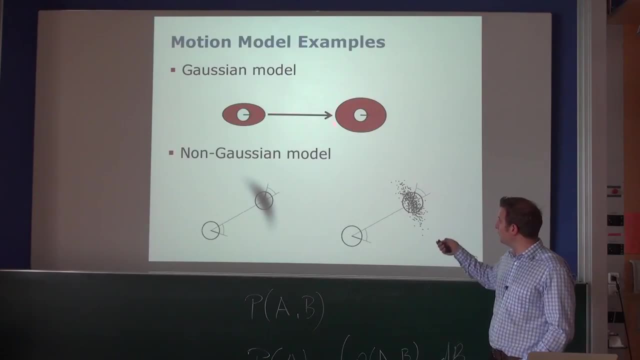 go a meter forward, what the probability distribution of where I end up? that's the motion model. so if you have, this may be your initial distribution. if you move forward- let's say, go a meter forward- you end up maybe with this distribution. if you have a non-Gaussian model, 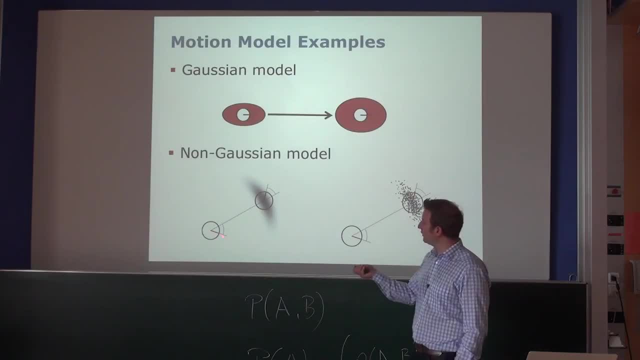 that means you don't have a Gaussian distribution from other means of distribution. the robot starts here, goes here and then this may be what's so called a banana shape distribution, so it looks like kind of a banana and the, the, the angular. so this and this kind of 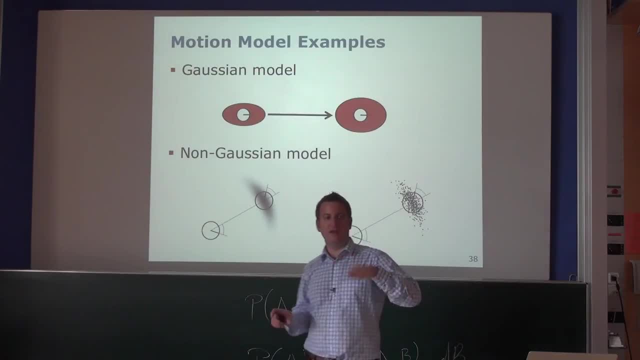 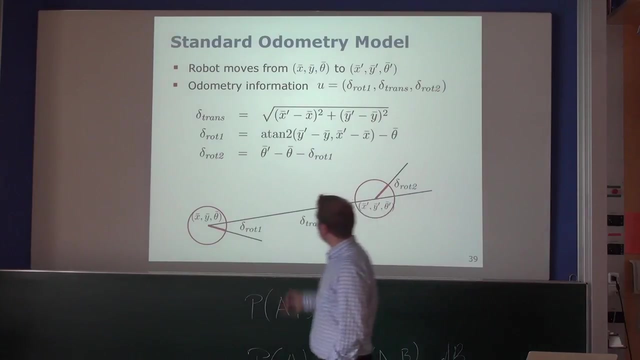 banana shape actually results from the orientation that the robot has and the tendency between the state and the and the angular component, or if you put in a sample based representation, that's also a form of banana shape distribution. we have a standard odometry model that means the robot is 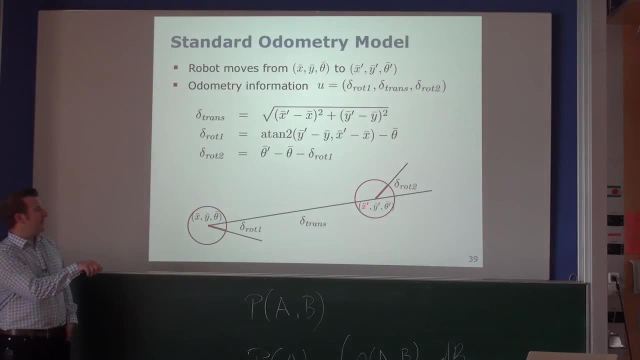 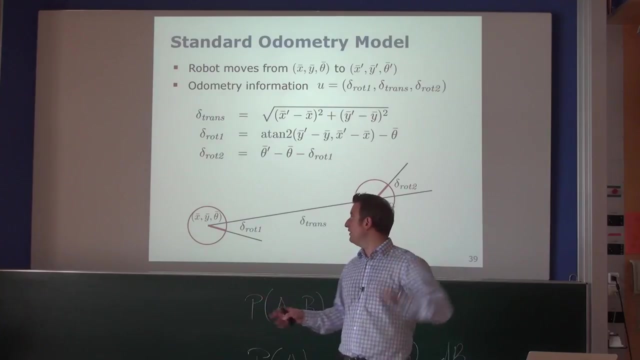 at one point x, y, theta and should end up at x, prime, y, prime, zeta, prime. how can we go there? we can express every motion in the plane by one rotation, a translation and a second rotation. we can describe a transformation between two poses easily. so if this is a current pose, 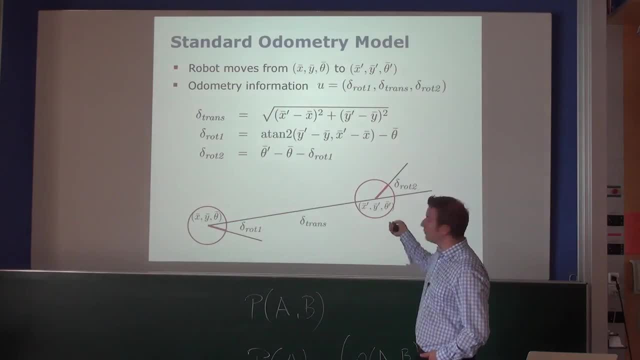 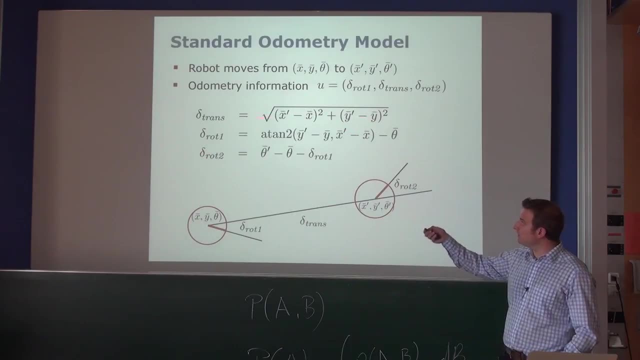 or this is a the heading of the robot: first rotate here, then move straight here and then rotate here. so with three components I can express this and these are the equations you can do that. so that's just kind of the Euclidean distance between those two poses. 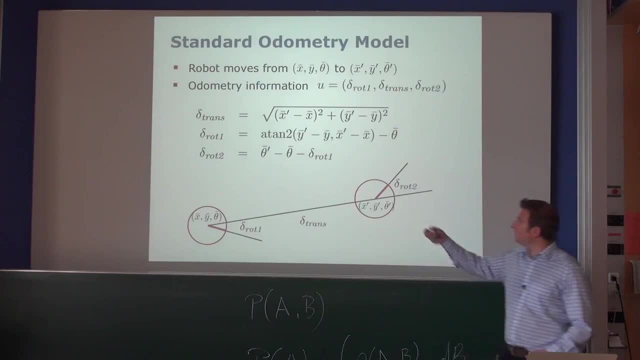 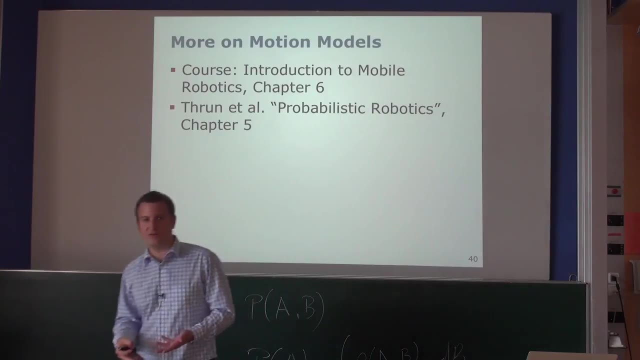 this is the Arcus Tangens for this transformation, and then just a subtraction of the angular components. that was something that we looked into in more detail in the Robotics. I course how to express this, and so there's video recordings from this year. there's chapter number six. 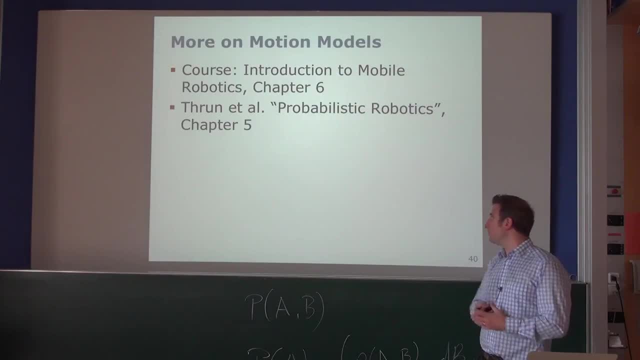 we can look that up again, refresh that. or you look into the Probabilistic Robotics book in chapter five, which tells you something about the motion model. so if you're unaware of that, I recommend you to take the book, read that chapter. it's not that difficult. 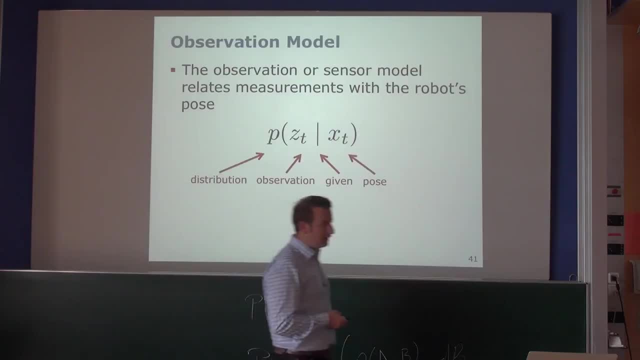 to understand and kind of refresh that we will. I will talk a little bit about that next week as well, give you again a reminder, but it may be good to have read that. the next thing is the observation model. this is kind of the distribution about what I'm going to observe. 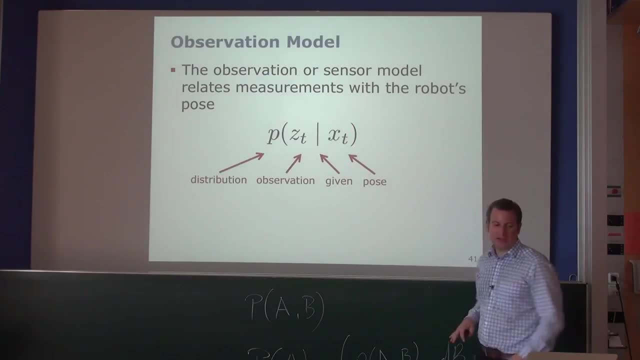 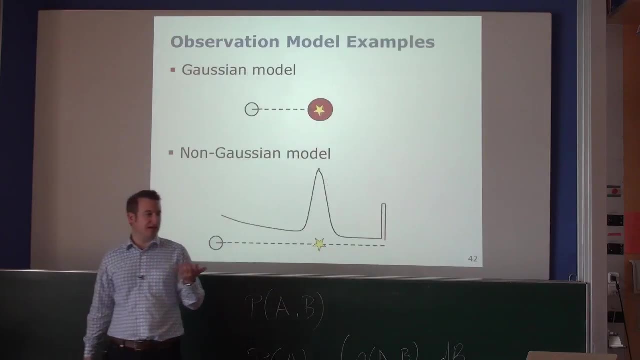 given I know the pose or know the state. also, given all the map which you typically neglect here and which tells you a kind of how do I relay? so what's I'm going to expect to measure, given I know what the world looks like. so, in the Gaussian world, 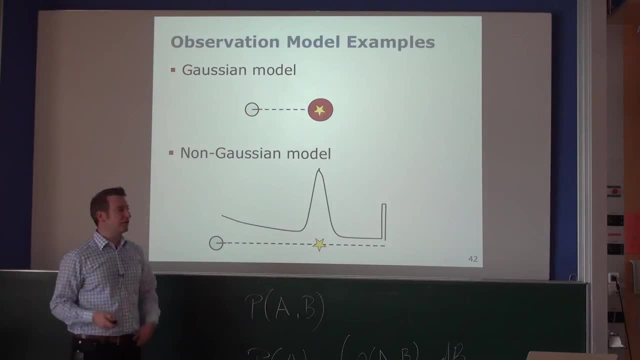 let's say I'm here. I know that the landmark is here, so this is my probability distribution that I'm going to expect. so if I'm standing here, I'm facing the wall. I measure the distance to the wall. I can see the distance a little bit. 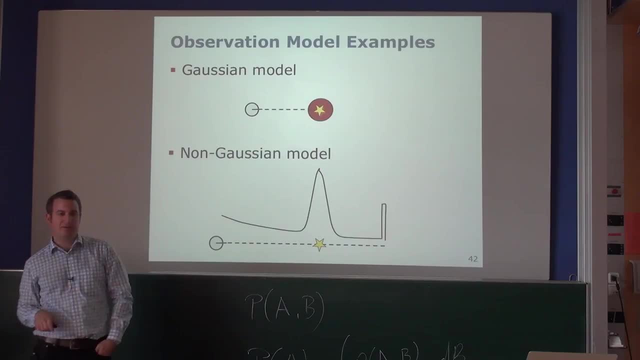 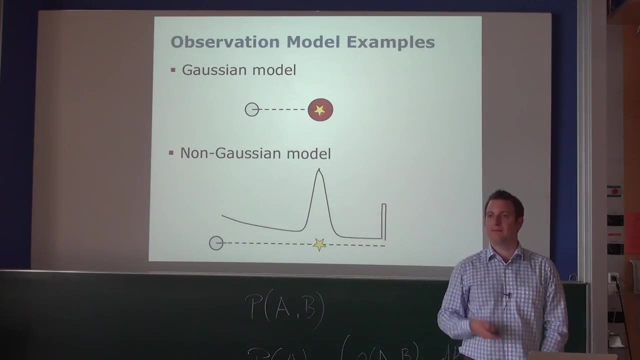 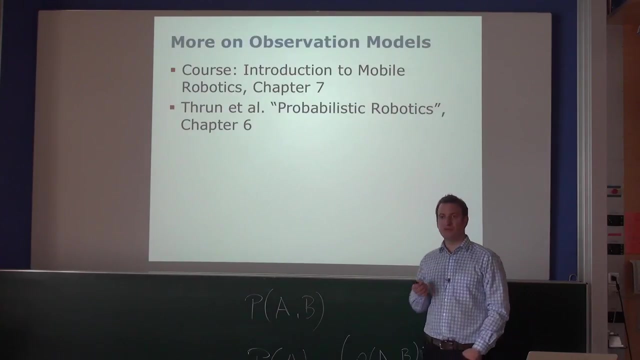 or if I have a non-Gaussian models, you may get other the beginning rather weird looking distribution. so that's for laser range scanner modeling, certain aspects such as dynamics about the scene again. chapter number seven in the robotics course or chapter number six in the probabilistic.